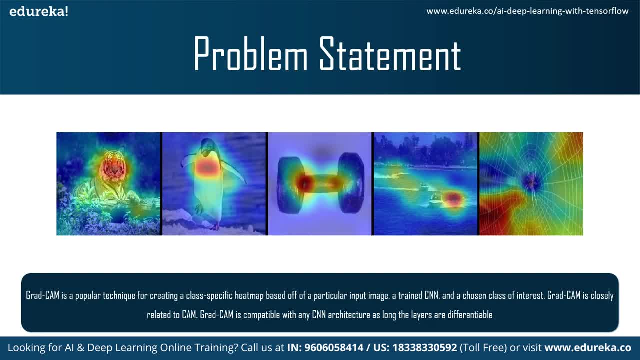 say, gradients that I have, and what this feature map does is, wherever the probability or the pattern that represents a cat are high, We will use the feature map or the probability value or that is going to be high. So what happens? what we're going to do now is we'll 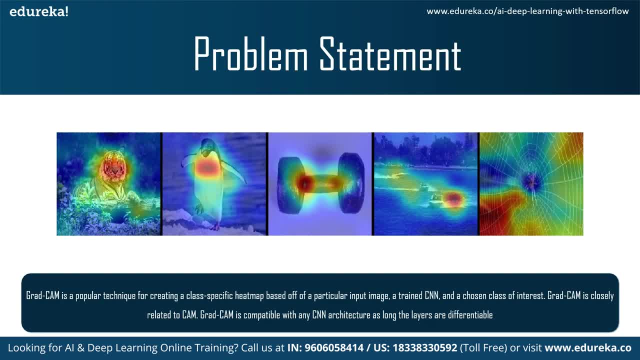 just change the color. Let me take some red color. wherever the feature that represents cat is that that region would be red in color and rest of the region, you know, as it moves away from the features of cat, would become cold. That is somewhere something, let's say, blue over here. So this is what we're going to. 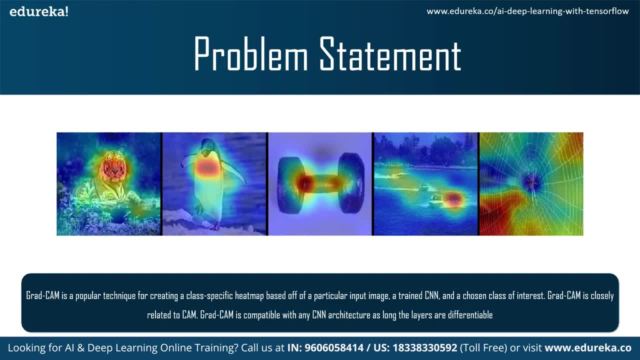 do here? First off, we'll take a couple of data set and we'll try to train it, and then our, as the main agenda says, we are trying to visualize the gradients. Usually, people say that deep learning models are black box model and this is basically we are trying. 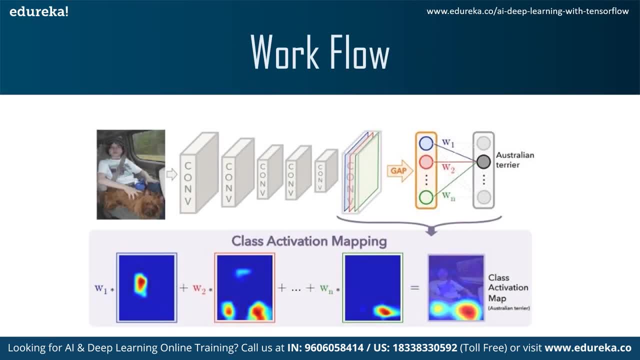 to interpret our deep learning model over here. So, moving ahead, let me now quickly walk you through workflow here. So what we're going to do. first off, we're going to import a data. have already loaded my data to my OneDrive or a Dropbox, and once we load our data, we're. 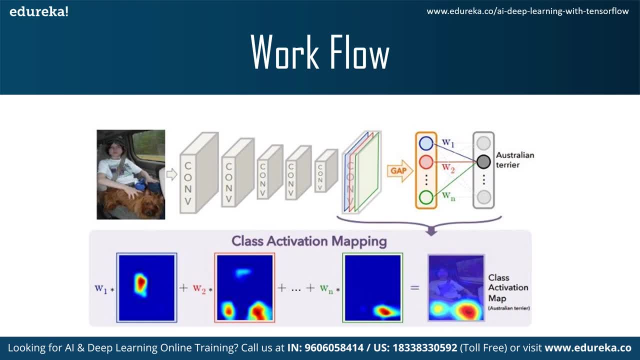 going to segregate them. I'm into cat and dog, just so that I can use data generators, and once I train my model, I won't be creating my own model here. Instead, What we'll do is we'll use some pre-trained model and let's take something like inception model or VGG 19, and finally we'll have we. 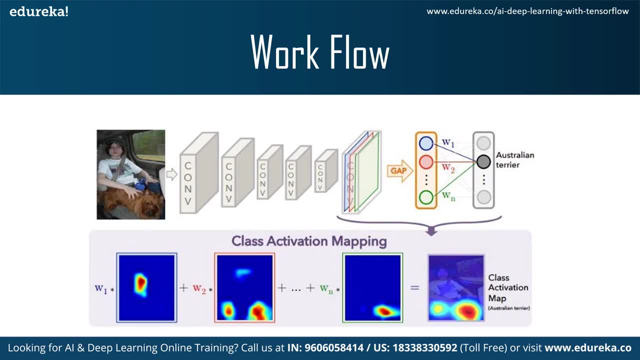 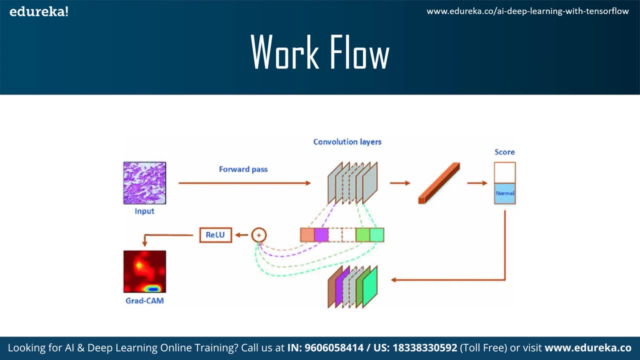 have trained a model, and then we'll try to test this up, like how well our model is working. and then the next stage, what we're going to do is we're going to use a grad cam method to predict or to get a feature map, and this would be in the form of a heat map. and finally, 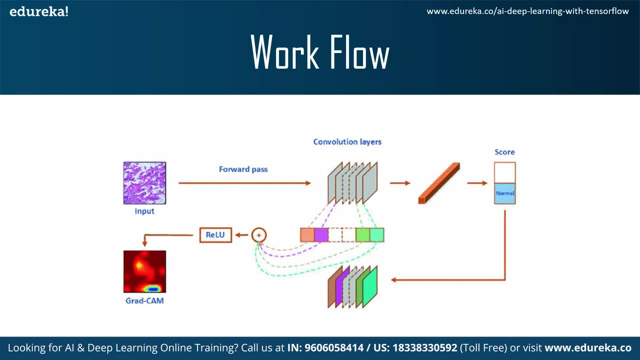 in the last stage. what we'll do is we'll take our original image and then we will use this and we will paste or will reimburse the heat map on top of this, So in this way, we can see where exactly are, or which region is, the pattern that it recognizes. 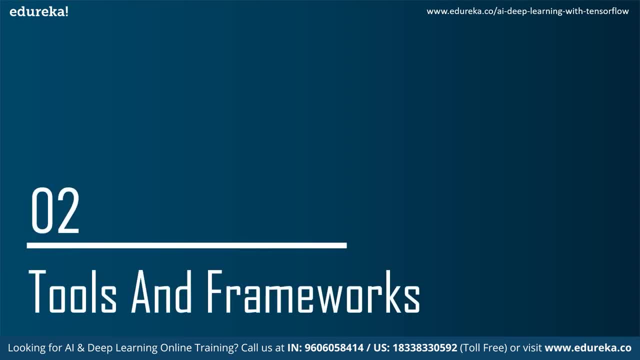 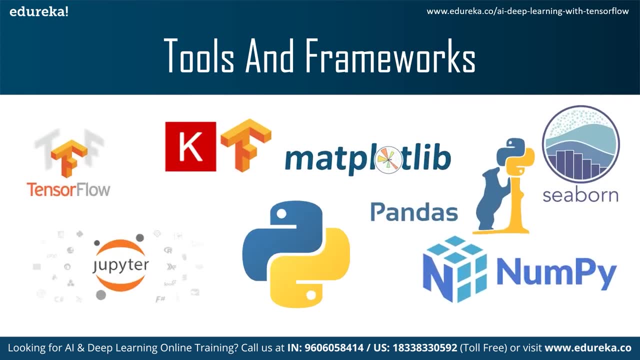 So let me now quickly move ahead and talk about the various tools and frameworks that we are going to use. So, as this is a deep learning model and it requires huge amount of compute power, I'm going to use Google collab, as it gives me a free GPU service. 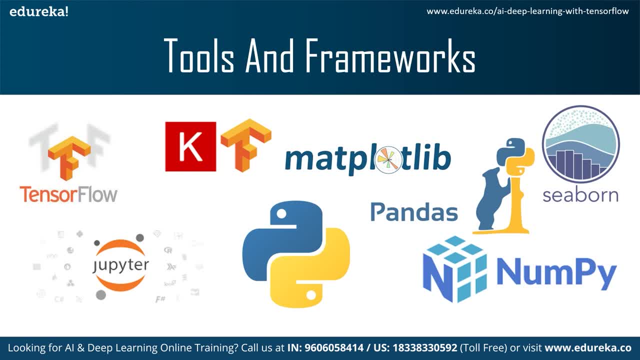 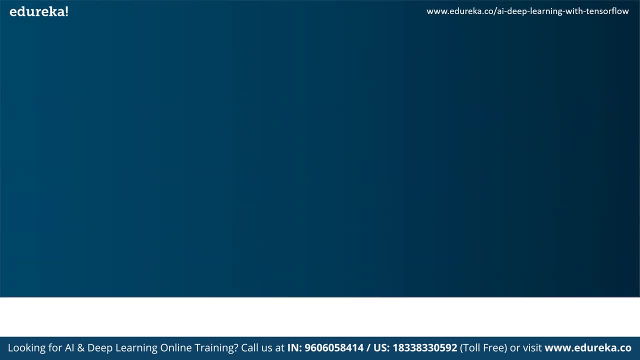 and coming down to the various frameworks that we're going to have. first off, You're going to use TensorFlow, and apart from that there's some generic ones. There's something like a numpy and matplotlib, all at that. So let us know quickly. move to our code editor. 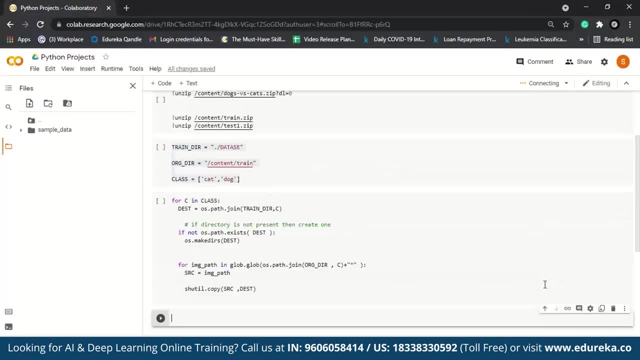 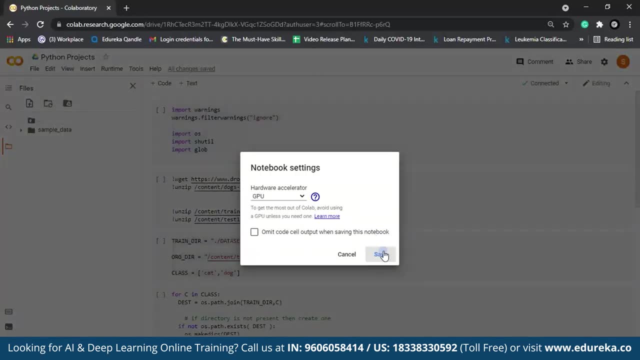 and see how we can implement this interesting project. As you can see, we have come to a code editor here. Let me change our runtime. Usually it's in none, So we'll change this to a GPU one and we'll save this. So now what we're going to do is, as you can see, I've already imported couple of lines of code. 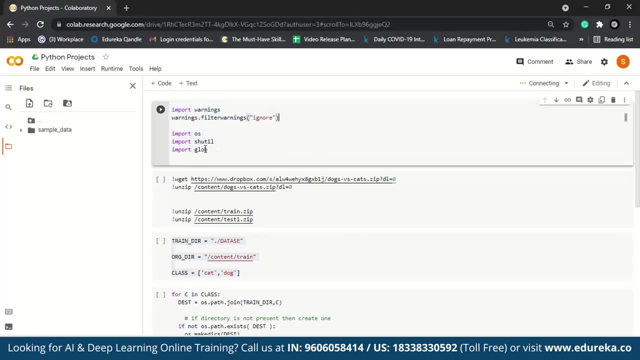 So, first off, I'm going to ignore the warning, So this is what I'm going to do here. And then these are the basic modules usually used for, you know, handling the file. So OS with OS, we can deal with path. shuttle, basically, is used to copy the file from one folder to the other. 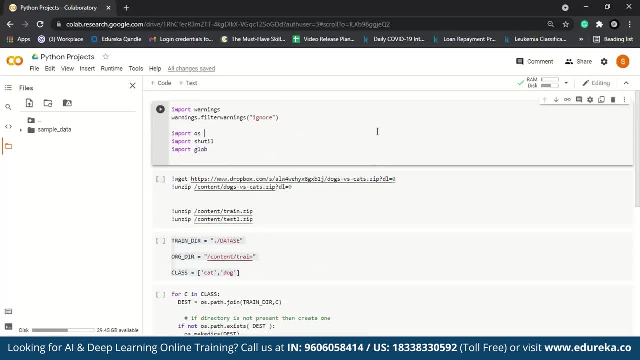 and glob over here is. we usually use glob for pattern matching. Let me quickly execute this up and we'll go ahead and this is where I have uploaded my data set in this particular Dropbox And once I execute this, you will have a zip file and we'll use this part to unzip our files. 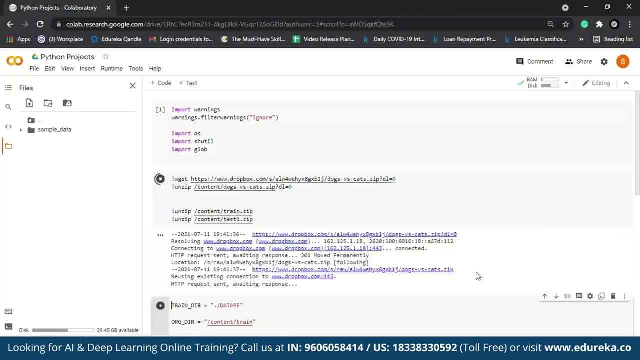 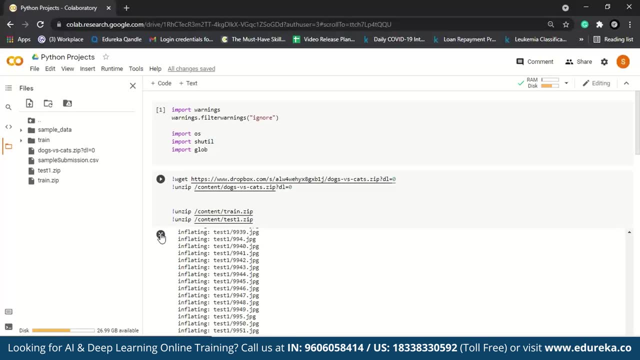 So let me execute this as well. This will take a moment or two, So let's wait for some time. As you can see here, we have successfully imported our data, So now you can see here We have this train folder, and let me give a quick refresh. 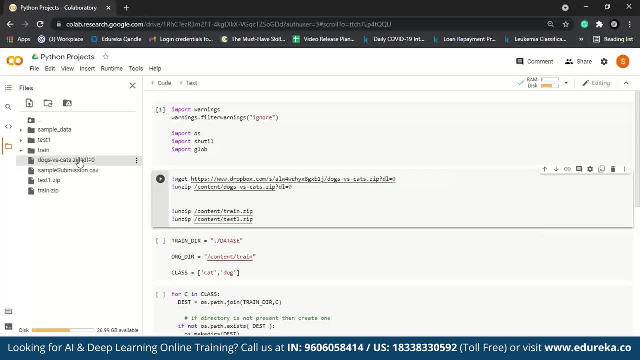 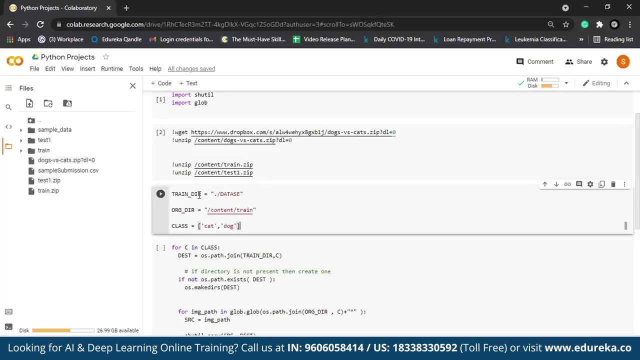 So this is our test folder and train folder, and this train folder should have the cat and dog folders. as this is a pretty huge file, This is going to take quite some time, So what we're going to do now is I just create this variable called a strain directory. 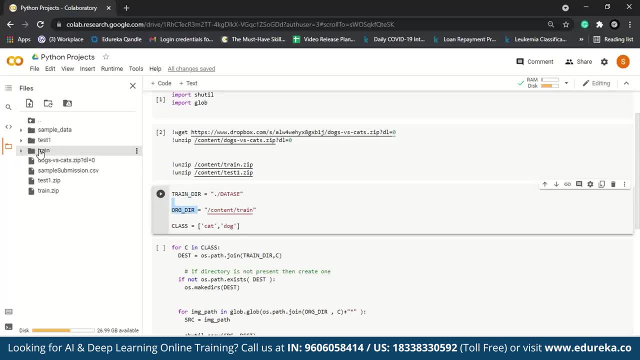 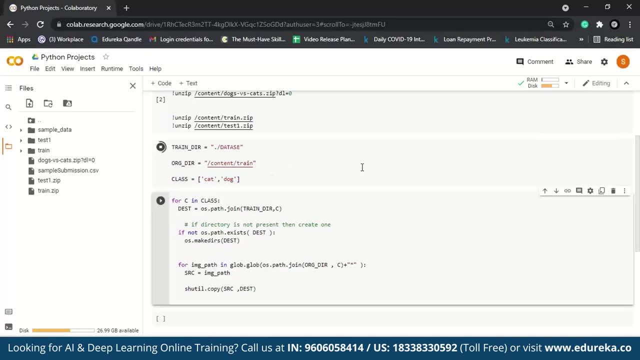 and then we have this original directory. all our images are present, as I mentioned, in this train folder. and then we have the classes dog and cat. So for here what I'm going to do. first, let me execute this and move down to our next block. 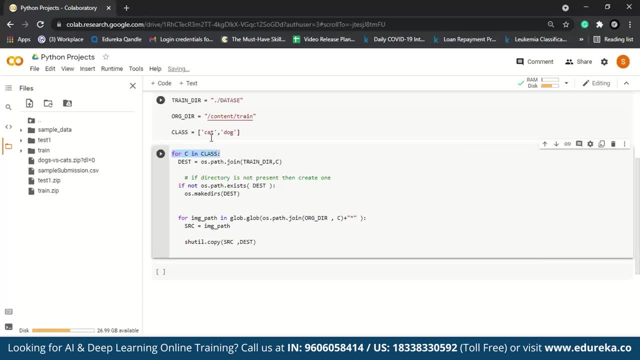 What we're going to do over here is for seeing classes, that is, the classes here can be cat or dog, and we are going to create just a path. So this is where we are going to use OS. Let me zoom in over here for you guys. 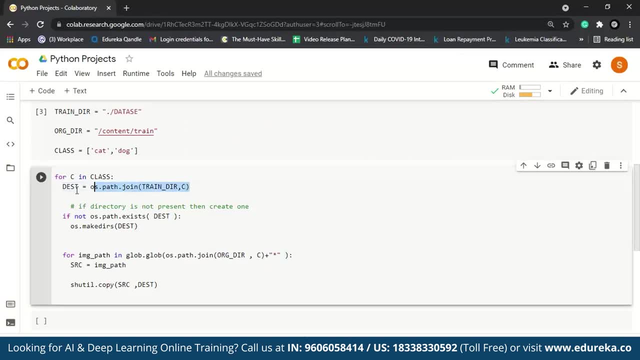 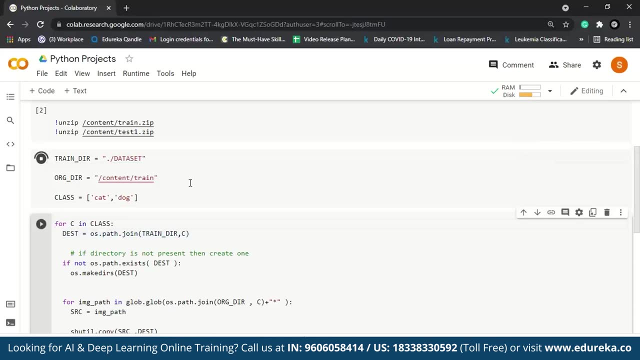 and let me minimize this. So, as you can see, I'm going to create this destination path, So this would be the extension of this data set. Let me change this to data set. Let's execute this and now. what this would do is data set slash. 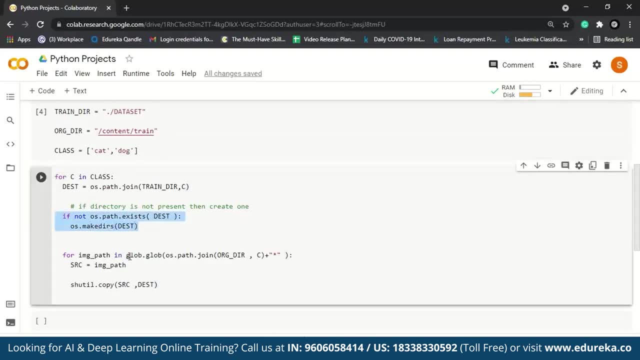 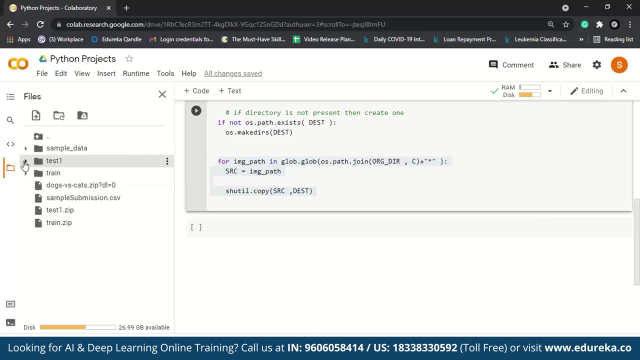 Cat or dog, and then if that particular part doesn't exist, then we have to make that dir and this part over here, basically in based on the pattern. So the name of the file that we have over here, if I can show you here, starts with either cat or dog. 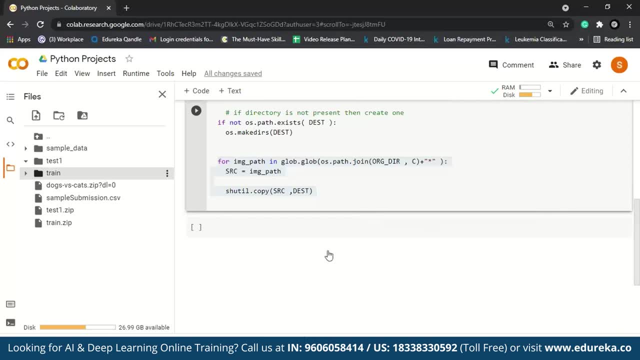 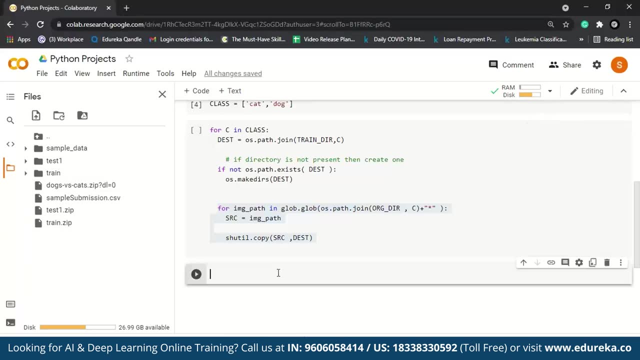 and then we have a serial number, So let's try to look into that at once. So, as there are a huge amount of images, so we are unable to see this. So if you want to see that, so what I can do is OS dot this dir. 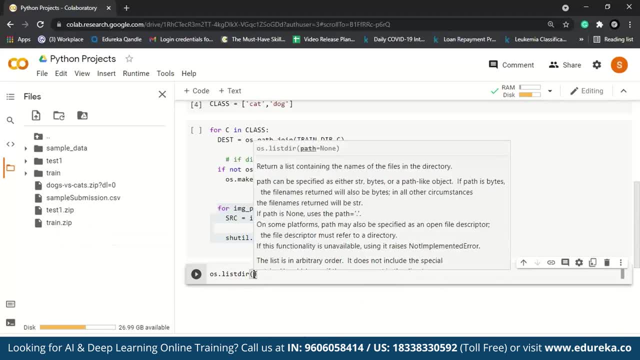 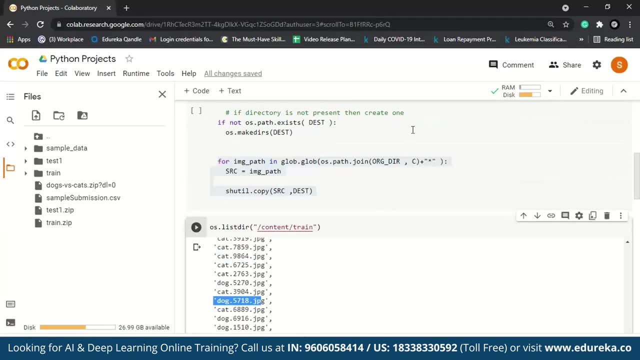 and let me just copy this path. So copy path and add it over here and let me execute this. So, as you can see, we have various cats and dog images and now, if I have to come down here and manually do this work without glob, 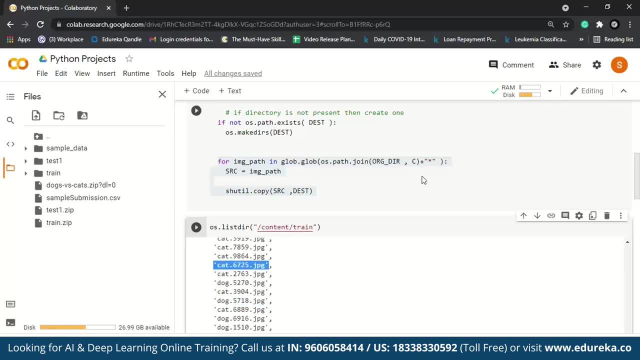 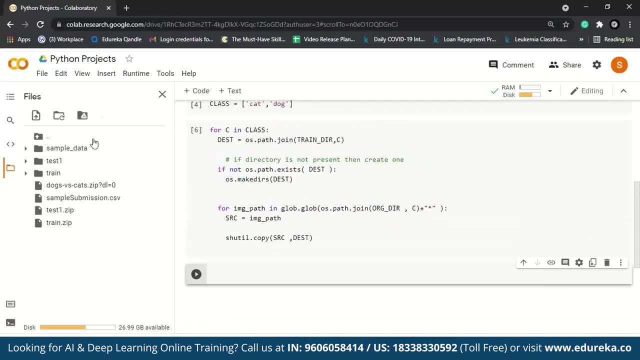 it's obviously going to take a lot of time for me, So this is what I'm going to do here, So let me execute this part of here: shift enter. This is obviously take quite a time and, yeah, it's done, So let me refresh this. we should have this new folder. 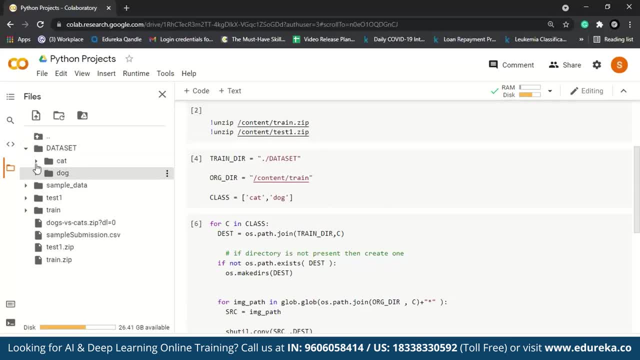 that we have created data set and within this data set I should have cat and dog, and this folder will have images only of a cat and this will have images only of a dog. Now that we have a data set ready, We can use data generator. 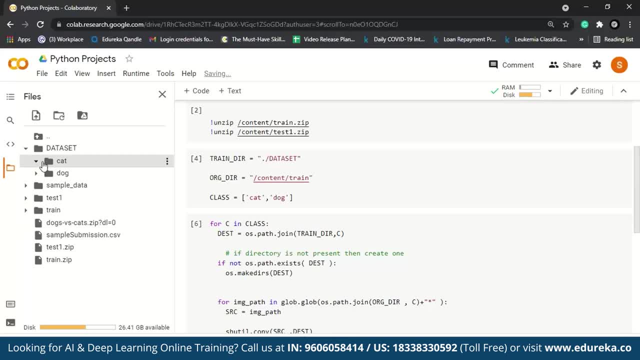 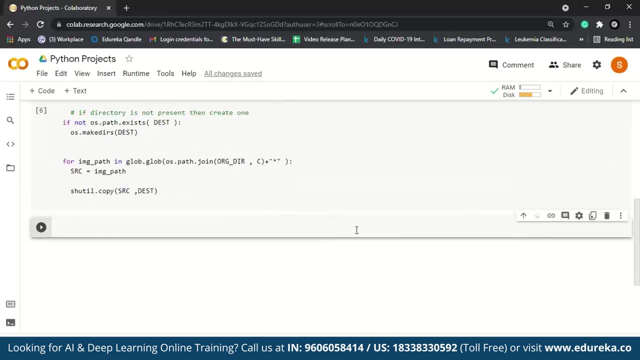 and we can easily, you know, pre-process our data and also add that to our model. So now what we'll do here? we will try to first build a model and then we'll pass our image to pre-process it. So let me give a comment. 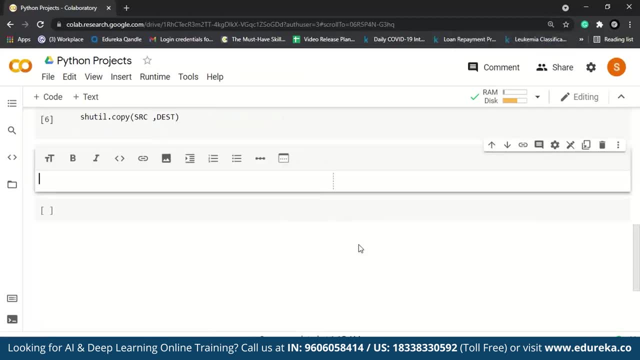 So before that let me zoom in a bit over here and let me give a comment. So let's say building a model. So for this we will be using couple of libraries. Let's say import NumPy as NP and we have import matplotlib as PLT. 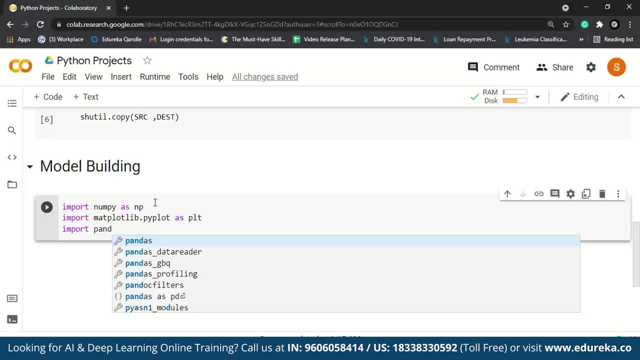 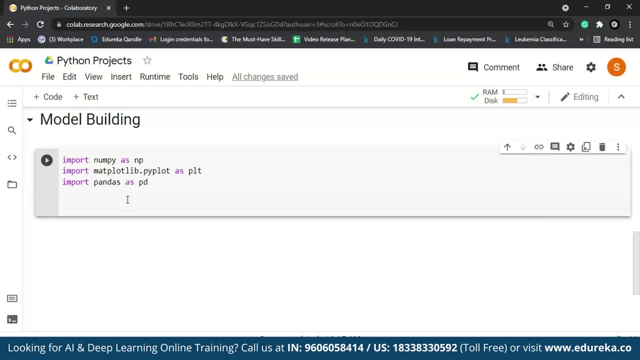 We can also get some import pandas- These are the generic ones- speedy. and now let's import something which is more specific to our model. So, over here, what I'm going to do is from TF, that is, tensorflow. first off, Let's import tensorflow. import tensorflow as Steve. 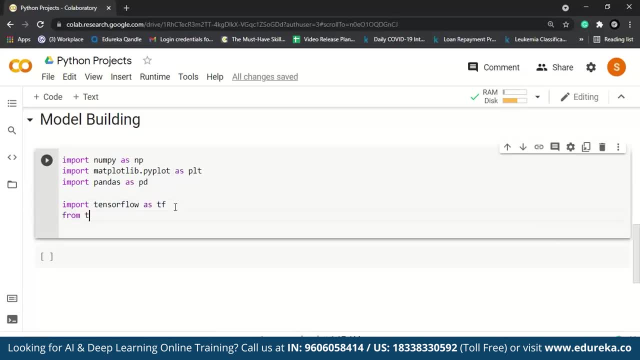 and now what we'll do from tensorflow or that is, TF dot care. There are not layers import as we are going to use just the pre-trained model, So we'll have to use this tool that is going to be dense. dense layer would be for classification. 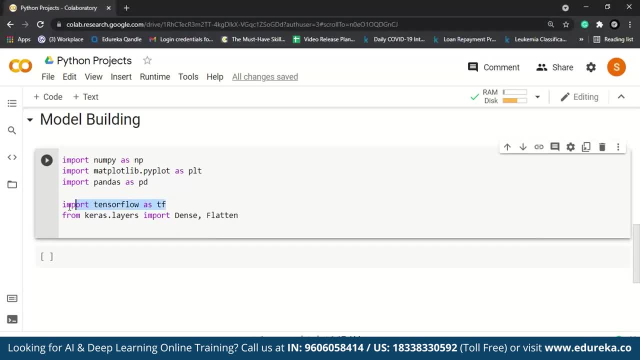 And then we can also use flatten, and as of now we'll just ignore this tensorflow. So, first off, you have got the layers, now we'll import the model. So from Keras dot models import model. This is basically functional API. So we have two options. 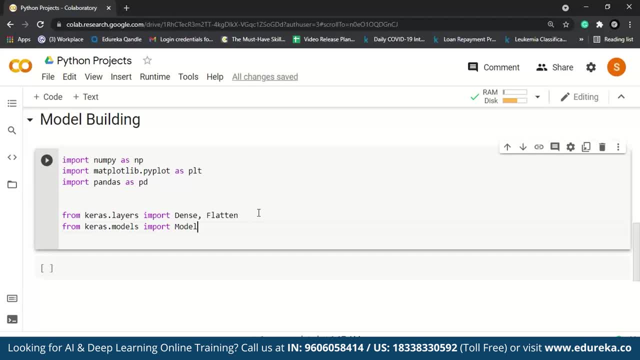 Usually that is sequential or functional API, and to get a functional API we use the model. So, moving on to the next one, let's get a pre-trained model. So we have Keras dot, applications dot. Let's see which one we can take. we have dense net. 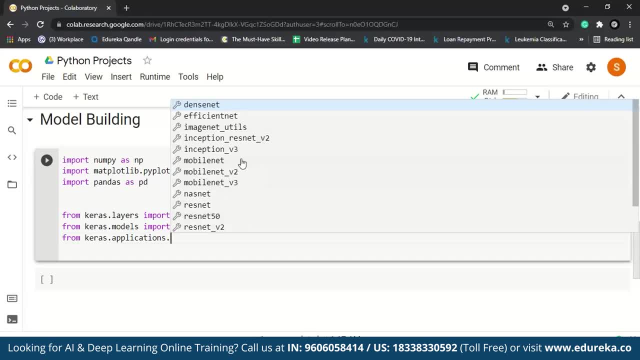 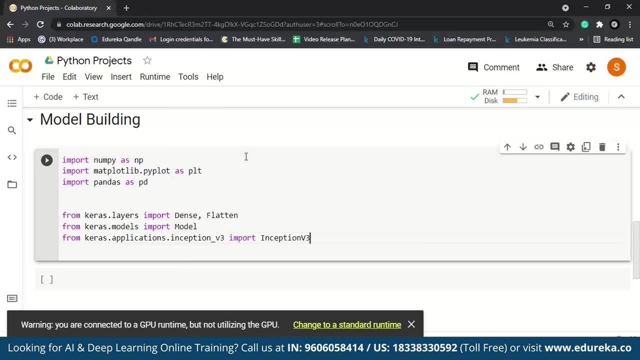 We have inception as net V2.. Let's take something new. So let's take inception V3 and let's import. Let's see what we have over here. So we have inception V3. you have that, so we'll get that up. 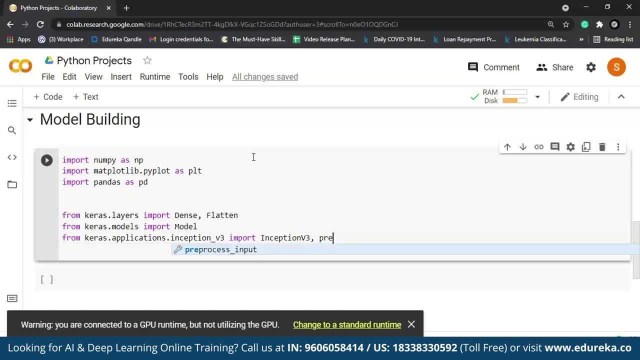 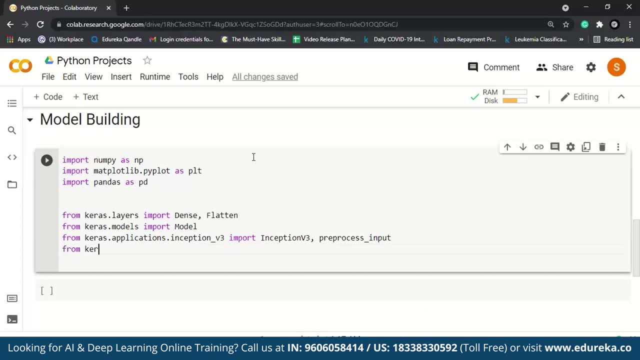 Then we have to, you know, get the pre-processing as well, Right? So pre-process input, and yeah, this should be it. and finally, moving on to getting our image. So, from Keras dot pre-processing dot. image import, Let's see what we have. 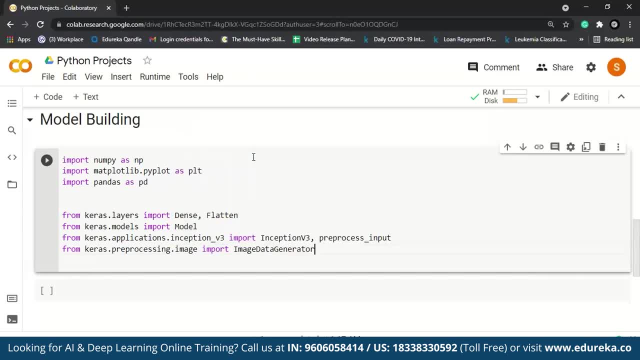 So we have to get our image data generator over here. So this should be it, and just for the generic sake, I'm also going to import Keras. So now we are done. These are the libraries that you'd need for building a model. 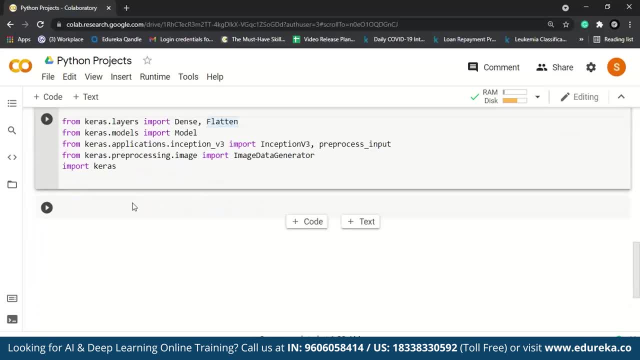 and these are the ones that are true generic. So now that we have executed this, let's more quickly go ahead and build a model. So this thing happens in two stages. Let me quickly show you that, as you all know, first off, we are going to build a base model. 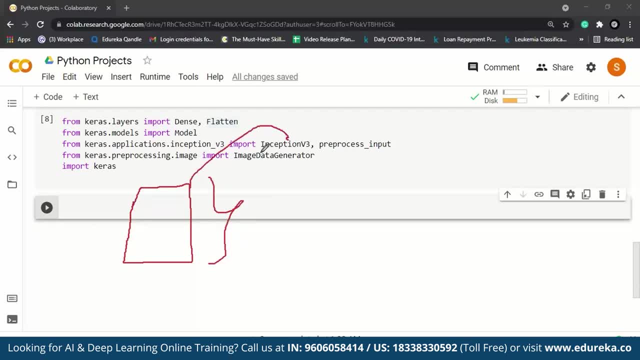 and this base model would be our inception, with whatever outputs I have of inception V3.. I'm going to add this to my flatten layer and then back to our deep neural networks. So- and over here we are not going to train the weights. So for every layer that we are going to see, 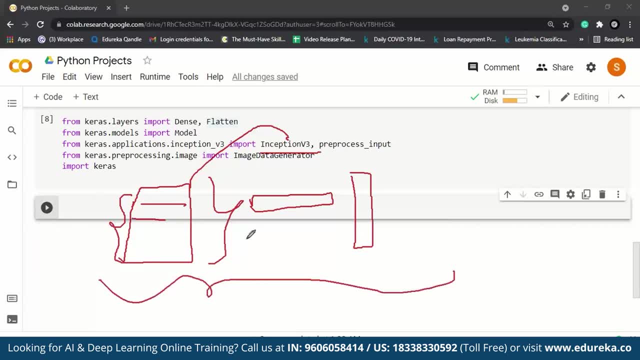 that not trainable is equal to false, and this is how it's going to work. and this model that we have will be a final model Which will give name as model. So let's not quickly do that. So we'll give the base model and what we'll do is we'll call the inception V3.. 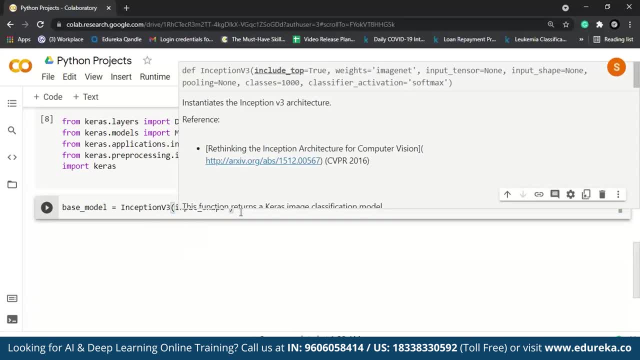 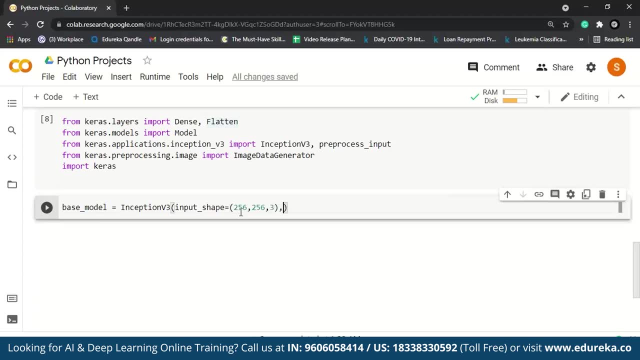 Now we're going to provide the input shape of our image. So input shape, let's say 256 comma, 256 comma, 3, 3, as you all know, it's for the channel, and then we have include top. that is false and this is all there is we have to do to get a model. 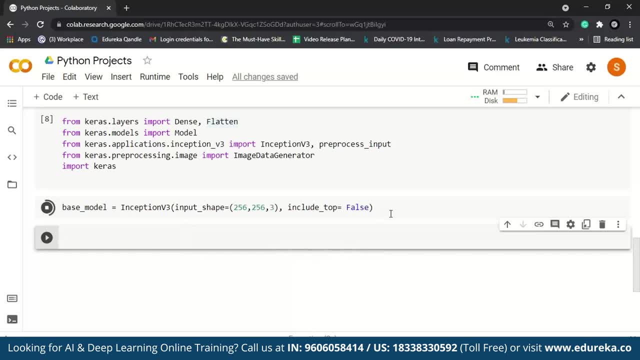 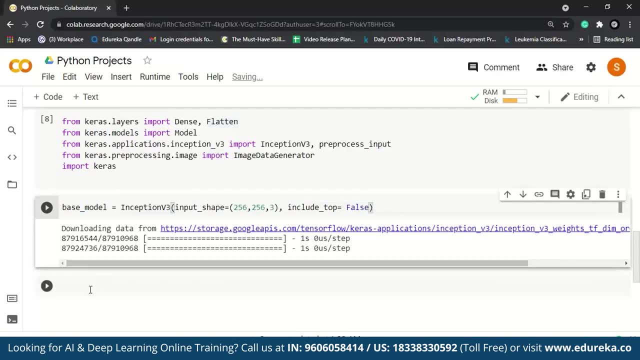 Let me execute this now. This is going to you know. make sure you're connected to the internet, because this is going to download inception V3. once this is done, as I mentioned earlier, we are not going to train any layers over here. So for this, what I'm going to do, for layer in base model, dot layers, 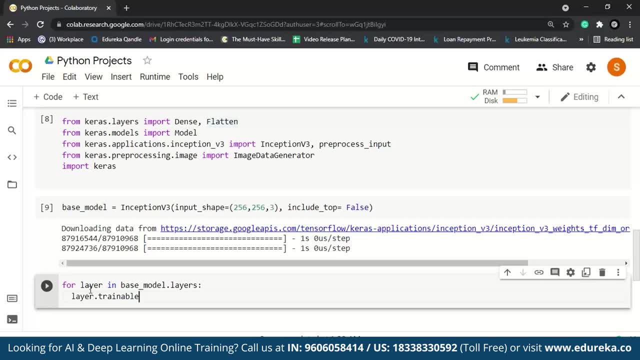 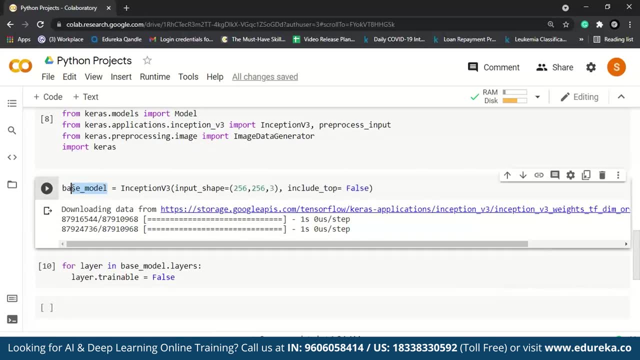 and we layered or trainable would be false. And now we execute this. Yeah, now that we are done, what we're going to do Now, whatever is the output of our base model, we are going to take that and add that to our actual model. 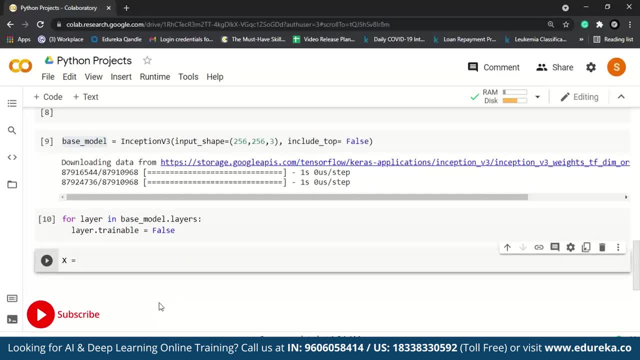 So for that we'll say we are going to use functional API. So let's say, X is one variable and we are going to flatten this and obviously you're supposed to give the input for this. now for the input for this is going to be base model dot output. 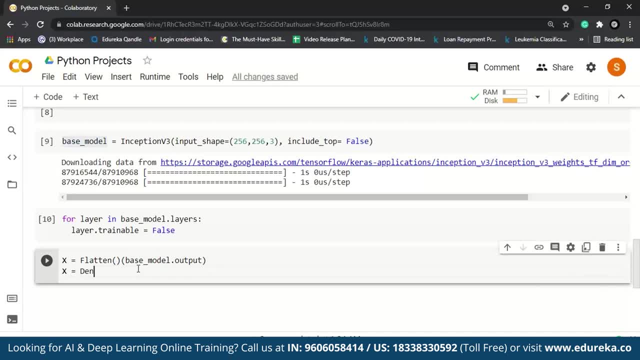 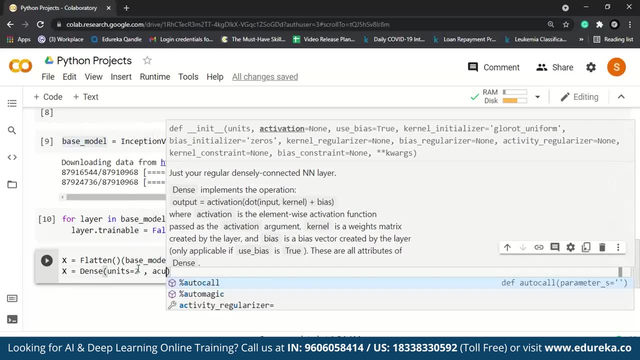 And again we'll have X. so over here We're going to give a dense layer and, as we have number of classes as to, so our units over here will also be to. activation that I'm going to use is going to be sigmoid And the input for this is going to be X. this part is going. 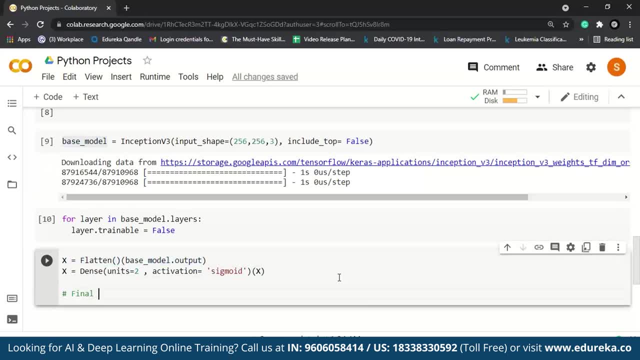 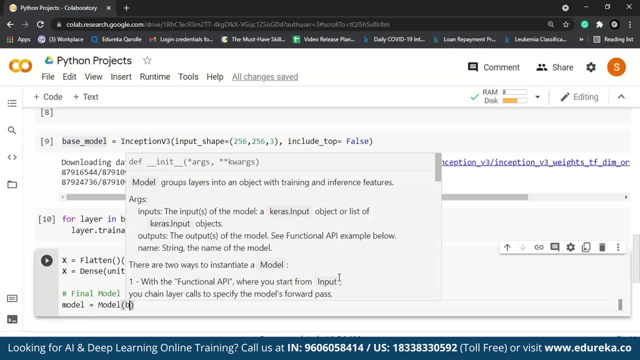 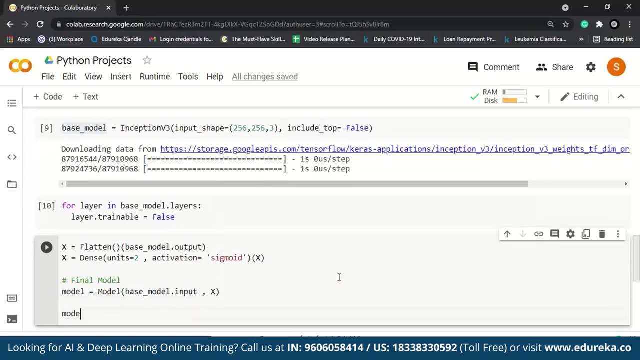 to be the input for this. and finally let's create a model. So we'll give the name here as models and we'll say model and just give the inputs and outputs. So base, model, dot, input, and finally we have our X parameter and now let's try to see model or summary. 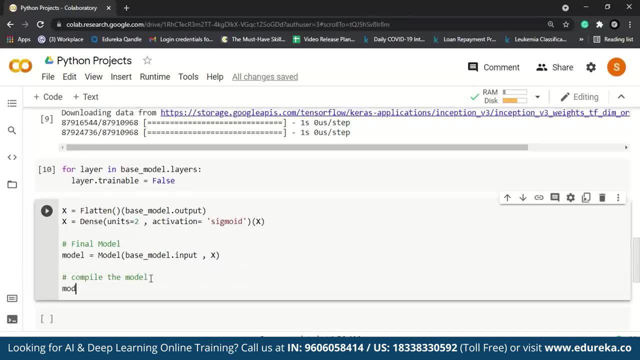 But before that let's compile a model, And here we're going to give couple of parameters. We have optimizer- the optimizer I'm going to use is Adam- And then we have loss. Let's say we're going to use binary cross-interview. 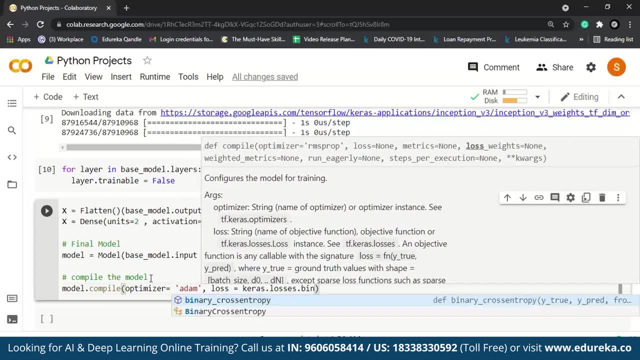 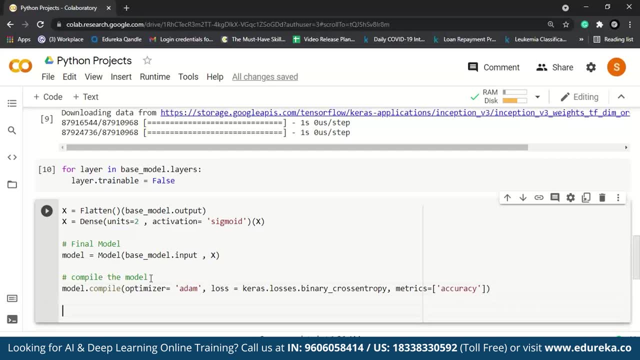 So we have Keras dot losses, but binary cross-interview, and then we also have metrics here and we are going to provide the metrics to be accuracy, And now let's see the summary of this. So, for this model, dot summary and let's execute this. 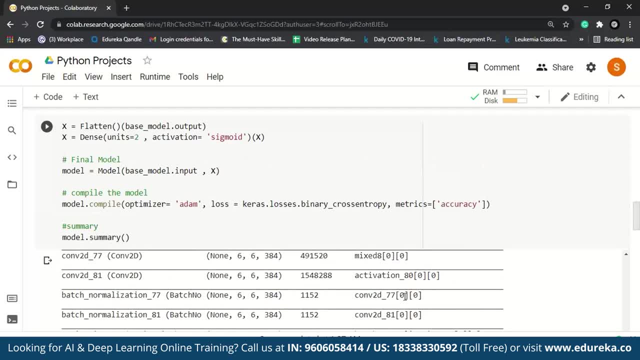 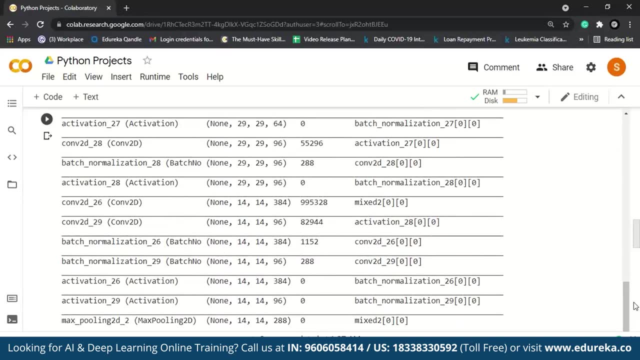 So, as you can see, this is going to be a pretty huge model and although it's not necessary for us to use such a complicated model on such a simple data set, but you know, we are just trying to see what's going to happen, right? 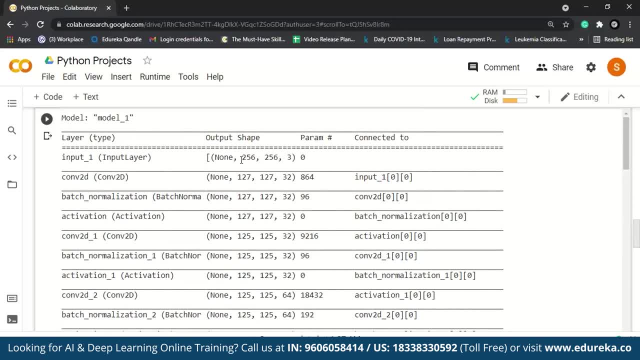 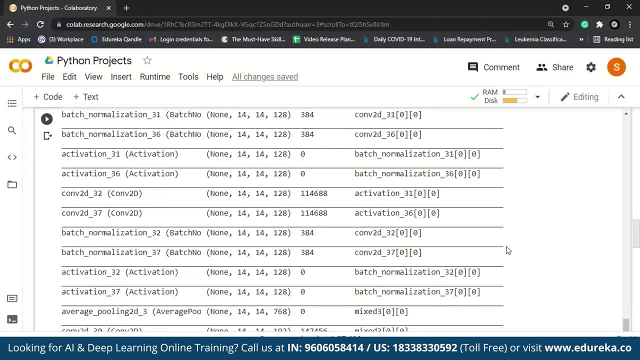 So this is something new that we're trying to do here. So this is the input layer. as you can see, it's 256 comma 256 comma 3 and finally we are going to take the outputs. Let's see how our output over here looks like this definitely. 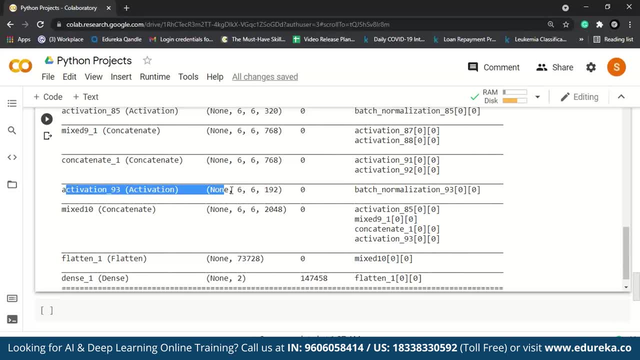 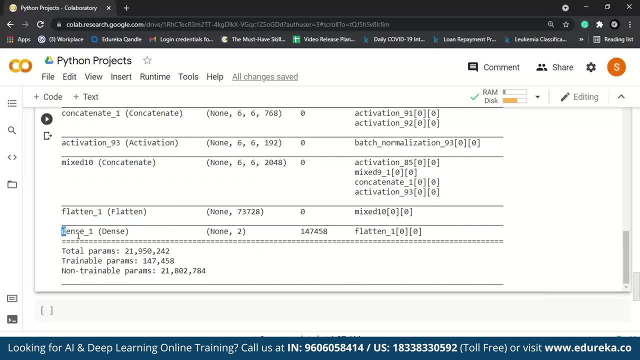 has a huge amount of layers. So, as you can see here, this is our activation function. Then we have mixed 10, concatenate and finally we are trying to add this right, so flatten, and then finally we have dense layer which has two outputs. looks great now. 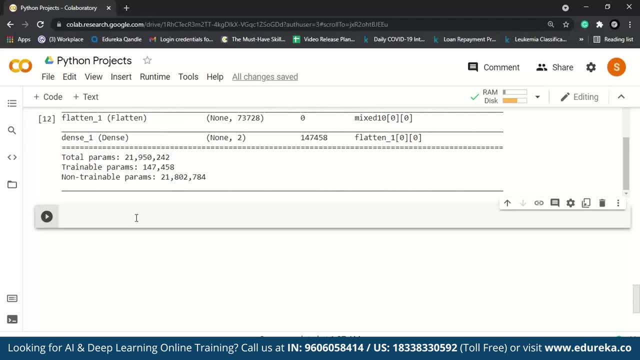 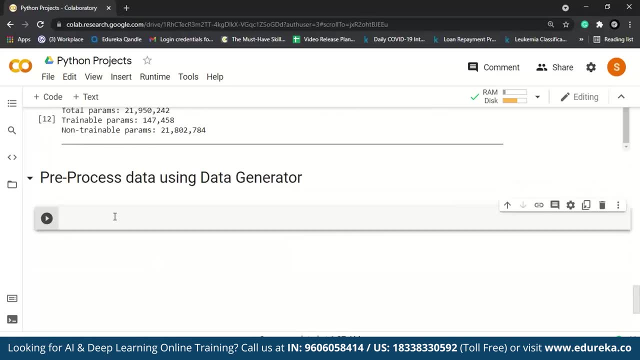 So now what we're going to do In our next stage? We are going to pre-process our image, that is, pre-process our data, using data generators. So we are just going to use training data generator. So let's say, train data gen over here. 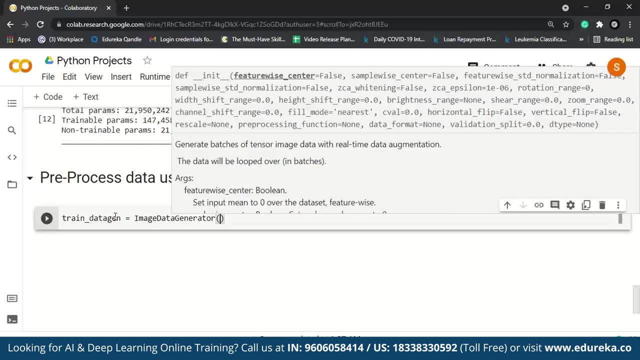 We are going to have image data generator. So couple of things: we can add all of these values here. So let's now start adding all of these values, and the more the number of values are add, It's like I'm adding more number of dimensions. 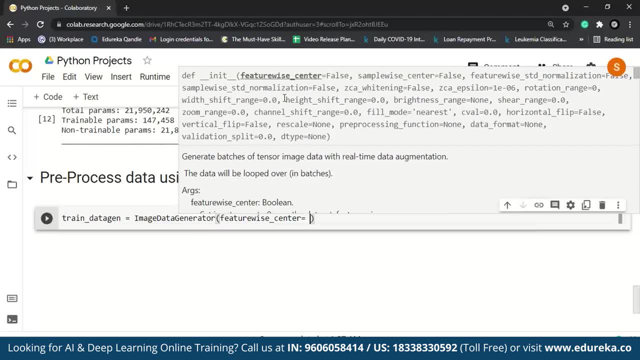 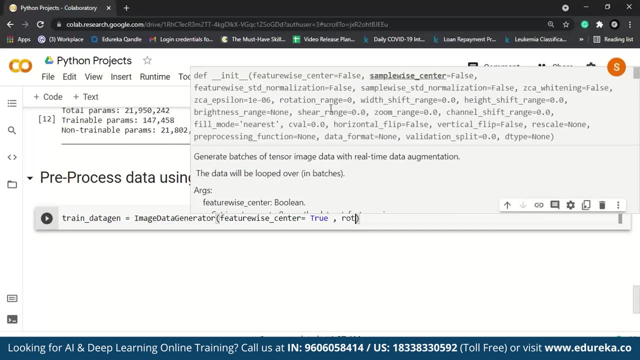 So let's now get started. So let's say feature Center, we can set this to true, and then we have stepwise Center. Let's ignore that. we can add this up: rotation range. This is how you know how much our image is. So let's say 0.5, or let's say 0.4. 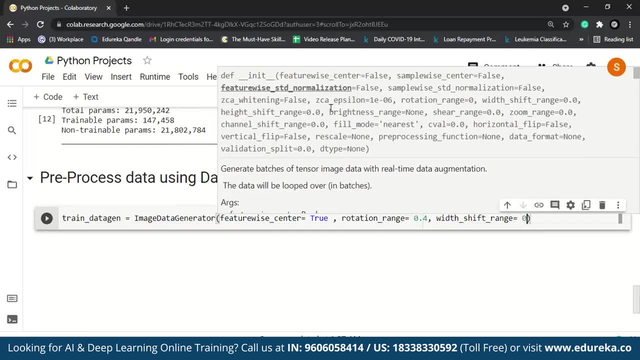 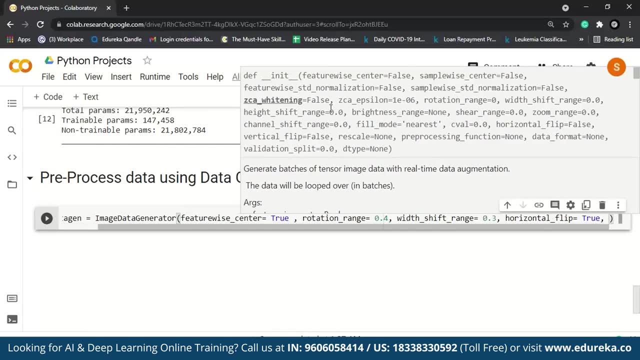 and then we have which shift? let's give this as 0.3.. But then we'll do horizontal flip. Let's say true, and we are also going to add a pre-processing function, which is pretty important. The reason is because, as we're using this inception model, 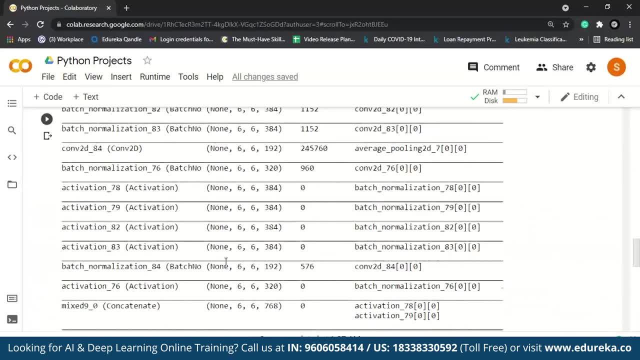 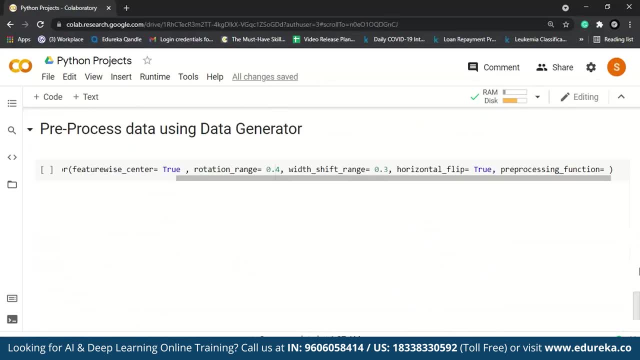 so this model of trained on certain data set. So we are just going to provide that as well And let me quickly see what that's going to be. So that's going to be this part: pre-process input. So let me scroll down for this. 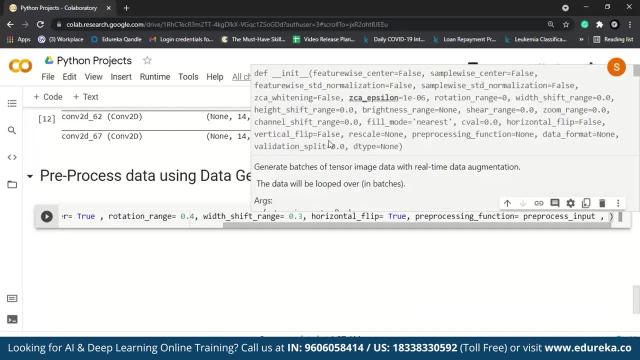 Let's add pre-process input and then let's say vertical flip. It's totally up to you. We don't have to rescale over here. The reason is because, anyways, where you passing this through a pre-processing function? So we don't need to do that. 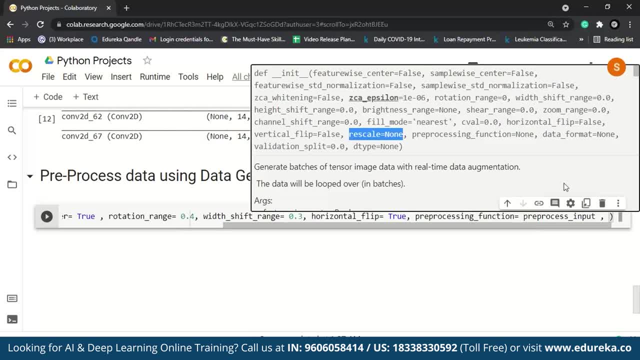 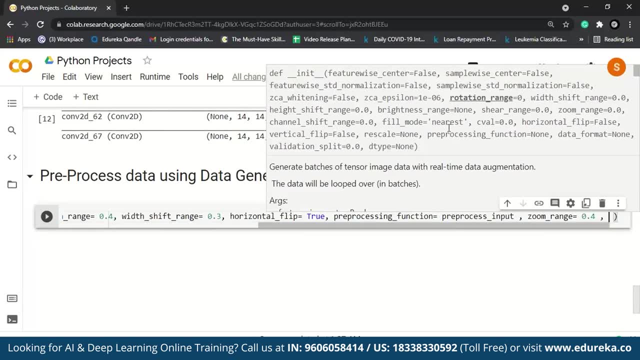 And then let's see something else. We can add this zoom range. Let's say zoom range to be 0.4.. Similarly, we can also add some more values. Let's say something like sheer range 0.4, and I think this should be fine. 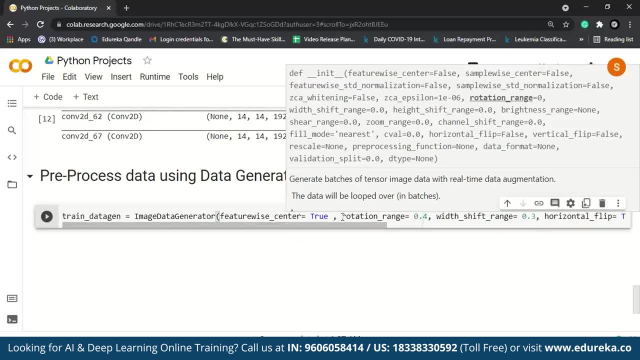 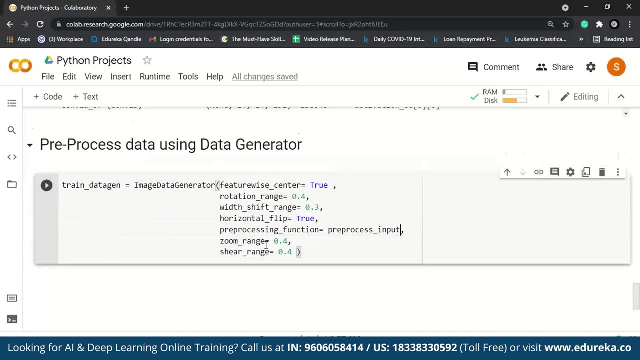 So what I'll do is, just for the simplicity, say let's try to add this one below the other, just so that it looks good, right? So? so we have added this data generator. as you can see, we have added couple of dimensions and will execute this now. 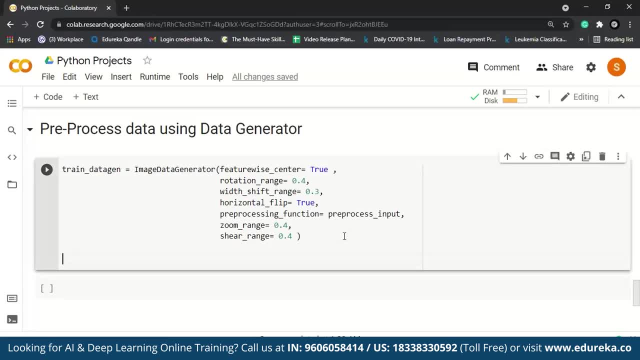 So now, finally, for this, we have one more step, that is, let's say, train data will give this name, and this is going to be trained data gen, with the function flow from directory, and we are just going to pass a directory name. And let's come back here. 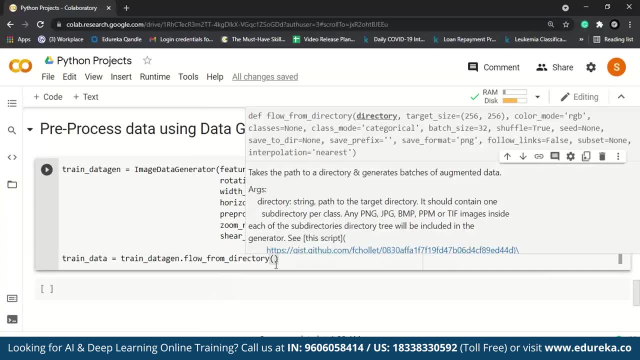 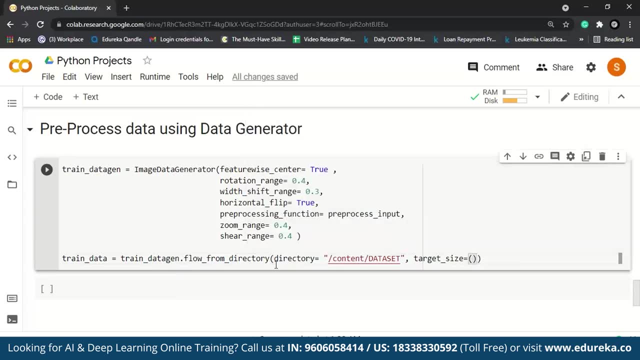 and this is going to be our directory. So we'll copy the path and now we'll give directory name over here. Then obviously we need the target size. So, as I mentioned earlier, it's going to be 256 or 256. this should be similar to what we have provided. 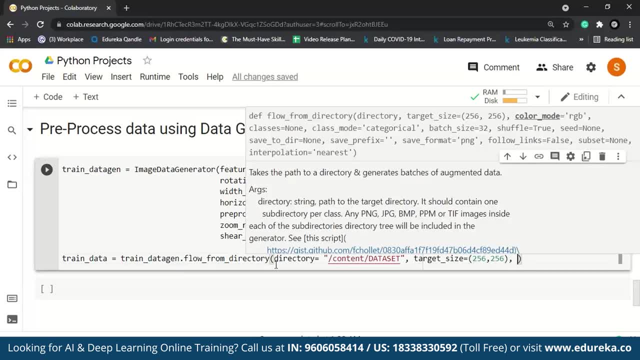 or else your model is through an arrow and then, as is a pretty huge amount of data, We are going to pass some batch size as well. So we let's say batch size to be 36, and let me do the same thing here, Let me put this one below the other. so we are done with this. 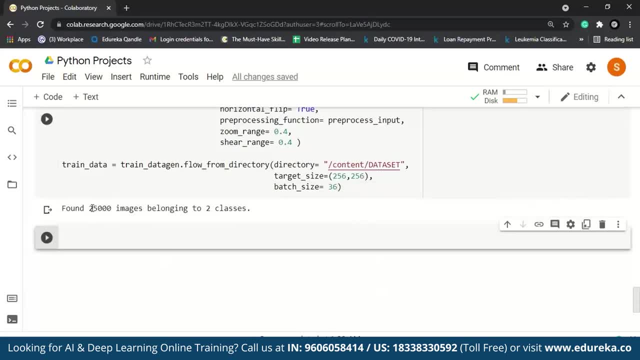 and let's try executing this from now. So, as you can see, here we have 25,000 images which belong to this class and each class has 25,000 image. So if you want to see what is the index value which we have, 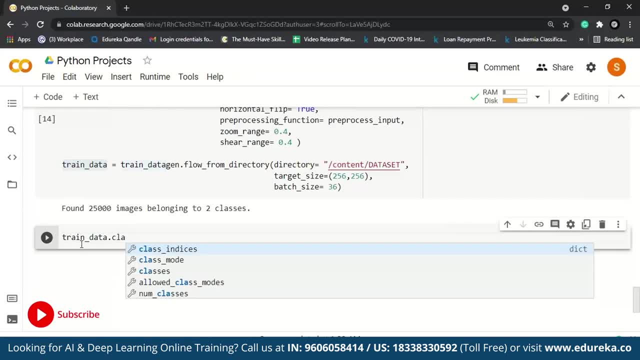 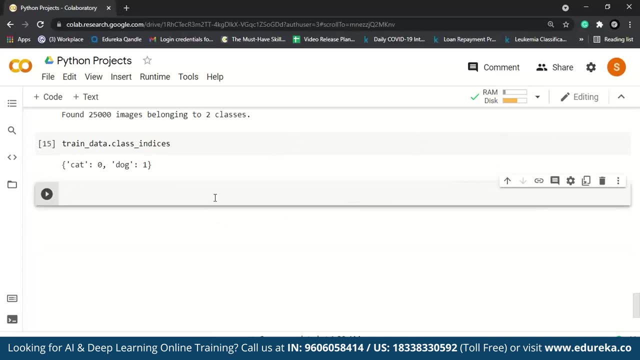 let's say, train data dot index. Now you can see: zero here represents cat and one here represents at all. So this is great. Now, finally, what we're going to do is we're going to train our data. before that, Let's add a model checkpoint. 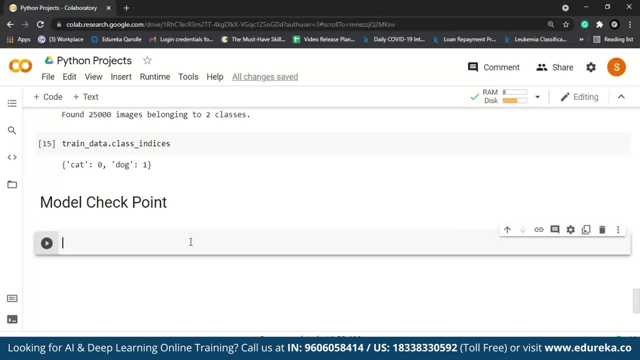 So let me give checkpoint. So before we move ahead for model checkpoint. I'm pretty sure now you might be wondering how does this data would look like, So let me quickly show you that as well. So before we go ahead, let me add that as well. 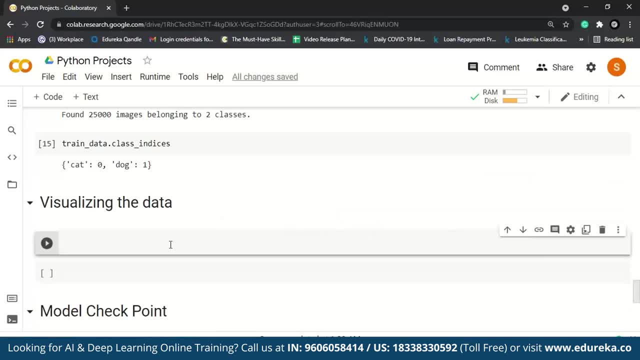 So visualizing the data, right, And let's see how this would look like. So for this, first off, we have this function, that is trained data dot. next, this returns two things. One is the image and the label. So we have trained image and then we have label. 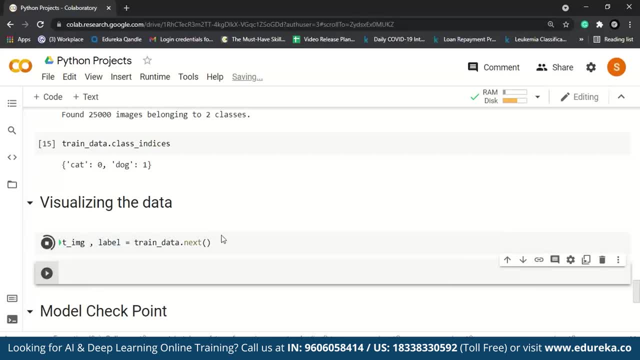 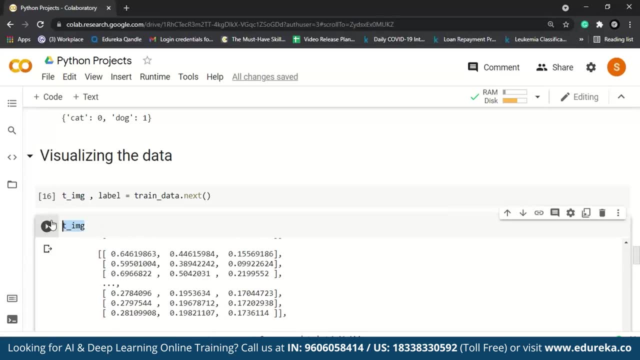 although label isn't that important, But yeah, let's add them up. So if I just see T dot train P image, this is basically, you know, all the images that we have now will pass them one another, like one after the other, and let's see how that would look. 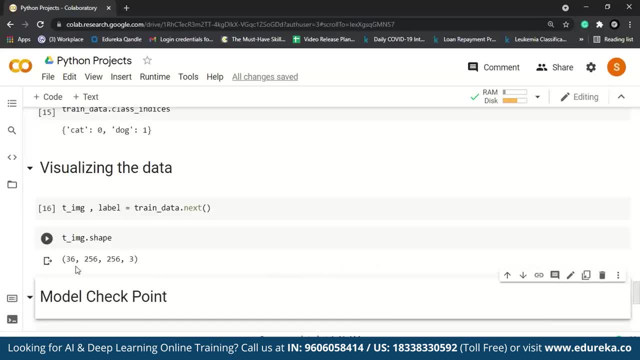 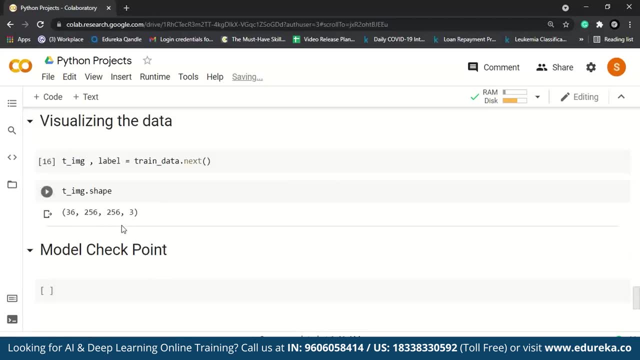 Like. but before that let me see the shape. So, as you can see, here we have 36. if you're wondering why we have 36, that's the batch size that we have given here, and 26 256, 256 is the size and 3 is the number of channel. 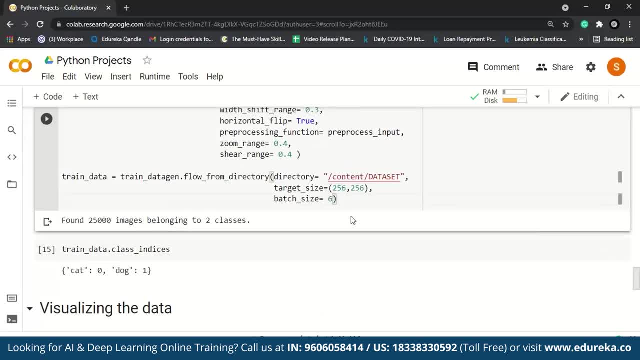 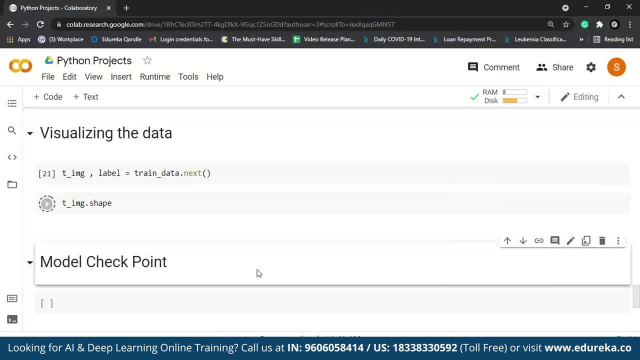 instead of 36.. We can also give batch size as 64. This increase the number of images, and now you can see. our value here changes from 36 to 64.. And now let's try to plot the images. for this We'll create a function. 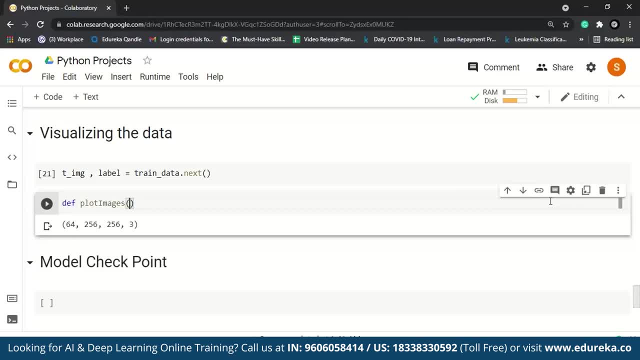 Let's say def, plot image, and we are going to pass image array and then label. Let me tell you what this thing gives. So let me give a comment here. So the input here would be array of images, right? So image array, that is going to be T image and output. 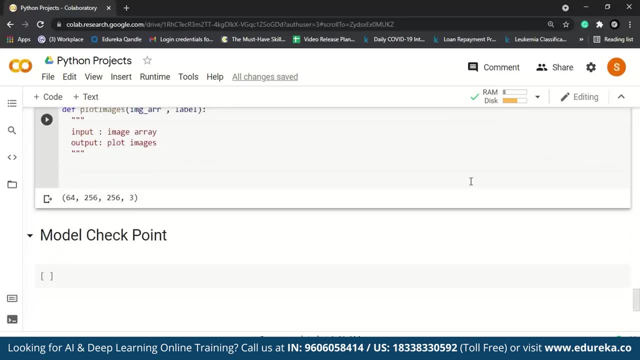 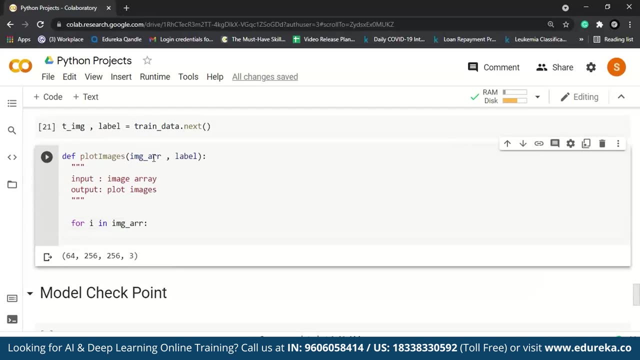 We are going to plot the images. So now what we'll do for I in image array, right? So image array and what we'll do here. if I try to do this, all the 64 images would get printed out, So I don't want that. 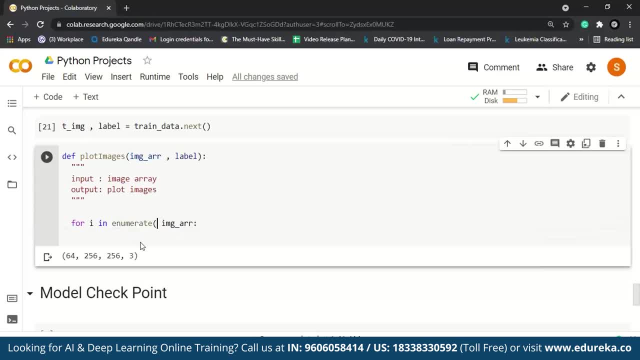 We'll add a function here called as enumerate, and with this I can also get the index over here. What we'll do- we'll give a name here as image index will be IDX and then image IMG. this looks great, And what we'll do here is we'll just print for the top five. 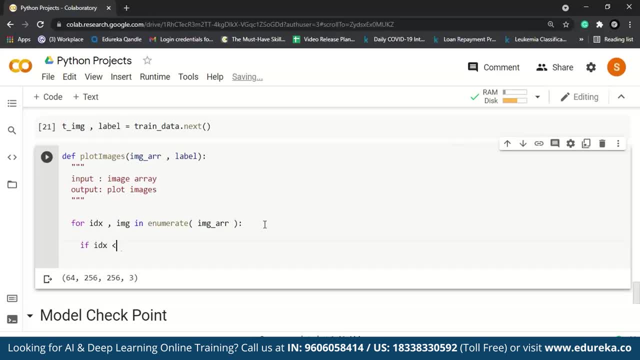 So if index is less than or equal to- let's say, we want 10 images. So if this is the case, then we'll have PLT dot figure. And here we are going to pass figure size at, say, 5 cross 5, then we have PLT dot. 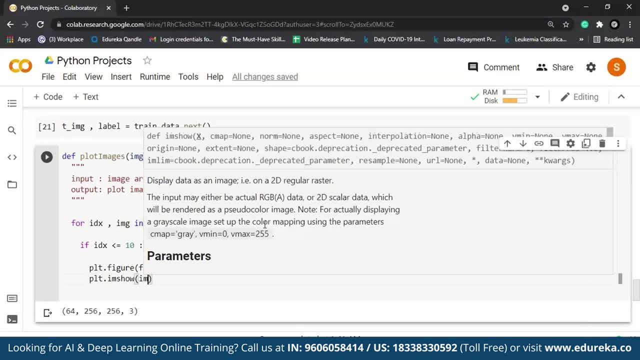 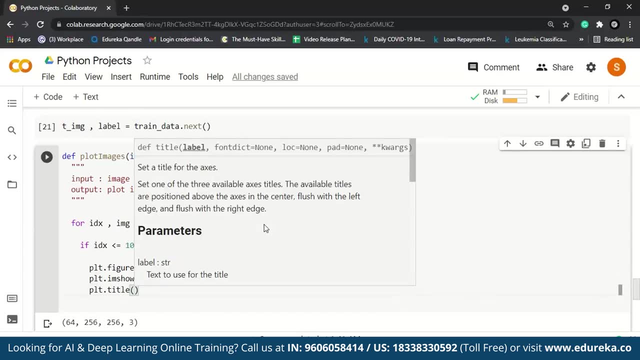 I am sure you're going to pass image here. I am G and the title for this would be PLT dot. title: the size of our image. Let's say the size over here It's going to be shape and finally, PLT dot show we can turn. 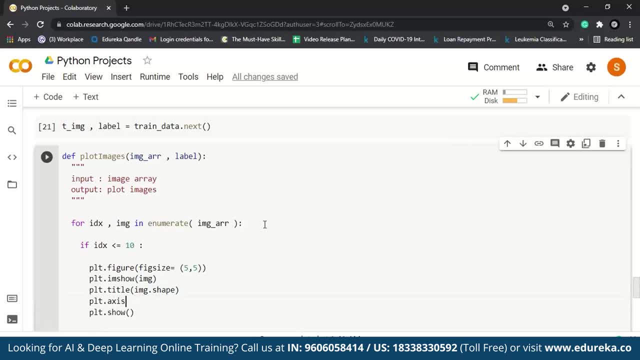 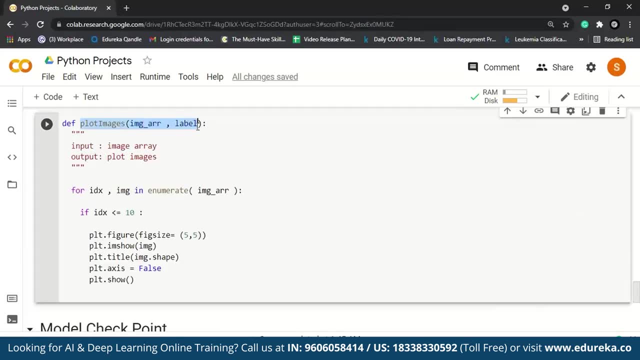 off the axis PLT, dot axis. This can be false and let's execute this. So now all we need to do is pass this image over here. So let me copy this and add a code, and all we need to do is pass this part here, the image. 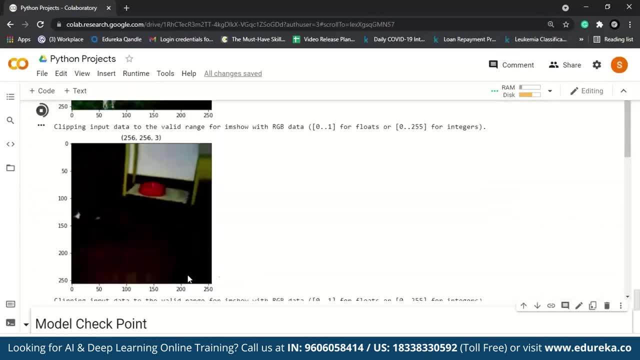 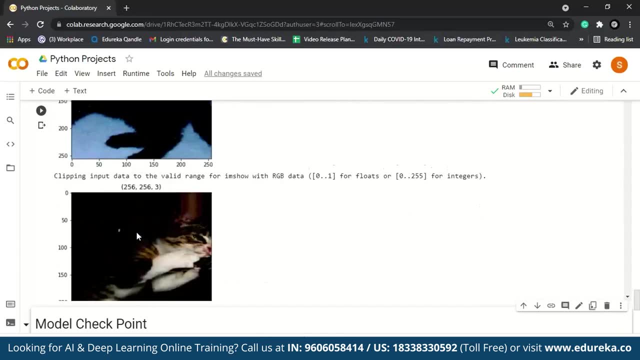 So let's quickly do that and let's execute this. So, as you can see, we have images of cats and dogs and obviously others. data has pre-processed. all of these are pre-processed images and this is how it works. Now, if you want to increase the number of image, 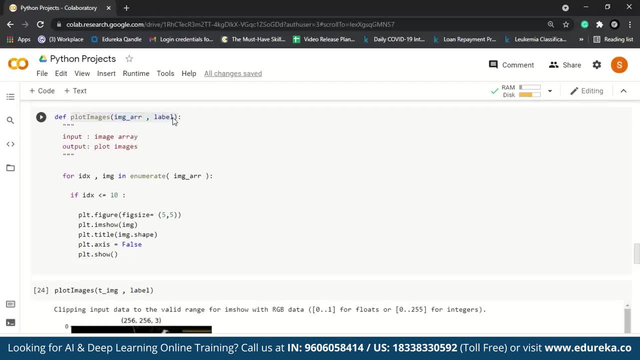 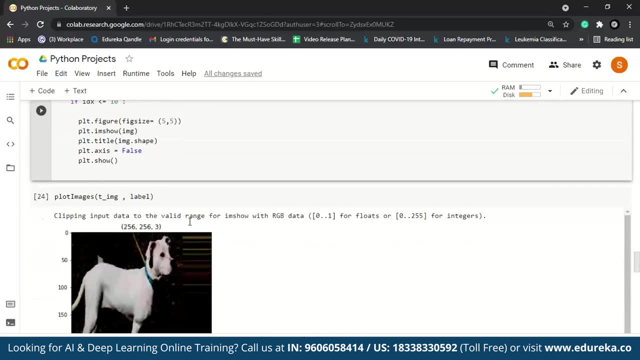 you can definitely do that. Let's try adding label. So instead of this, let's also add label. if I want to add label, then I can add. you know one more value, but let it be for now. So now, what we'll do can just turn off the axis. that's done. 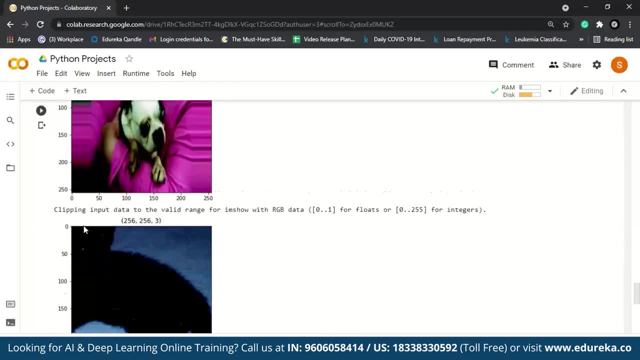 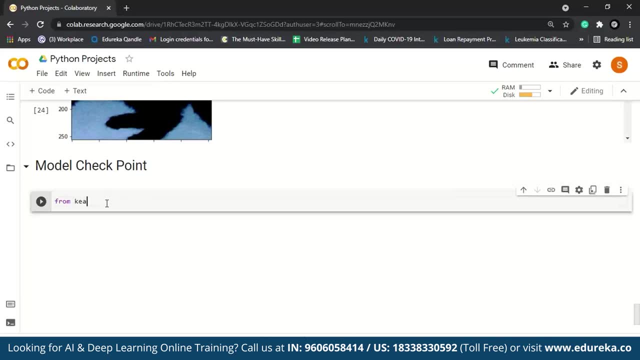 Yep, So this is all that we can do over here, and let's now move ahead and let's try to create a model or train a model. So let's do that. So that is from Keras, not callbacks: import model checkpoint and early stopping, and now we'll just create a class instance. 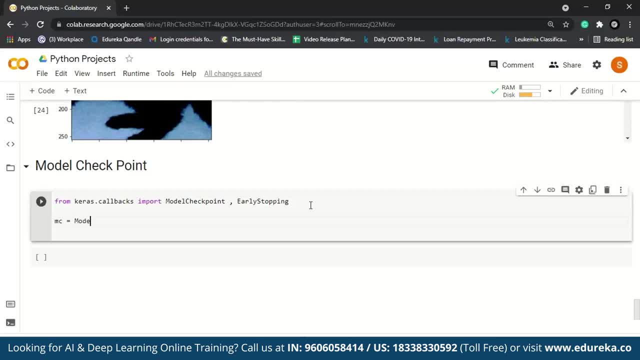 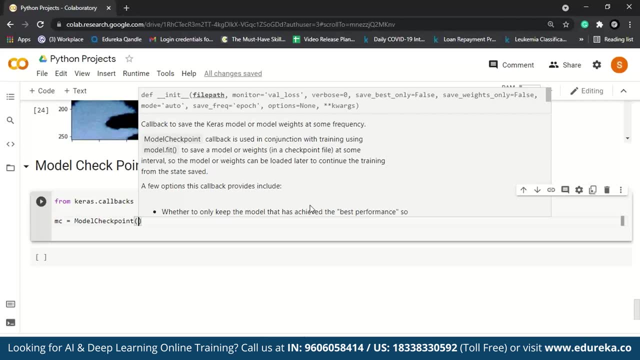 of this. So for model checkpoint is going to be MC and we have model checkpoint. So let's see what are the different parameters. first off, we have file path. you know, this is where our best file is going to be saved. So we'll say: best model is going to be saved here. 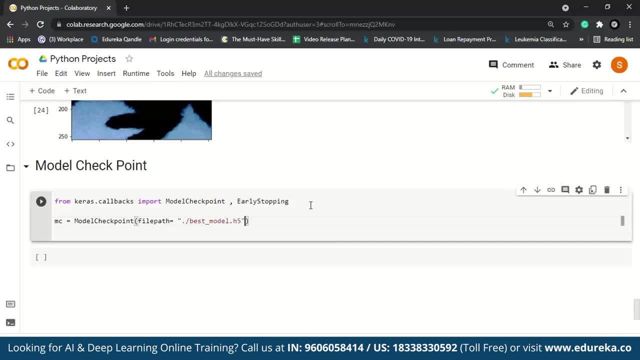 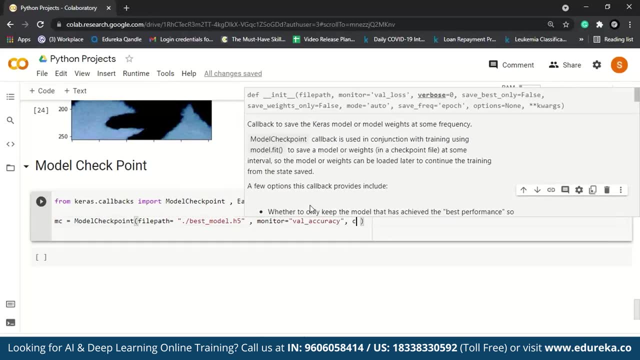 as best model dot h5. So this is great. Then we have to monitor validation accuracy And apart from that we have verbose. we want to see what's happening. So we'll say verbose is equal to one: save the best file or save best. only this would be true. 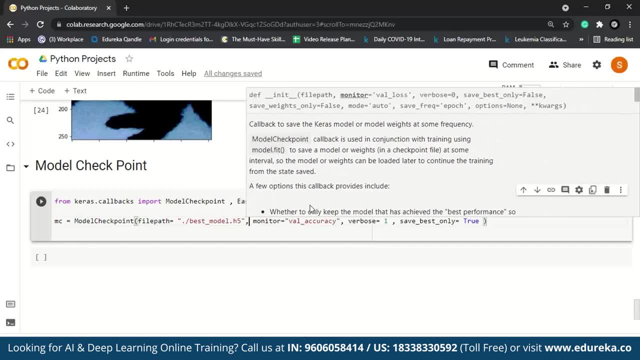 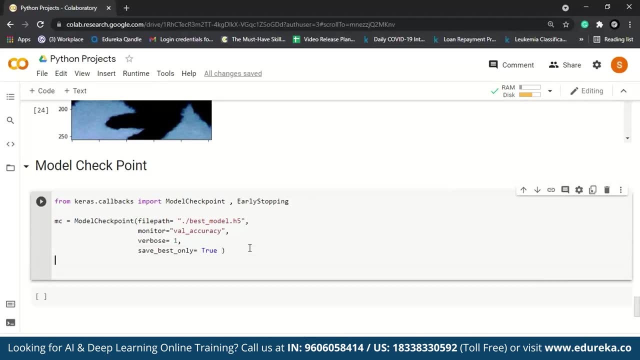 And yes, so this is fine. Let me just rearrange all of these just for better aesthetics. So when we are done with model checkpoint and now we'll come down to early stopping and we are going to say EC or ES, early stopping. So oh, here as well. 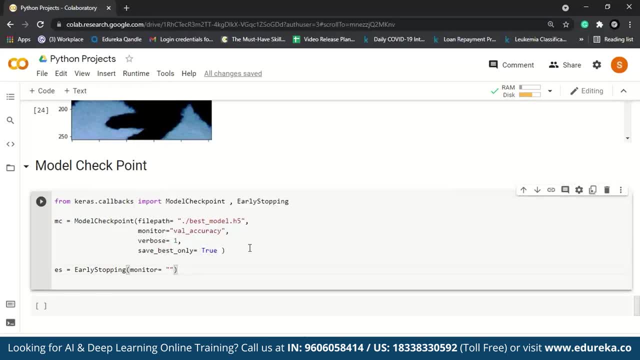 We are going to see what we're going to monitor, So monitor validation, accuracy, And then we have minimum Delta. So here I'm going to keep a big value. as our model is bit complicated, What we'll do is, instead of a big value, 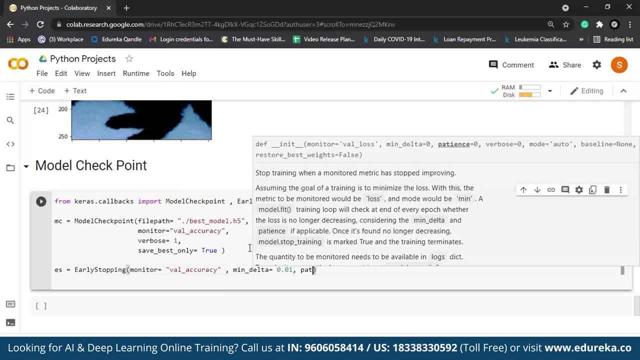 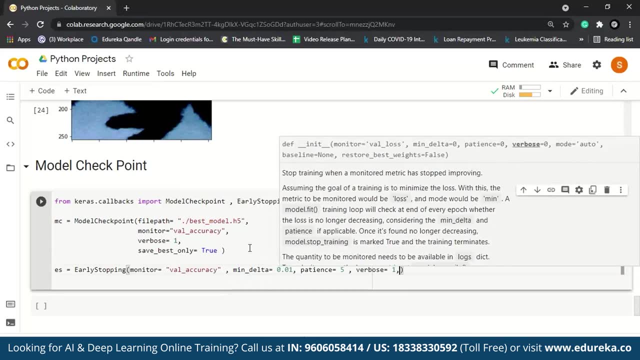 Let's take up a narrower value, So 0.01, then we can have patients. that is the number of times it should wait. So it's going to be five. same here. We're going to have verbose should be one, and more obviously is Auto. 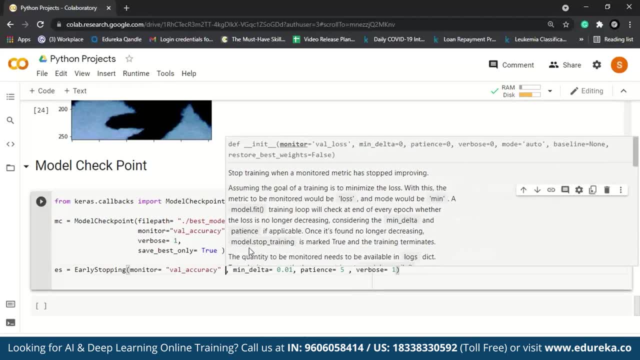 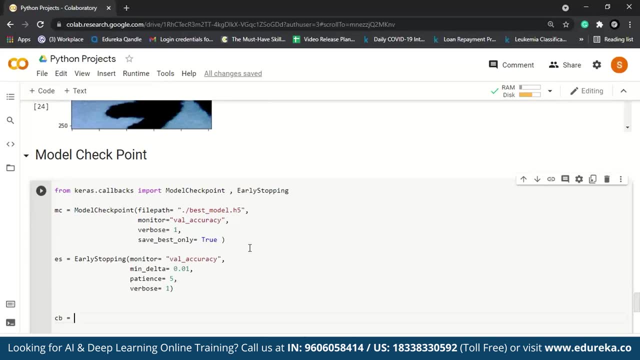 So this should be fine. So now let's try to fix this up, Let's align this and we'll put all of these in an array. So it's BCB, that's callbacks, and we'll have model checkpoint and early stopping, and we execute this and we're done. 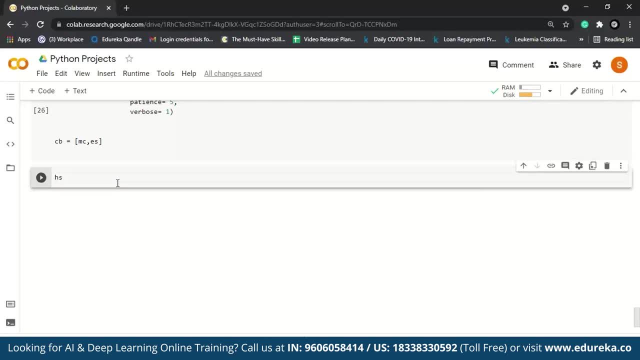 So, finally, what we'll do? we're going to train a model. model returns factor here call as history. So this is going to be his, and then we have model not train, or it's going to be fits, so fit generator. So now we'll do? we have to pass the generator. 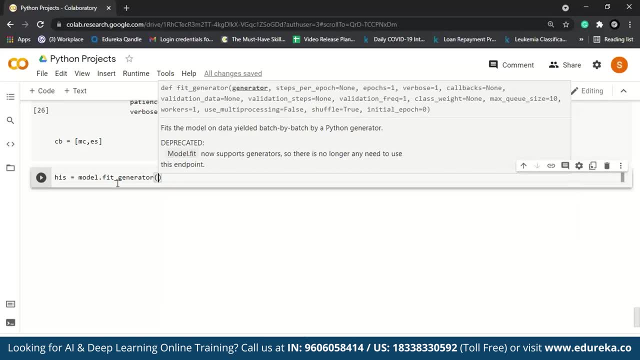 We have test generator, right. So we have test data- It's going to be trained data- and then we have steps per Epoch. Let's say we're going to give steps per Epoch over here as 10. then number of Epochs that I want to follow: we can give 30. 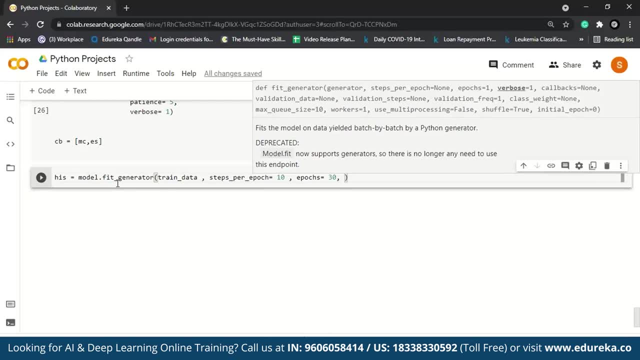 or any number, 300 or whatever- Because as we have callbacks, so once we know that model has trained properly, we don't have to worry about it, and then we'll also pass callbacks. callbacks will be CB. This looks great and let's try to execute this now. 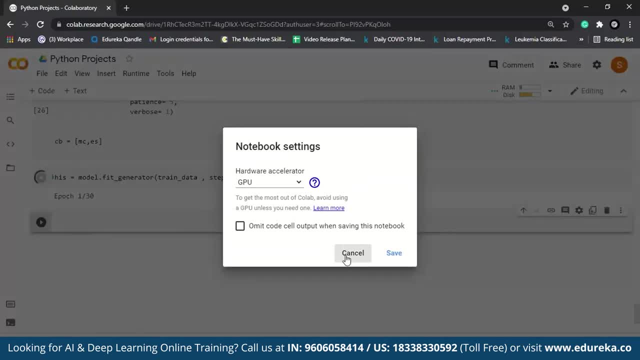 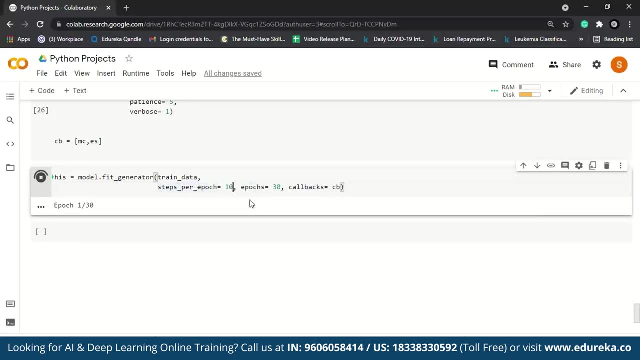 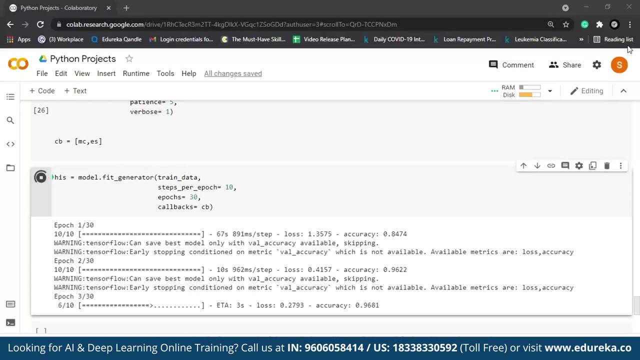 Make sure your runtime is in GPU, or else it's definitely going to take quite a lot of time to train your CNN model. Meanwhile, that is training. Let me just give a proper alignment here And, yes, this should be fine. So, as you can see here, 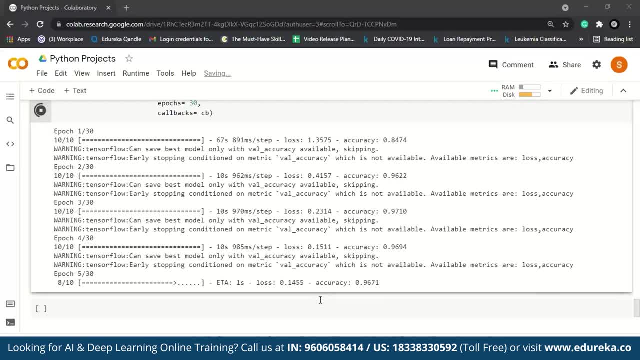 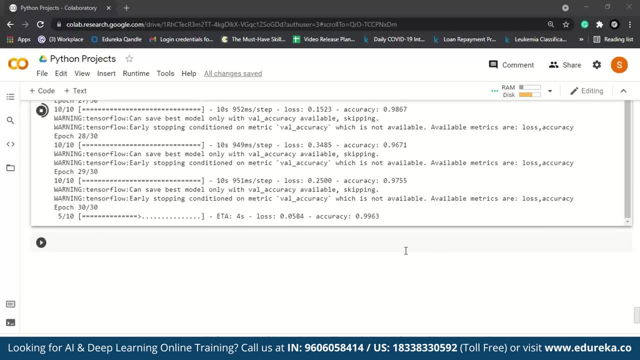 we have done a small mistake. So, although the model has trained, perfectly fine, but the issue is that our model checkpoint didn't work, and the reason for this is because I had done a small typo. So what we're going to do here is- let me quickly take this up- 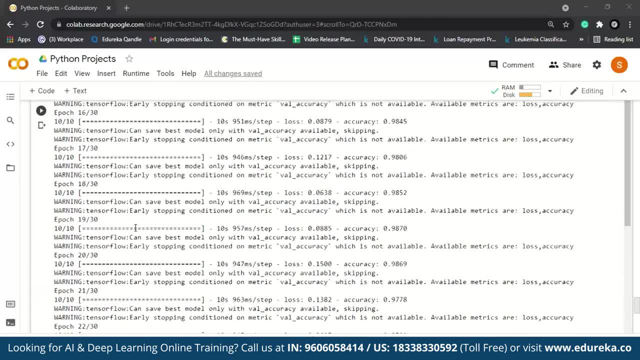 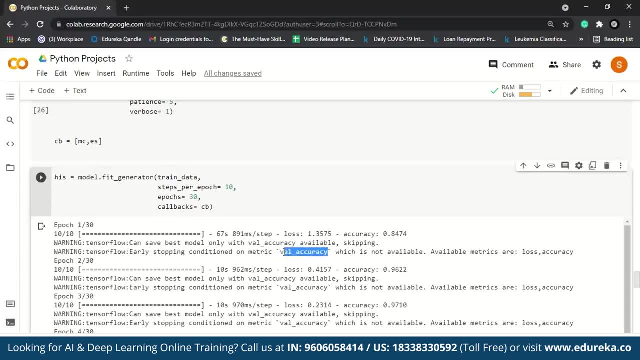 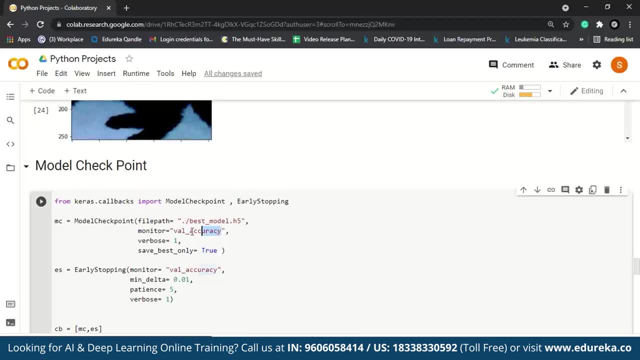 Validation accuracy. and let me come back here and let me fix this up And let me do the same over here. What happens over here is, if I don't try to do this, our model might end up overfitting. Let me do a cross check here once again. 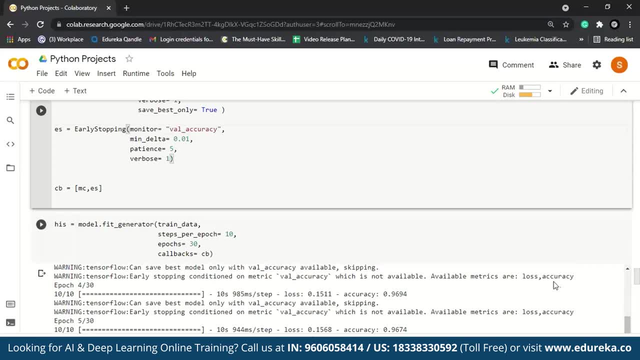 So we don't have validation accuracy here, right? So that's why it's not working. So what we'll do? we'll just take up accuracy and add it over here. So one more thing keep in mind if I try to rerun this. 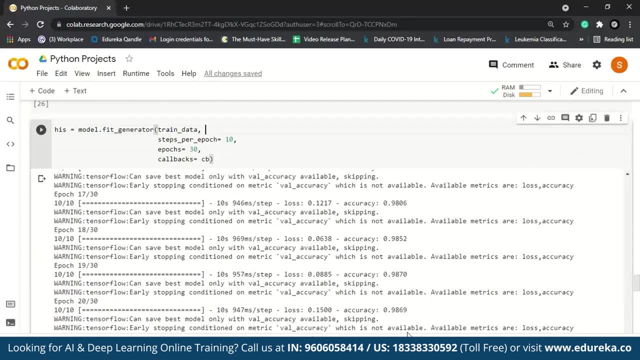 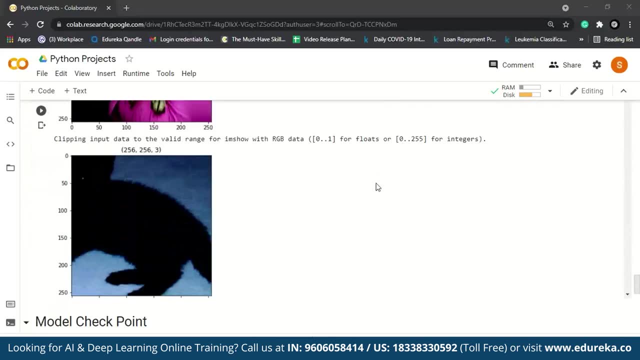 and this block again. So what happens is my model will start training from here, because everything is saved. So if you want to retrain your model, all you need to do is just go back on the top, go to the place where you have, initialize your model. 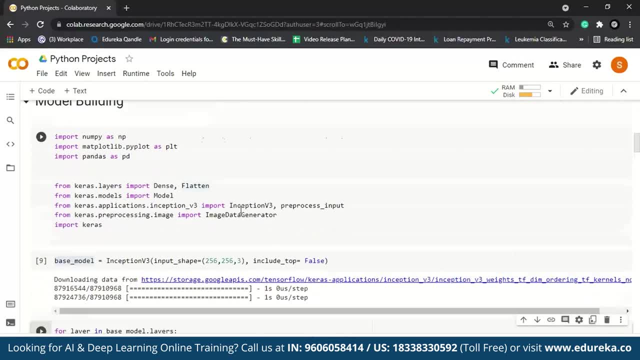 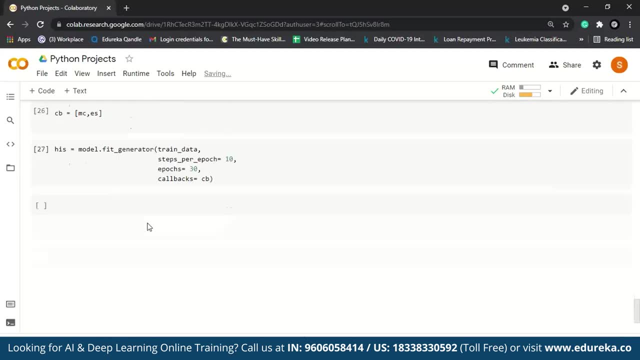 That's over here, And once you come here, we'll just try to run all of these once again. So this is the part where we have to rerun, and once this is done now, all we're going to do is come back to this model checkpoint. 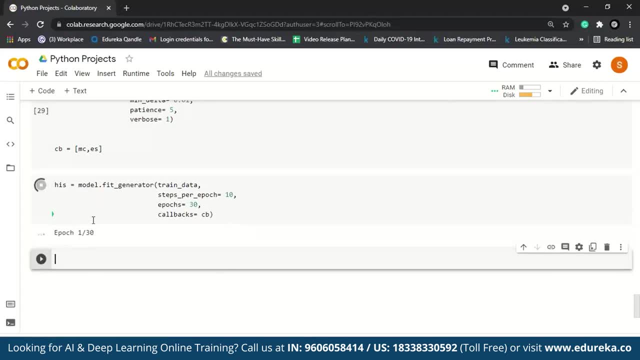 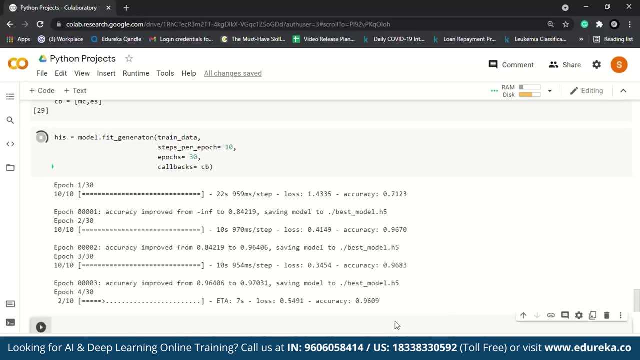 We'll run this and this as well. So now, instead of going through all 30 box, I'm pretty sure it's going to be like very few. So, as you can see our model, stop training at the 9th Epoch, although I could have gone all the way to 30th Epoch. 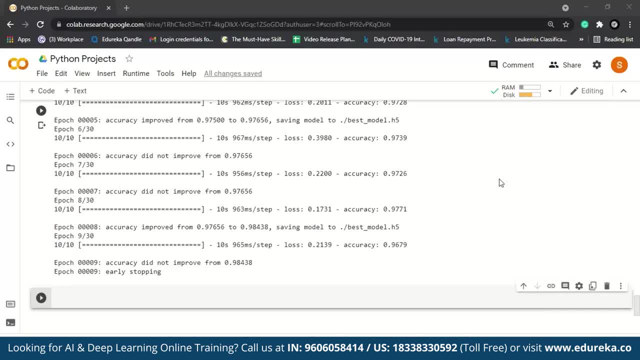 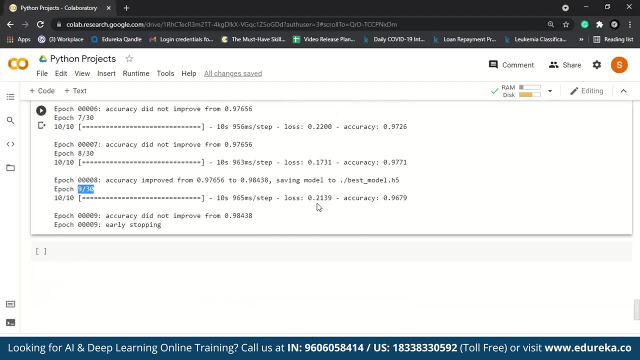 but it's of no use. and apart from that, one more thing I would like to show you here is: initially we had loss here as one and then, as you can see, the loss are decreasing and here again it's point: one person or 10% loss. 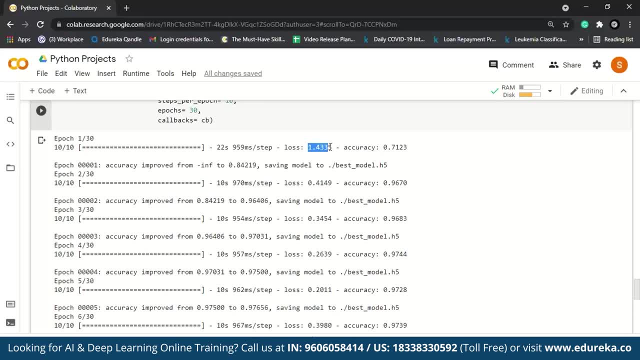 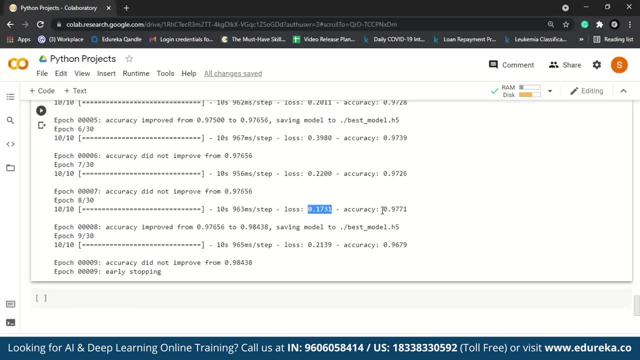 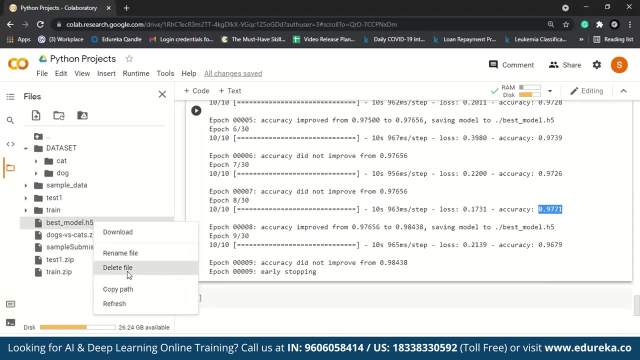 and then the accuracy here is 97%. So that's all for this video. Thank you for watching. I hope you have a great day, Bye, Bye. So whatever the best model is that it gets saved over here in model dot h5. will try to load this model. 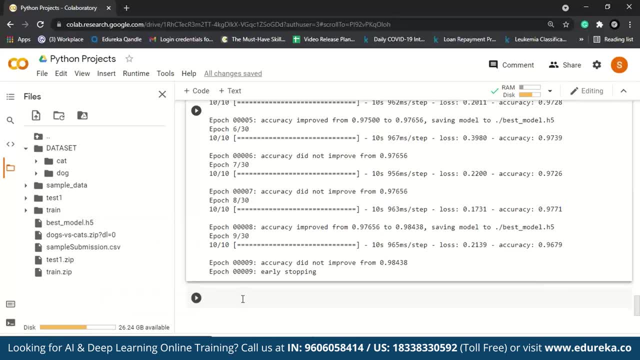 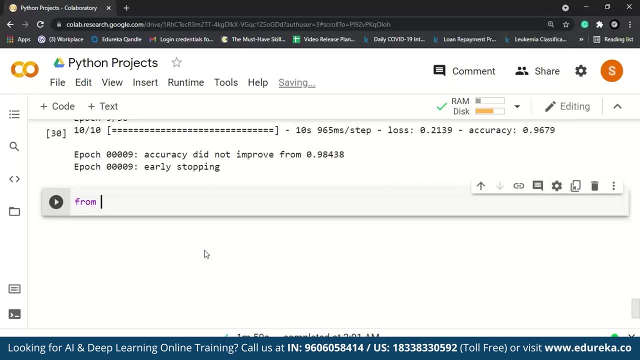 and let's see how our training went. But before that, let me copy this path, Let me add over here from Keras. Let me close this and zoom in a bit. So this is fine. So from Keras, not models, import a load model. 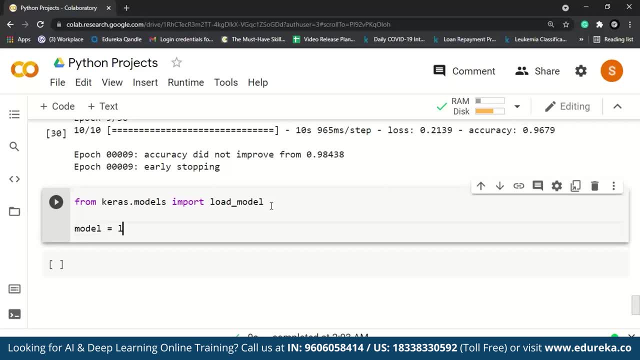 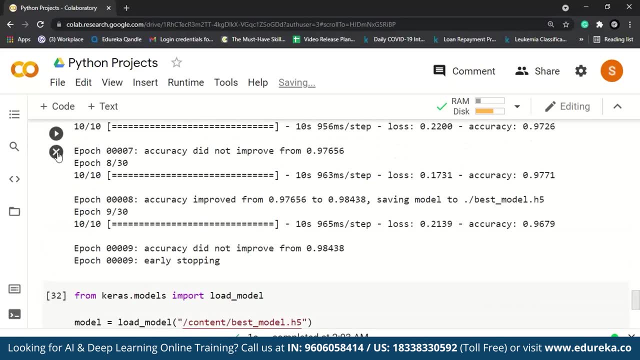 and we'll just give the same name. model is equal to load model and then we'll just pass the path and this should be fine and we just load this up, as I mentioned earlier. Let me close this for now. You know this. we have this history function. 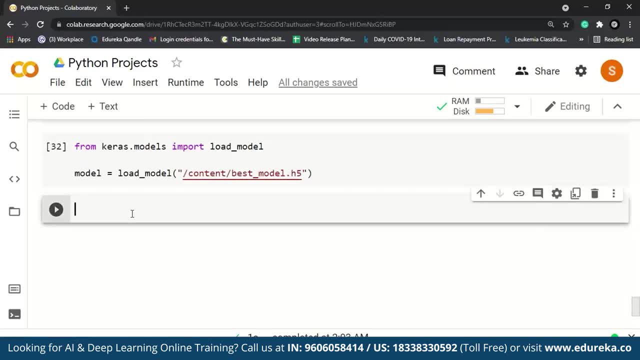 Let's see how well our model has performed. So if you put here, as let's say, H is equal to hist dot history, and now what we'll do is edge dot keys, Obviously there will be just two, that is, loss and accuracy. and let's try plotting them up. 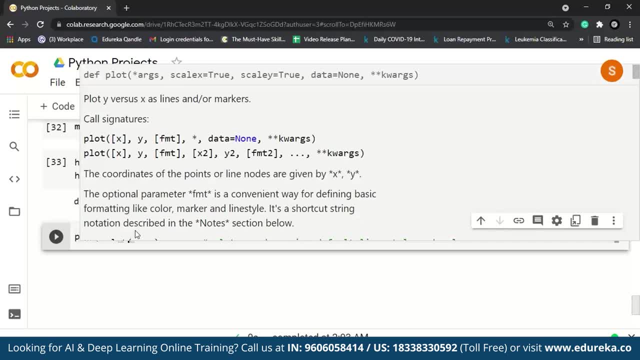 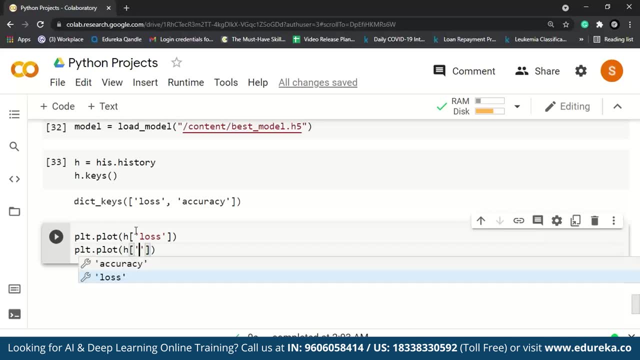 So PLT dot plot, as is the dictionary, We'll just have to press H of loss, PLT dot Lord, H of accuracy, and then we can just say PLT dot title- Let's say loss versus accuracy- and finally PLT dot show- let's execute this. 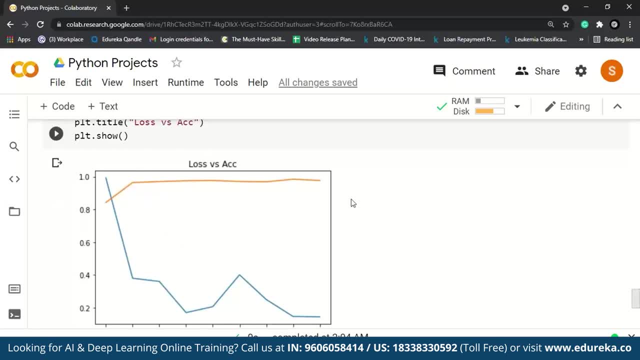 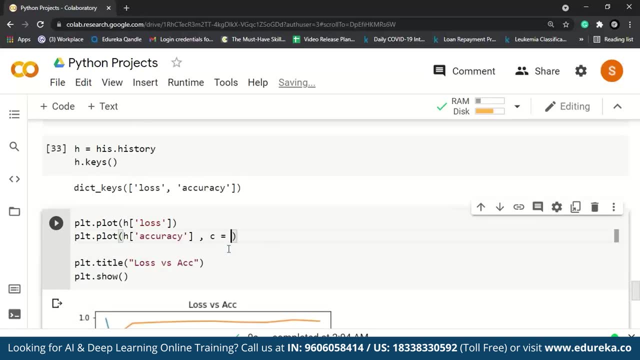 So, as you can see, we have our loss versus accuracy, but we're still not able to understand which is what. let's give a color. this color here would be, let's say, blue. I guess just be would be sufficient, or we can pass this as a string: blue. 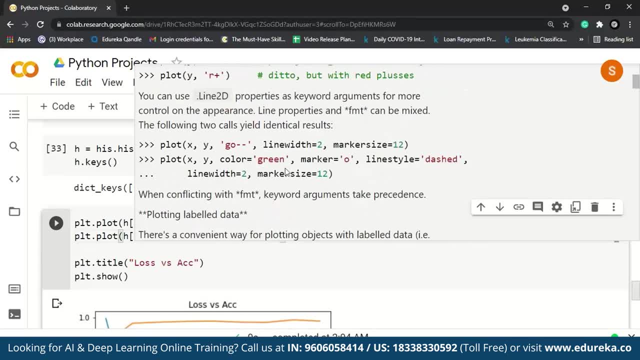 And let's see if we can give any other value here. So what we can do here is: you can see, we can add a marker when we can also add this line style. So let's go with this. Let me copy this and paste it over here. 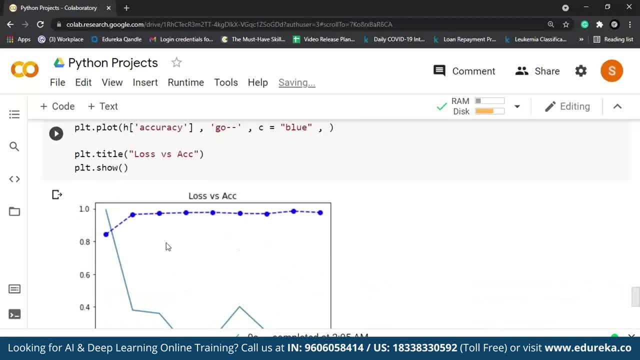 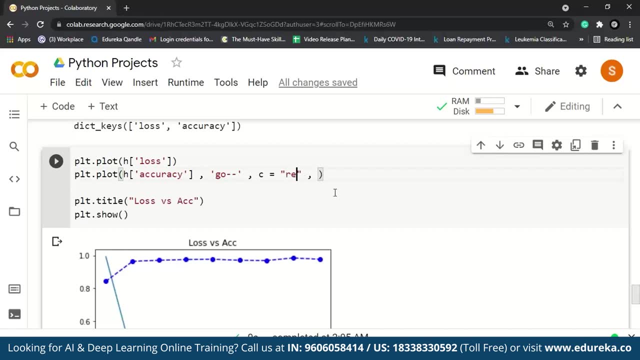 Let's see how this would look like and let me execute this up. So, as you can see, this is what our accuracy here represents. both of them are same color. Let me just change this to, let's say, red, So for every Epoch. as you can see, our accuracy has increased. 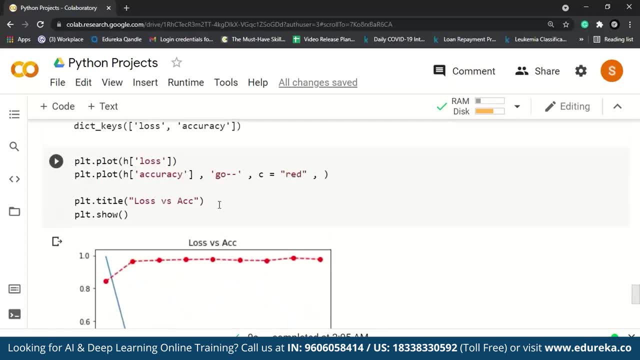 and for every loss, you know, for every Epoch, our losses also decreased. if you want the same thing to be done for our loss, to see how our Epoch has worked, So let me add this and execute this now, So as you can see, right, for every Epoch, our loss value. 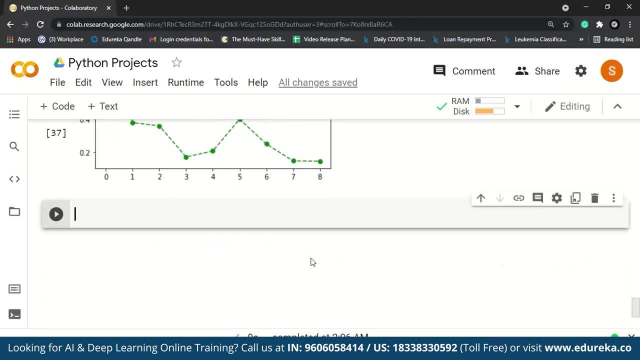 has decreased, and this is the notes below in person now. So this is all there is about, you know, building a model and creating predictions, and if you're someone who is really curious about how well a model is working, what I can do is I can just create a function and pass an image. 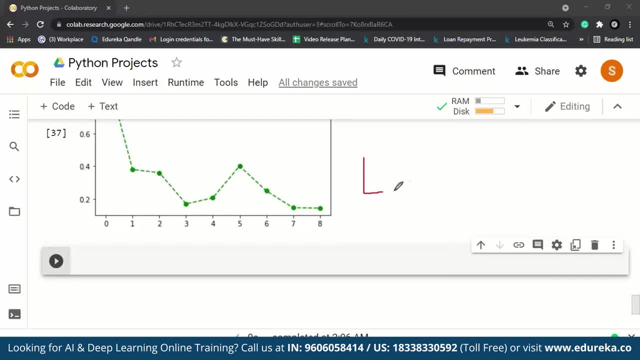 but that's not our major agenda. So our major agenda here first was to build a model, and we'll train this on some, let's say, some class, and over here we are representing cat and dog, and once I have this model I will create a grad cam function. 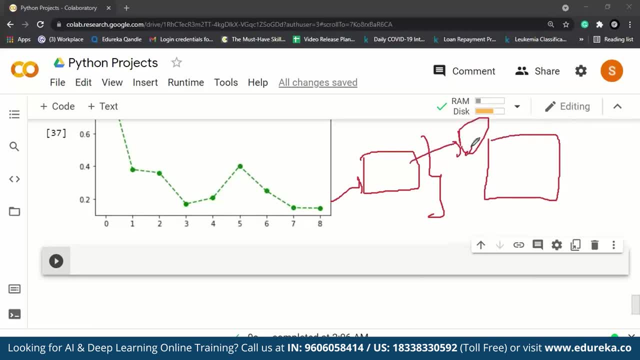 which will take gradients from this deep learning model and it will create a heat map and whatever is my image is going to plot on top of that. So let's not quickly move ahead and do that, But just in case, if you're someone who is really curious, 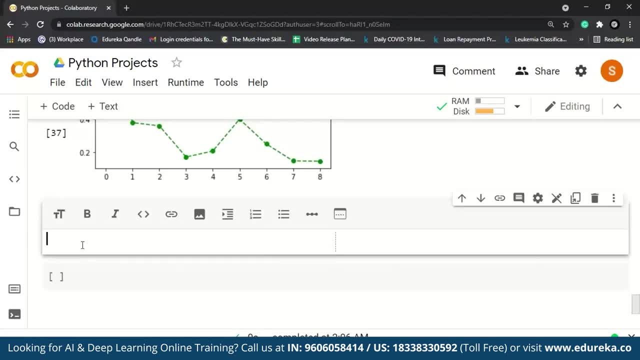 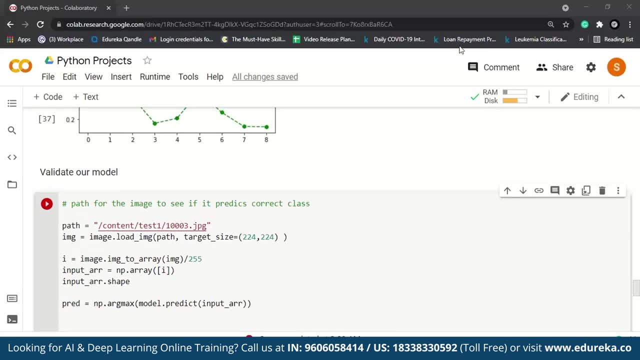 to see what's happening here. let me write a text: validate our image. So I've already written the code for this. Let me just copy that up. So, as you can see, I have written my function here. Let me give this in bold: 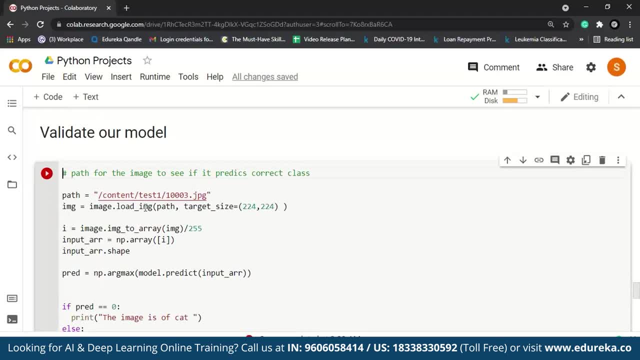 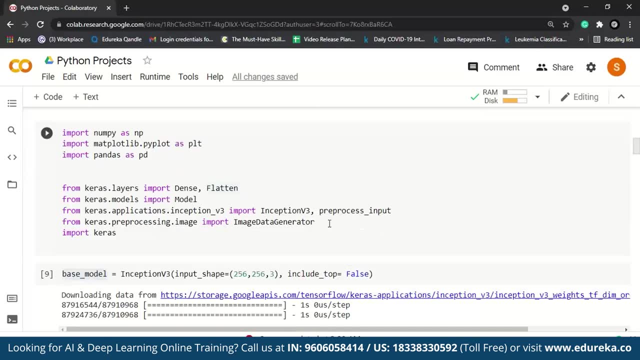 So now what we're going to do here is basically get a path, load the image using load image function for this. We are supposed to import this from our libraries over here, So we'll come back up pre-processing image or here We'll say load image and image to it and we'll run this up. 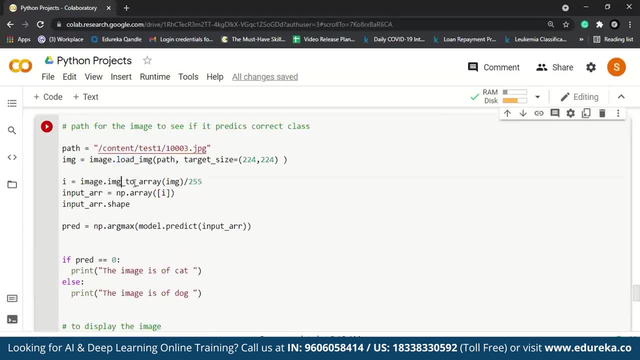 So we'll scroll down, So we have loaded our image. then we convert this into image to an array. So let me remove this and once this converted image to an array. so what we're going to do now is basically try to expand our model here. 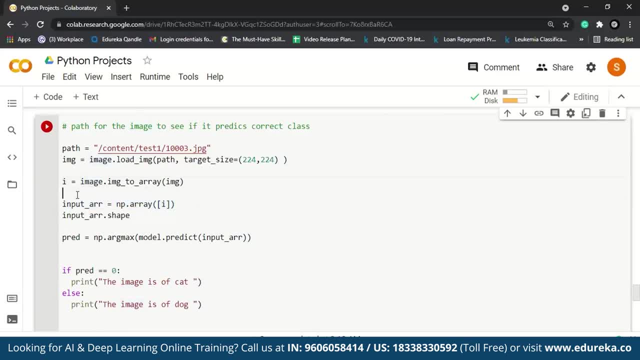 But before that we also are supposed to pre-process our image. So we have I is equal to pre-process input. here We're going to just pass the image that I wanted is I? so pre-processing your input is pretty important and this part over here. 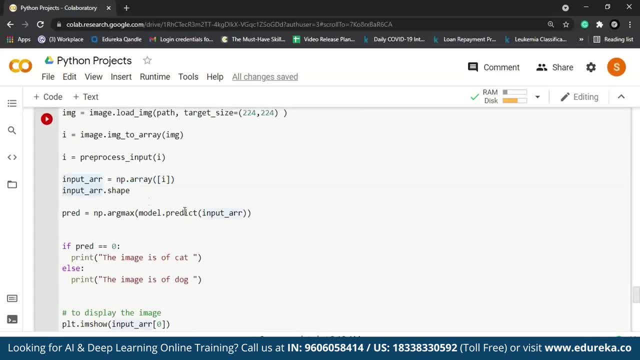 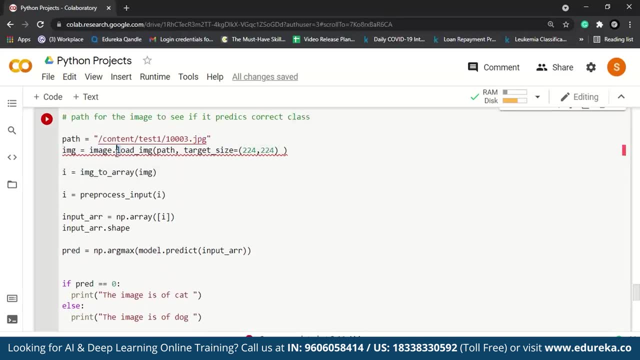 I'm just trying to increase the dimensions, So which we can see over here. So let's now execute. this says: image is not defined. Maybe that's because of this, as you already loaded here, right, So we don't have to provide that. and one more thing here. 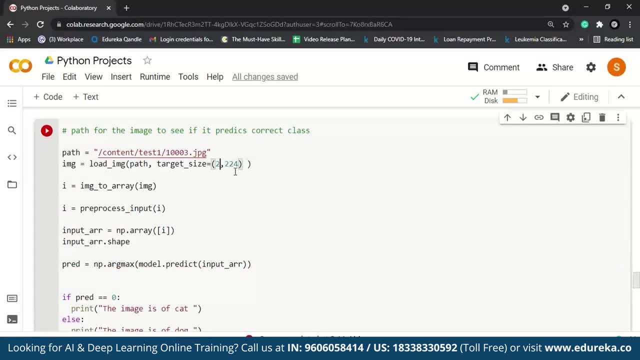 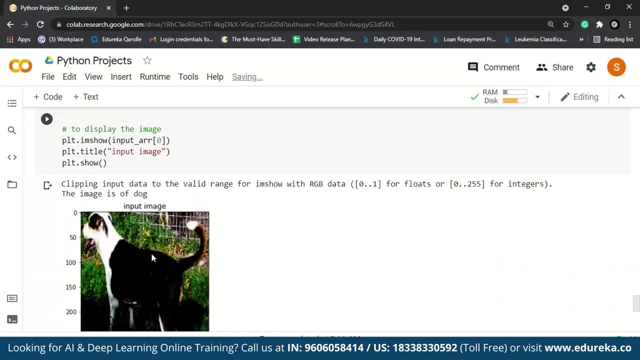 is: make sure your size is same. It's going to be 256 comma 256.. So, as you can see here, model has predicted it. fine. So images of our dog. and the reason why you're getting this initial error is because we haven't regularized it. 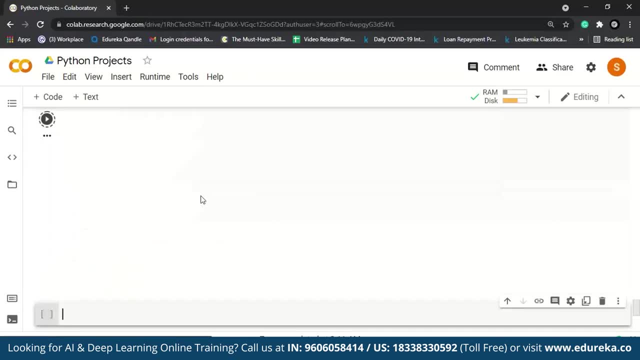 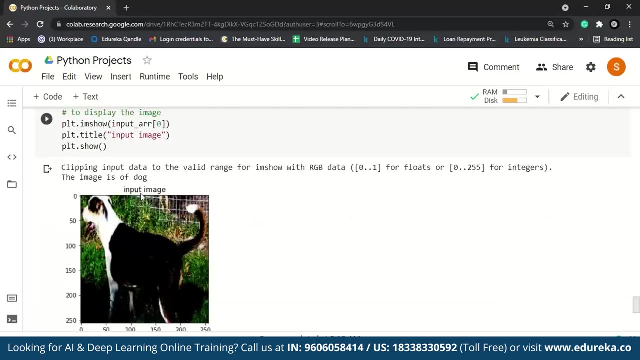 So, if you want, you know, all you can do is divide this by 255, and so you cannot divide this by 255.. The reason is because you know we have already pre-processed it, So this will remain the same and this is what it is. 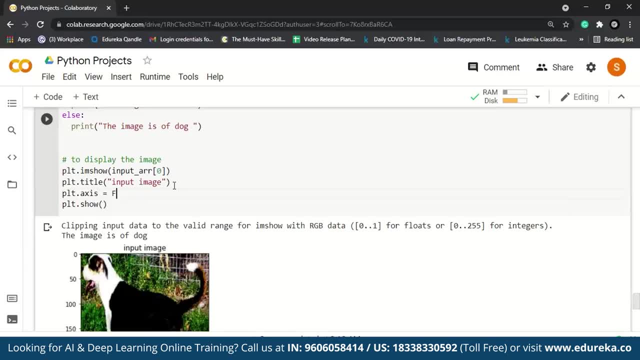 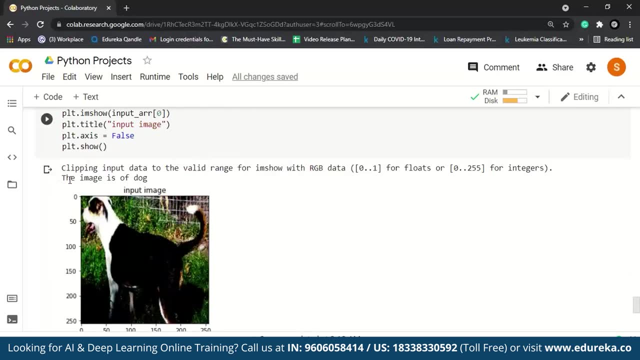 I can remove the axis. PLT dot access will just turn this as false. And yeah, so this is what happened. So, as you can see here, our model has predicted fine. So the images of a dog: and yes, the image was indeed of a dog. 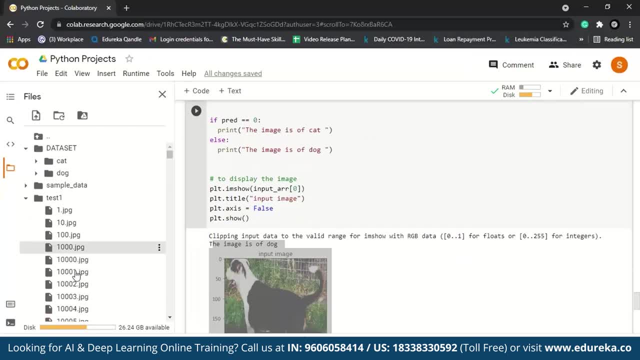 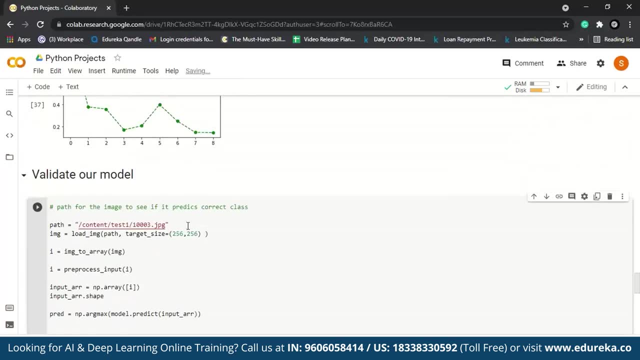 We can take some other random image Now. let me zoom out. So let's say we'll take any random image. copy the path closes up for now and try adding this to the path over here. So let's see What is this image of and, as you can see, 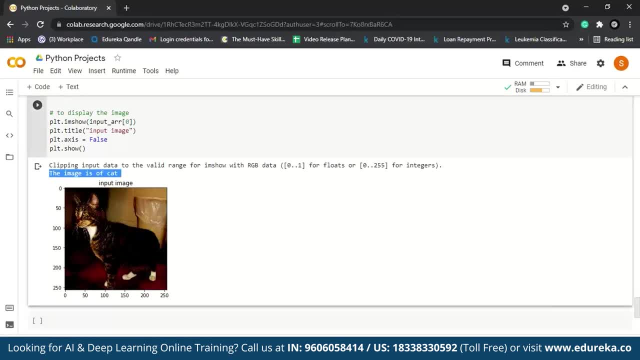 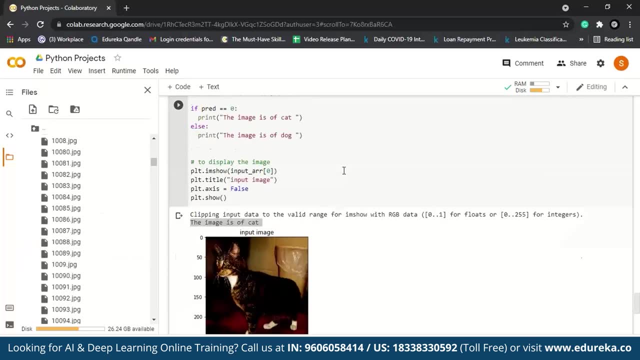 this image is of a cat and a model has also predicted that this image is of a cat. and just one last thing: before we move ahead So randomly, let me choose any value, Let me take copy path, come up here and pass that particular image. 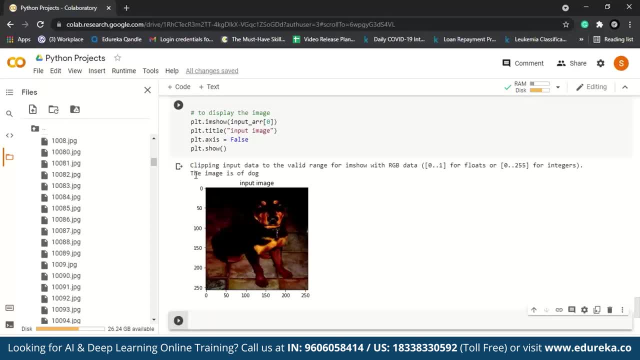 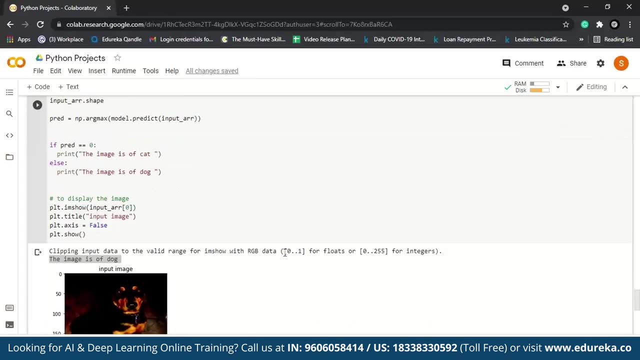 Let's now see what we get. So, as you can see, this is a dog and our model has predicted it. It says: this model is of a dog, So now that we know what exactly is happening here. So what we'll do is: now we'll try to visualize. 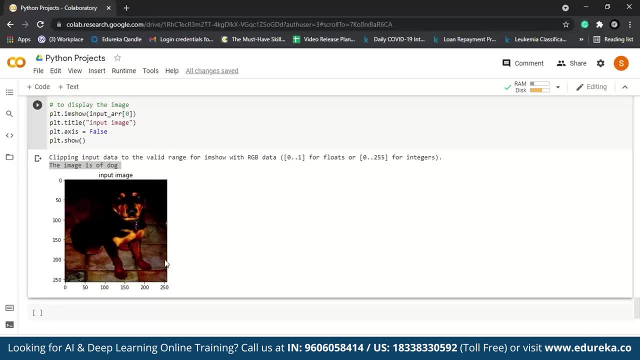 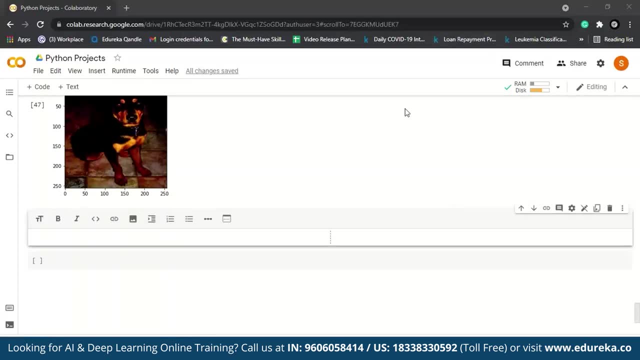 what makes our deep learning model thing, that this is of a dog. So what feature here represents that of a dog? So for that we use something called as grad cam. So let me write down here, So let me give a title here. Let's say grad cam visualization. 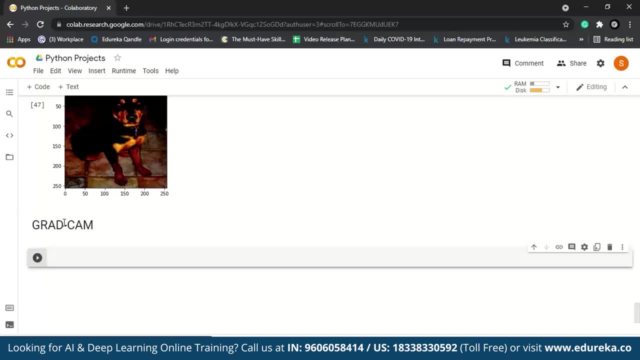 So grad cam. So if you're someone who's wondering what does this grad cam represents here, Well, grad cam over here is basically class activation map. So gradient, class activation map. So that's what grad cam represents. Let me just put this in bold and execute this up. 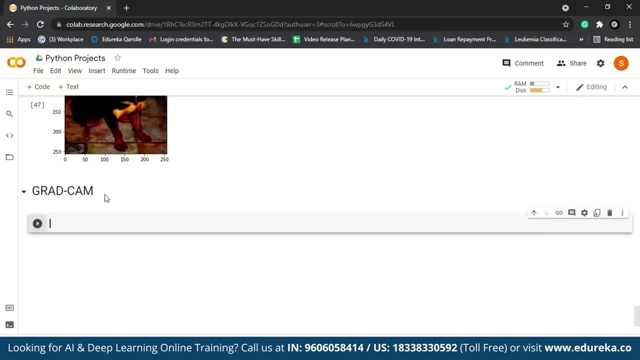 So this is what grad cam is. So what we're going to do, first off read the image and then we are going to extract the gradients from our image and then, finally, we are going to display that on a function. So first off, over here. 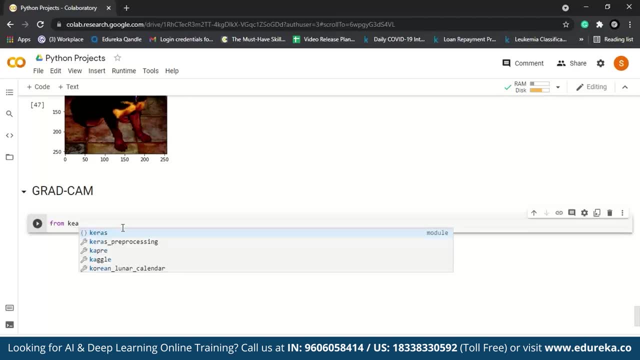 what we're going to do is from Keras or pre-processing import image. Okay, that's something which I've already done. So now what we'll do is TF, get major, and here we are going to just give the path, IMG path. So now, what we're going to do? 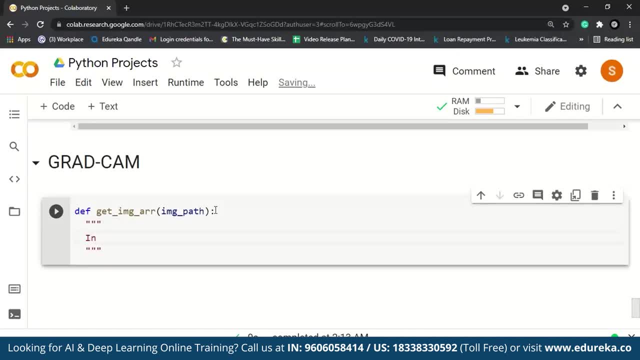 let's try to write some comments here. So what does this take as an input? input here is going to be like: takes in image path and output over here basically be like: gives a pre-processed image. This is basically similar to what we had done earlier. 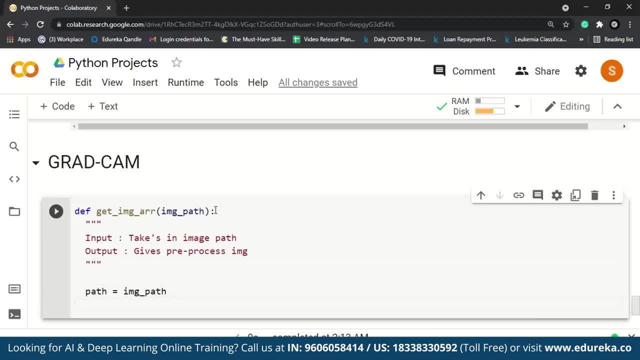 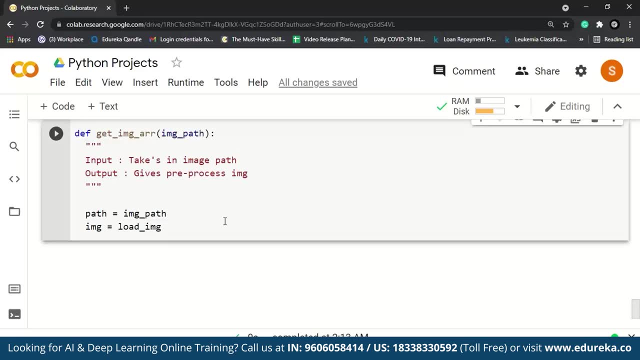 So, first off, we have path- this would be image path- and now we have image- IMG. Let me scroll up a bit. So we're going to have load image and we're just going to give target size and all that. So what we'll do? we'll just copy this from here. 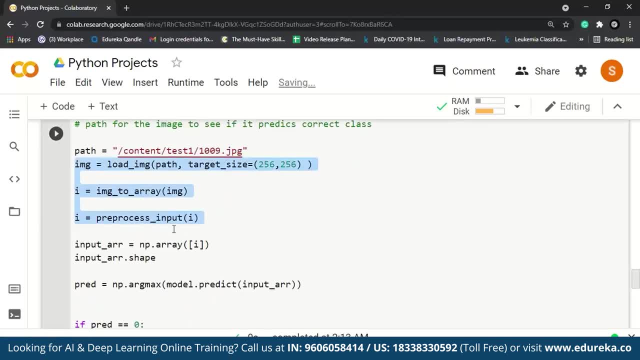 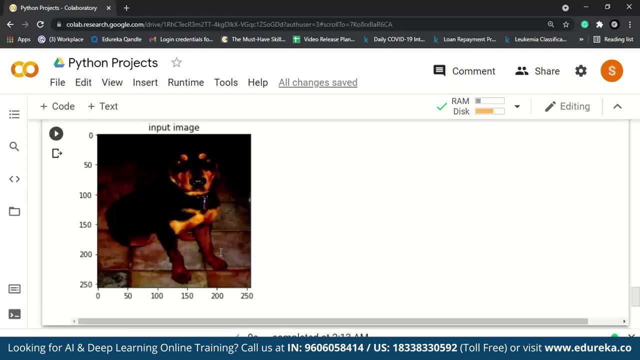 Obviously, first off, you're going to load our image, and then we're going to convert that into an array and then, finally, we have to do all of these. So we'll just do it here, copy this and add this over here. Let us give a proper indentations. 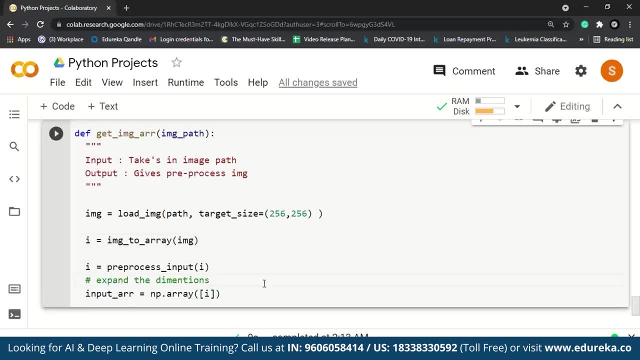 So basically, here we're trying to expand the dimension. The reason for this is because, you know, model takes in the batch size, then size of the image and then the number of channels. So if it's 256 comma 256, we should have number of channels. that's going to be 3. 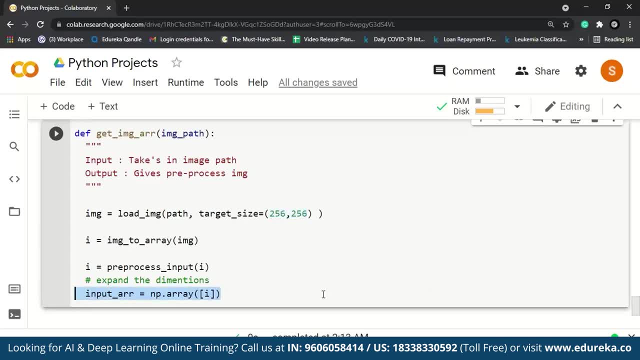 and batch size. that's going to be one. So this is what this function does. either you can use this or you can use numpy dot expand dimensions. That's totally up to you. Let's say this as image will actually change this for all IMG, and even this would be IMG. 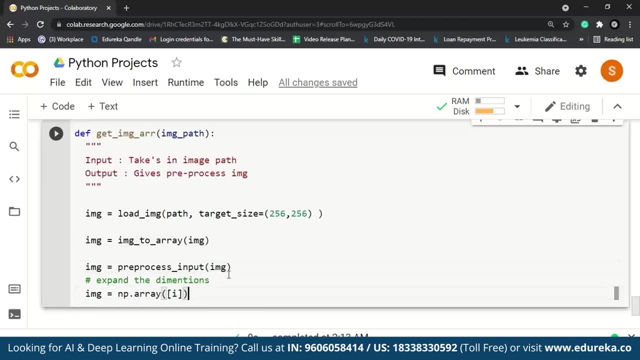 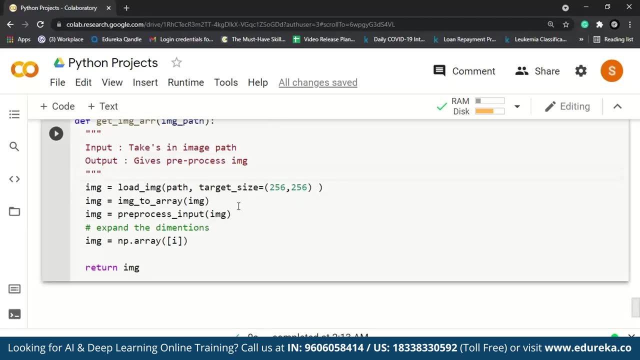 and we'll add this as well over here, And finally, this would return as image. So I hope you understood what we're trying to do here. This is a pretty simple stuff and let's execute this. So this looks great. So now, finally, what we're going to do. 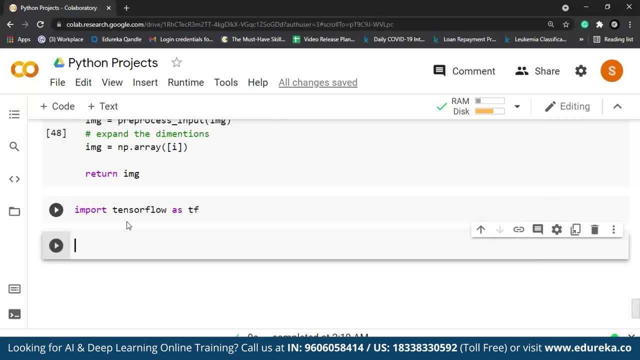 We're going to import tensorflow STF, and now we're going to write a function for our grad cam. So what does this function do? Well, this function is basically used to generate the heat map in our artificial neural networks. So this is a pretty advanced topic in deep learning. 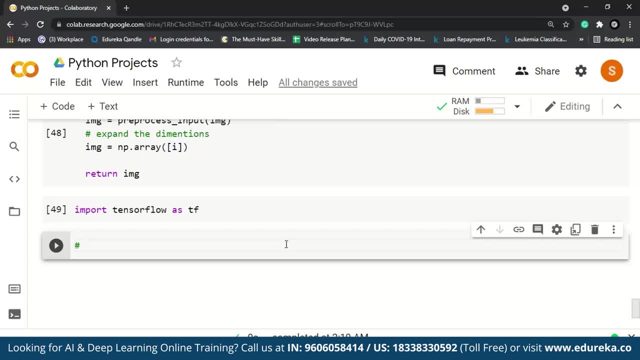 and if you're someone who is totally new to this or definitely first recommend you to go back to the basics, You can start off by looking into our deep learning full course videos and then you can come back here after doing some research on gradients and how this deep learning models work. 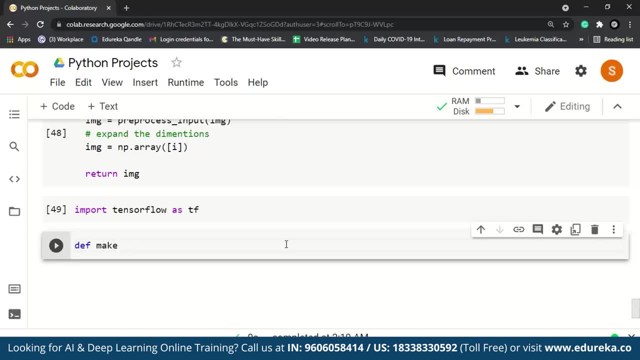 What are we going to do? We're going to create a function. So let's say, make grad cam heat map. So there are a couple of parameters that this thing takes in. It takes an image array. So the image array is basically what we are going to have over here. 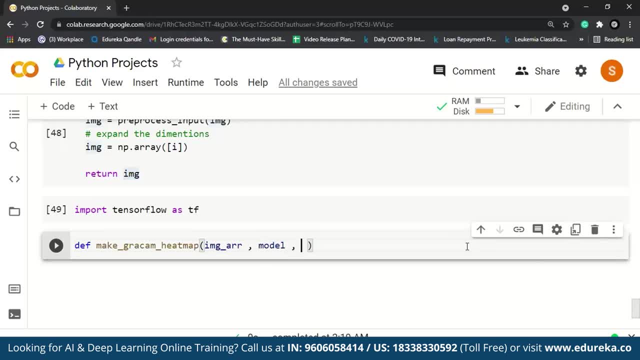 and then it's going to take in model. then we have to take the last convolution layer name And then we also need to provide predicted index to be false. So Fred, index will make this as none. So this is great. Now what is the last layer of a convolution layer? 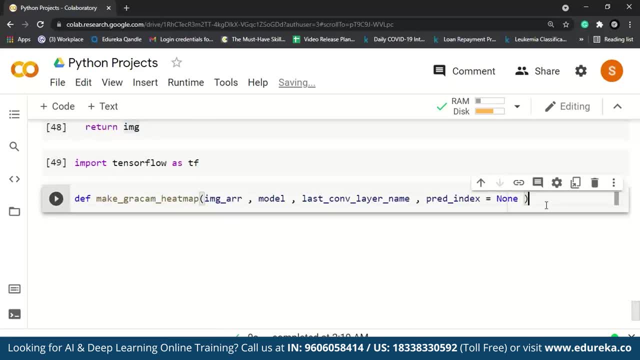 We can just scroll up and see the summary. We'll get to know that, but meanwhile let's just get on to this now. So what we're going to do here is: first, we create a model that Maps the input image to the activation functions. 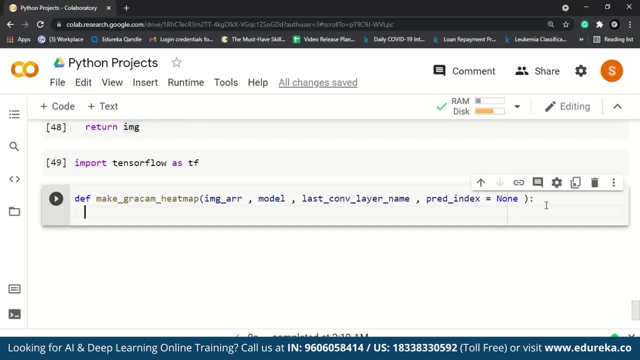 of the last convolution layer, as well as the output predictions. So we're going to create a model here, Let's say grad model, and for this we can use either TF dot Keras or you can just directly use Keras. So for a change, let's use TF dot Keras. 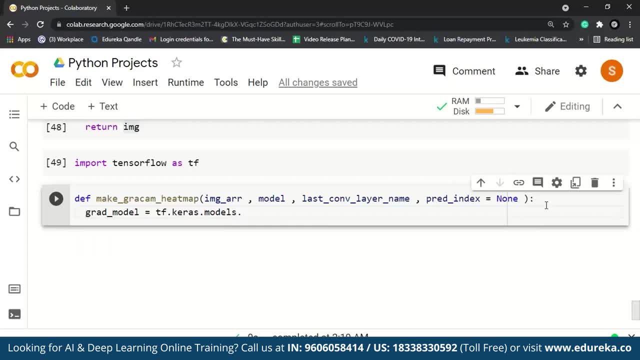 We know that there are a couple of models, So we have models dot model. We are going to use this. So for this, what we're going to do, we're going to pass in couple of values, So it will be model dot input. 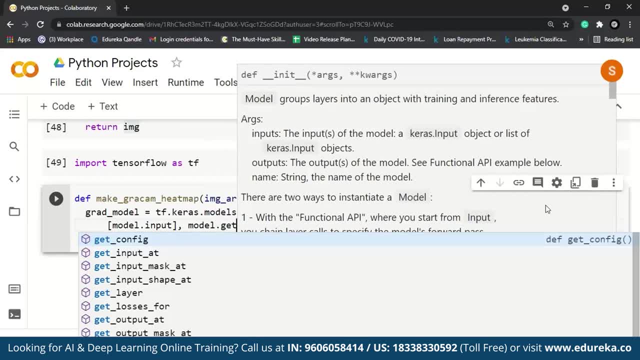 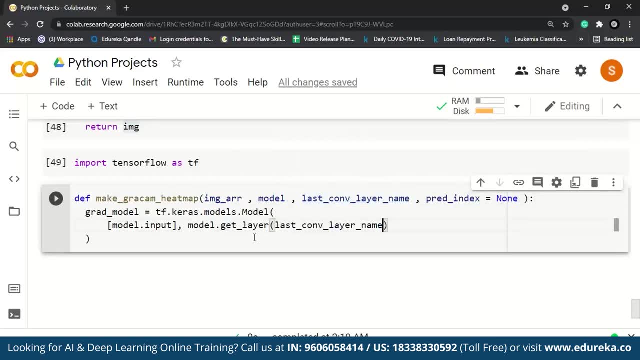 and then we have model dot- get last layer. This is where we are going to, We're going to pass the last convolution layer name, So let me copy this and paste it over here. and we want the outputs of this. and then, finally, we have model or output. 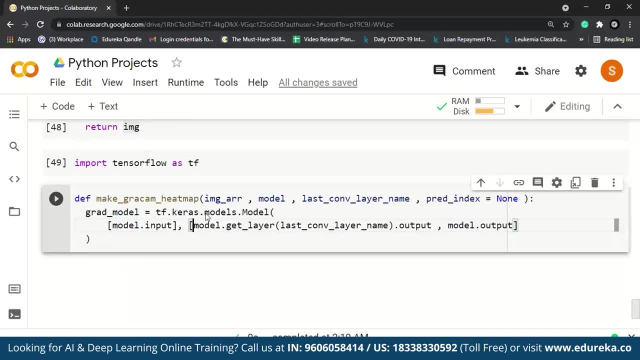 and let's add this thing into a bracket here. So this is what we are doing: We are created a model where we are having input layer and then the gradients from our last model and then the output of a model. So now that we have done this, 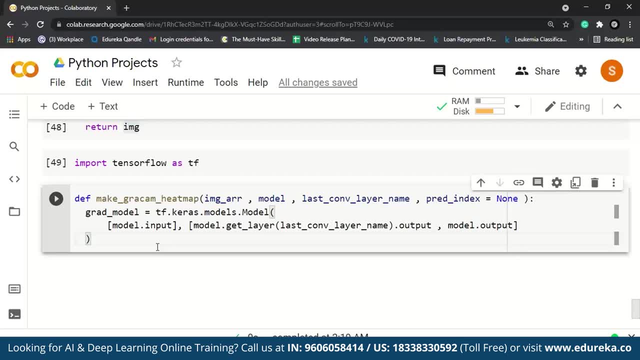 So now what we're going to do is we are going to compute the gradients of a top predicted class from our input image With respect to the activations from our model, which is present in this last convolution layer. So this is the only way that we can access the gradients. 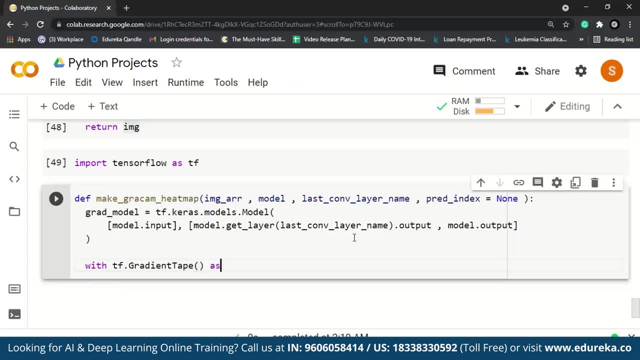 So we have this TF dot gradient tape is a function, Let's say as tape. and now what we'll do is last convolution layer output, last convolution layer output, and then we have the Preds. This is what is written by our grad model. So we have our grad model here. 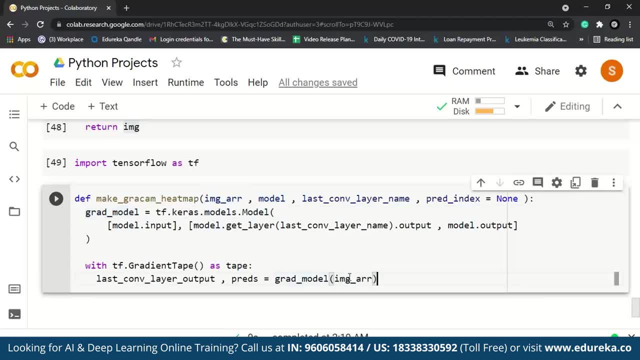 Let me copy this and over here I'm going to paste the image array. So this is where we are going to try to predict a model. So now, what we'll do if pretty index, that is this part for the index, if this part is none. 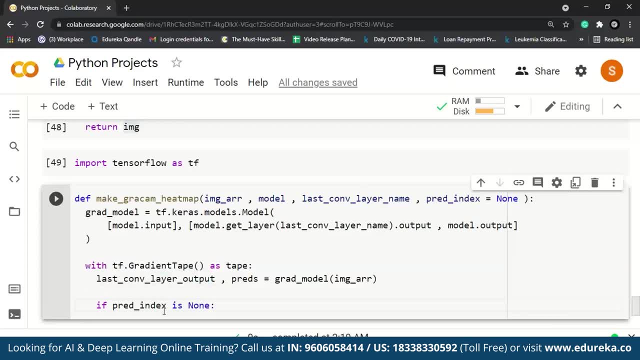 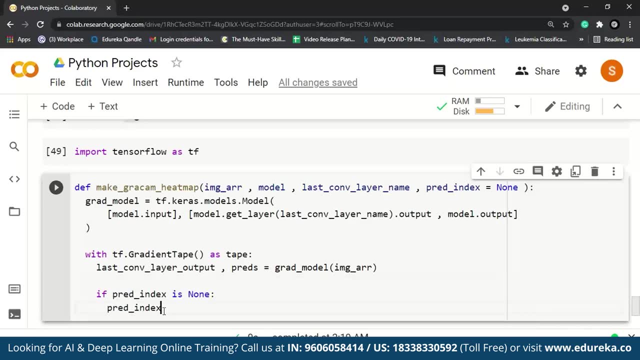 let me copy this and paste: here is none. If this is the case, then what we'll do is we just provide the predictions. we have dot argmax, pretty index. Let me copy this again. This will be TF. We can also use NP dot argmax. 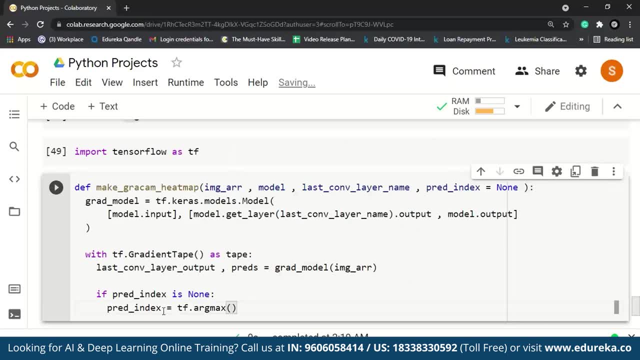 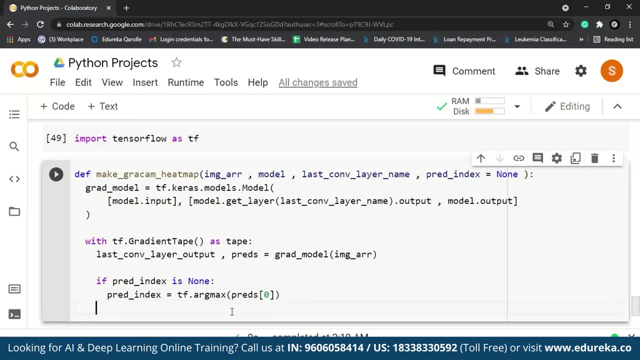 So it's totally up to you. And now this is whatever predictions we have. So Preds, that's present over here, And then all we're going to give the index 0. So if this is the case, and then what we'll do is we'll have class channels. 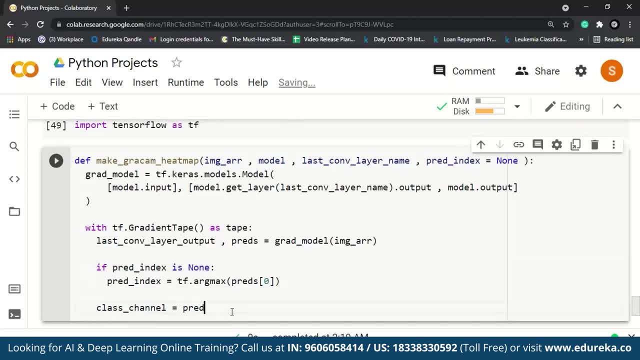 Are we going to add all the Preds value? So Preds, all these, and then we have play index. Let me paste it over here: Pred index. So this is a scenario here. So now what we'll do is we'll take off. 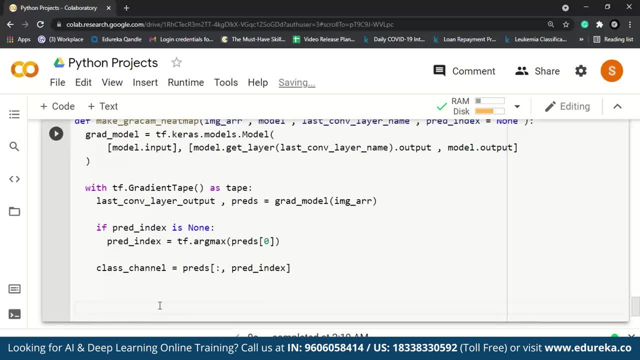 So now what we're going to do is, you know, from the feature map, we're going to pull in the gradients. So grads is equal to tape dot gradient. So here we're going to pass the class channel and then the last convolution layer. 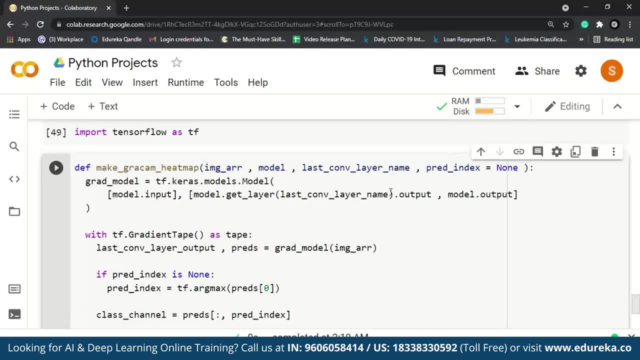 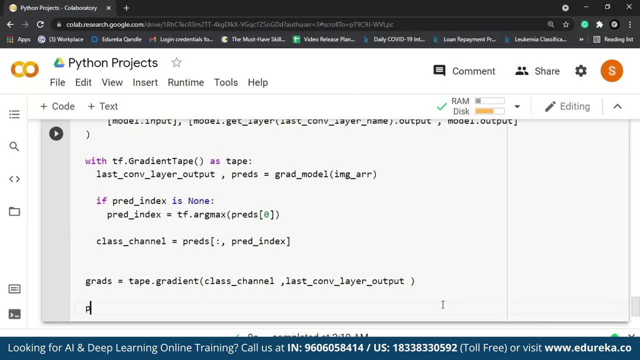 as you know, class channel is present here, and then we have the last convolution layer output, which we have captured it from here. So, finally, what we're going to do is we're going to get the mean of this. So we let's say pool. 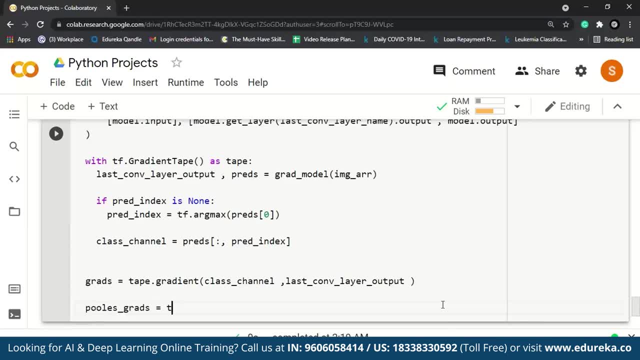 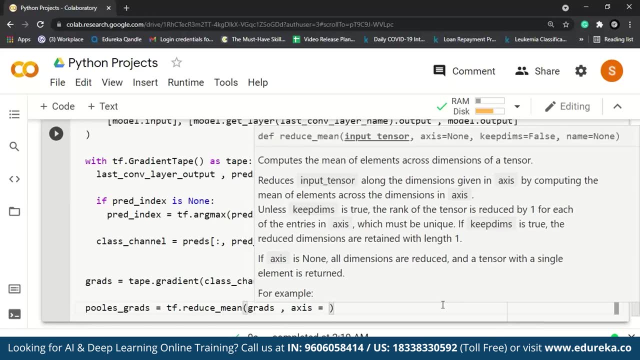 Let's give the name here as pooled gradients or grads. So we'll have TF, dot, reduce, mean now We'll just pass grads. Then we have axis is equal to 0 comma 1 comma 2.. That's because we have three channels. 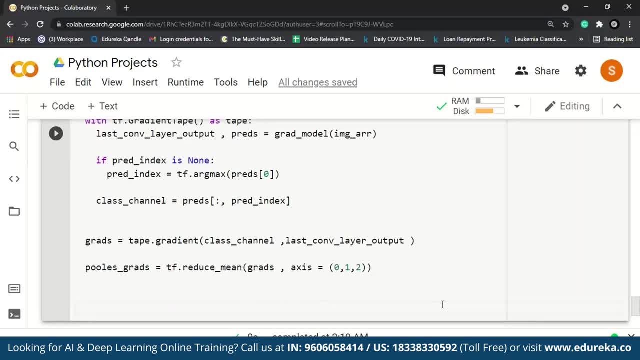 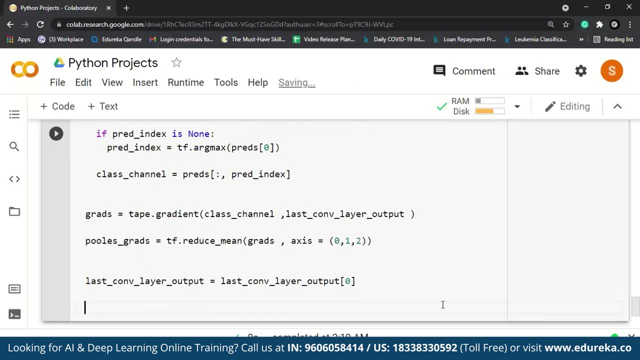 And finally, now we'll put this in the form of a heat map. So we'll have lost convolution layer output. This would be the same thing, but present at the index 0. And now we'll put this in a heat map. Let's give the name here as heat map. 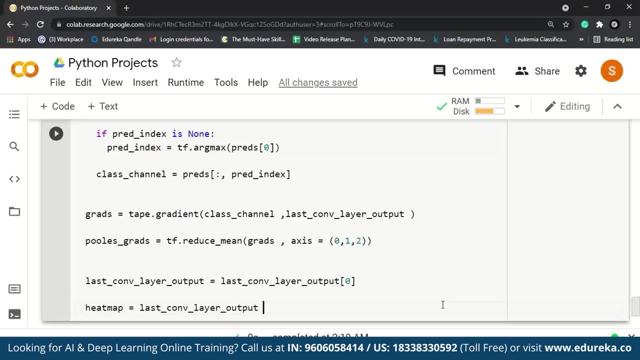 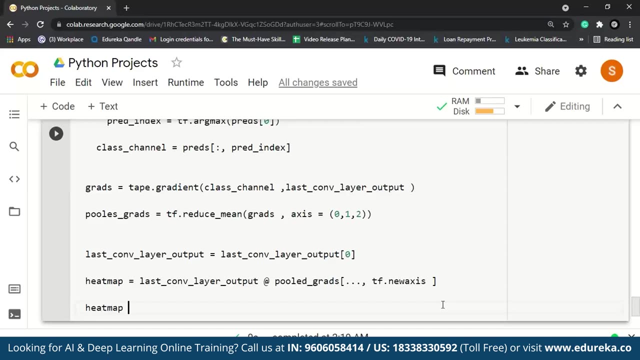 So this will be last convolution layer output, And then we'll give this at symbol pool grads And then finally we have TF dot new axis. So now we'll do it: TF dot squeeze, just to bring them in a shape. So heat map, this would be equal to TF dot squeeze. 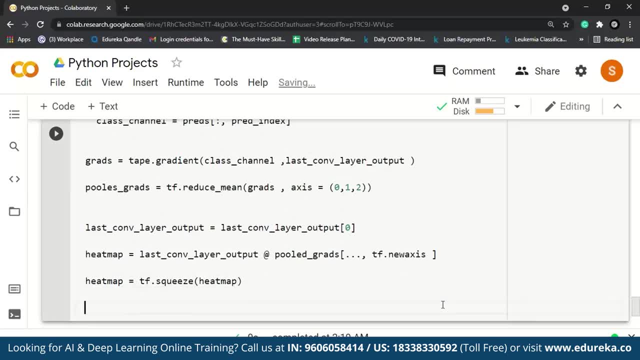 and then we are going to pass heat map here And finally, for the visualization purpose, We are going to see how this would work. So heat map, This is equal to TF dot, maximum heat map, comma 0. and then we have a F dot, math dot, reduce Max. 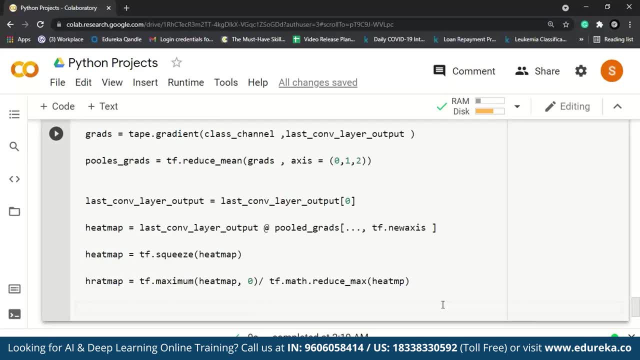 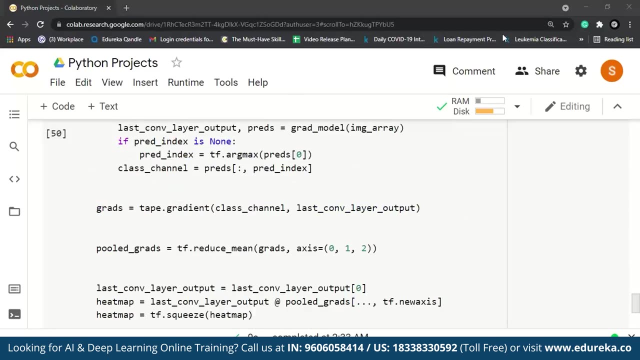 and here we're going to have heat map and this would basically written me: Heat map, numpy heat map, like basically the numpy array of that. so return: heat map, dot number. So let's now try executing this and we have successfully executed this function. I know it's pretty complicated and pretty huge function. 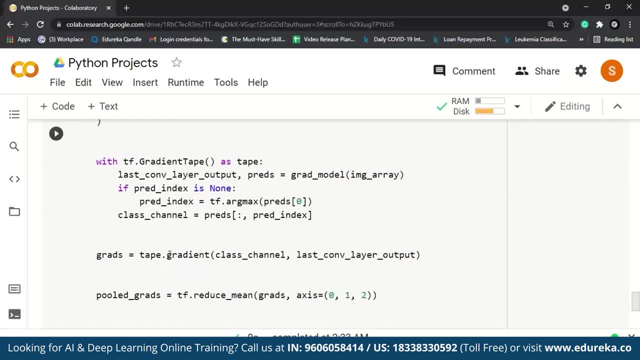 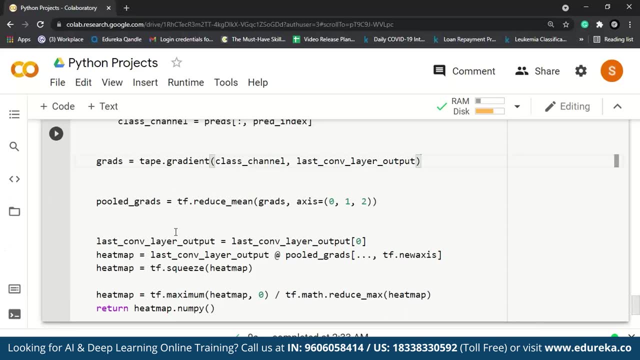 and you know in one go it's pretty hard to understand this. if you're having further queries, either you can mention them in the comment box below, and the other way you can do is you can just get down to the official documentation of tensorflow and check this out. 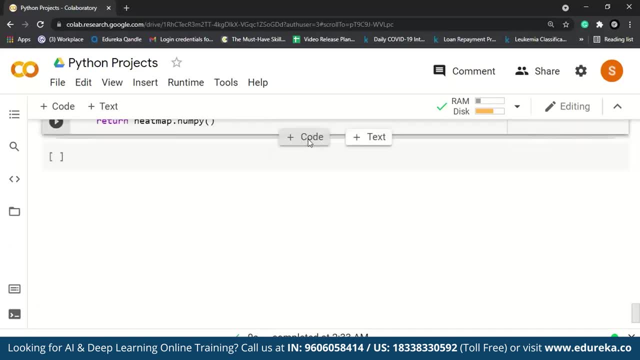 So now that we have done with this, now we'll mask the heat map on the image. So let me give a comment For this. we are going to import couple of libraries, that is, import matplotlib dot cm as cm, and then we also need to import I python display. 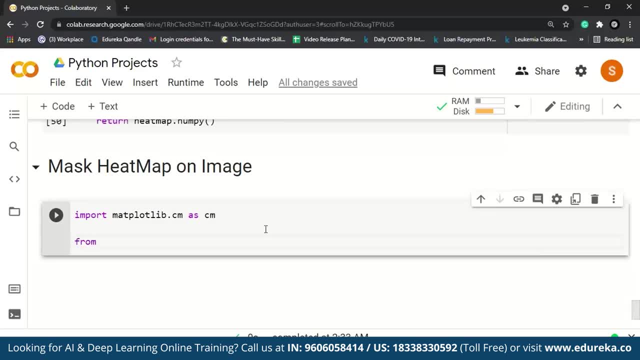 Although you can use PLT dot display or show, but let's try using different no library. here I python dot display, import image and then also the display. let's execute this up And now. what we're going to do? we are going to create a function. 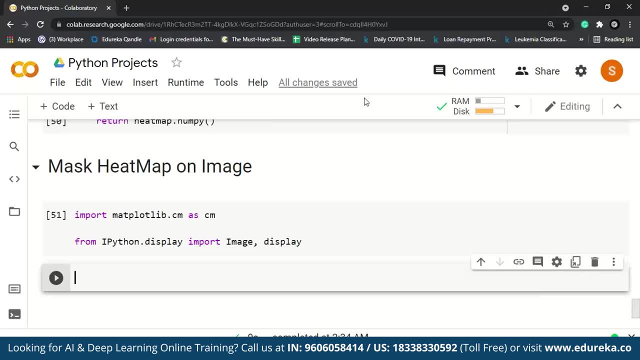 We're going to say save and display. That can be the name of function. This takes an image path. We'll also have the heat map which you have created. then place where we want to save our grad cam image and then the alpha value. 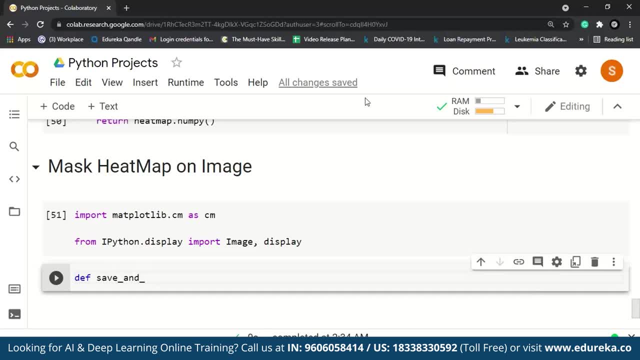 So they will have DF save and display grad cam. So we'll have to take image path and then we have heat map, then we have camp path. So if you can just give any name, will give it a scam dot, JPG or you can give any name you want. 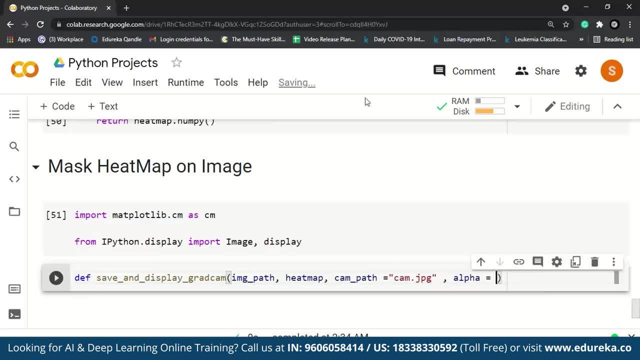 and then we'll also have the alpha value. I'll explain you. What does this alpha value, What do you mean? in a while, So, but as of now, just keep this in mind. So we have the alpha values, So the input image, whatever you pass over here. 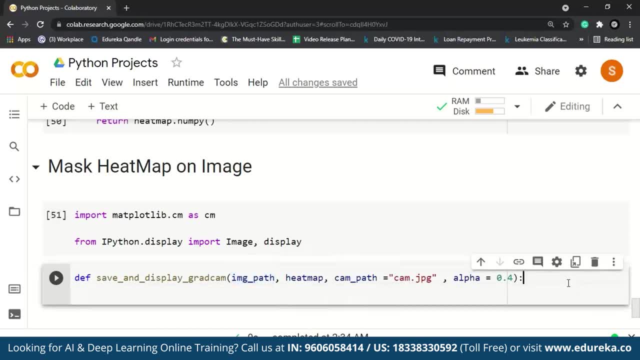 make sure it's not expanded and should not have a bath size. So that's what it means. So what we're going to do: we have image, So we'll have image, will have this as load image and we'll have image path, and now we'll try to convert this into an array. 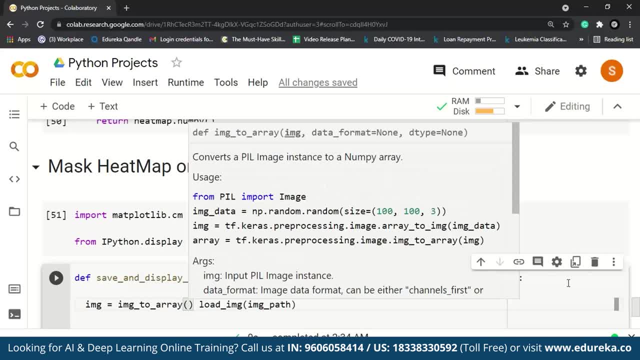 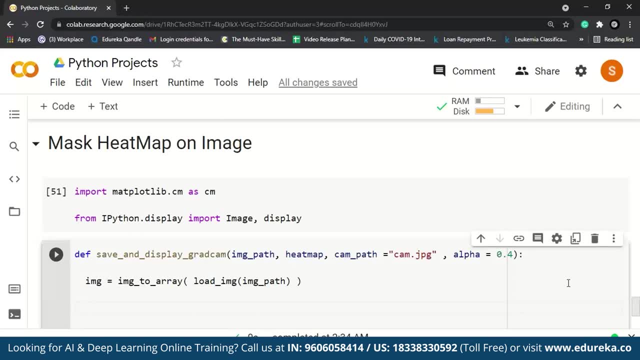 instead of writing this again, What I'll do is image to array and we'll pass this over here itself. This looks great. And now what we'll do is we'll rescale the heat map to the range 0 to 255.. So we have heat map. 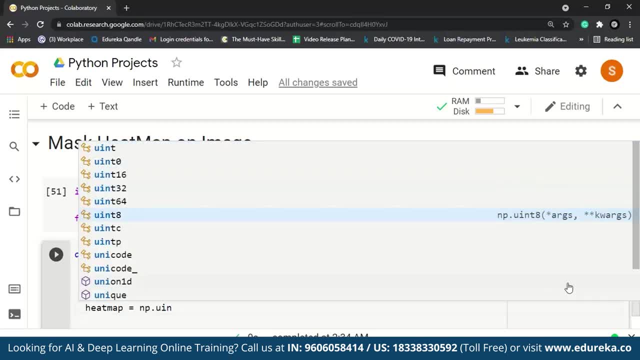 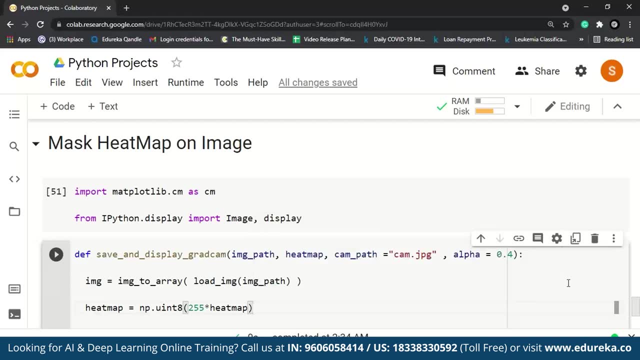 So we'll have NP dot units. Are we going to pass a? and we have 255 times heat map? This is probably up to you. either you can do this or you can divide this by 255.. It's totally up to you. So now we'll try to color map this. 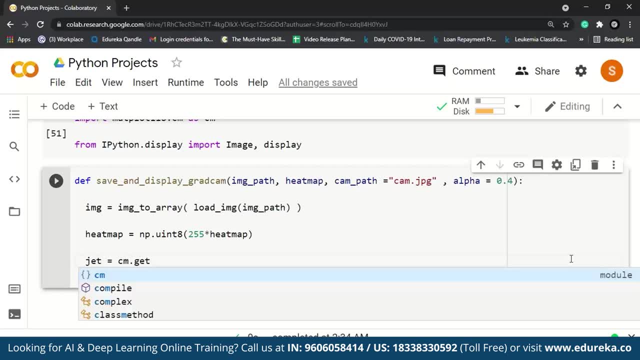 Let's say jet is equal to CM dot, get C map or color map. So here you can give either a, whatever value you want, but I'm going to use a jet. and finally, we are going to use RGB values of the color map. So let me give you, so we have, jet colors. 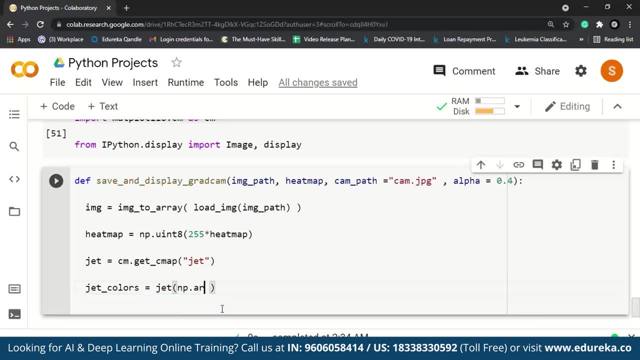 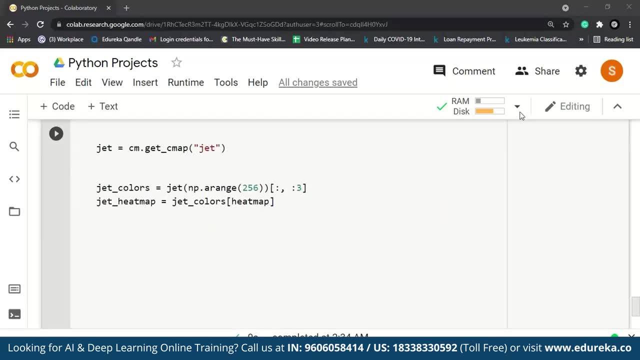 So we have jet NP, dot a range- We're going to pass 256- and finally jet heat map. So now, what we're going to do now is we are going to create an image with RGB colorize heat map. So let's do that. 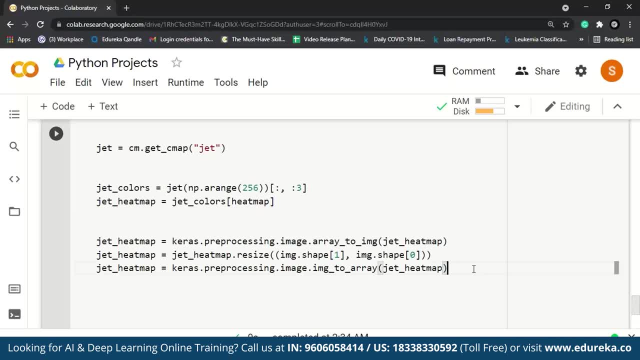 So, as you can see, we have done this over here now and in the next stage, what we're going to do, We are going to reimburse or we're going to superimpose heat map to our original image. So heat map basically has the gradients. 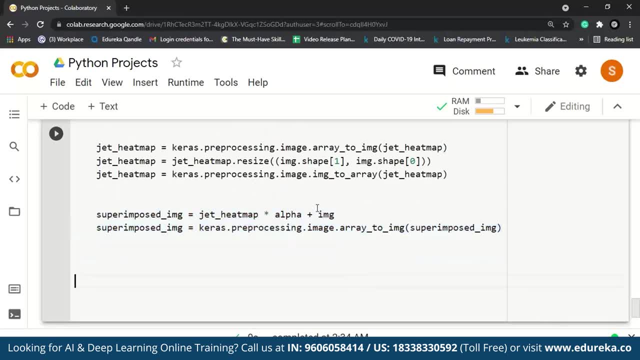 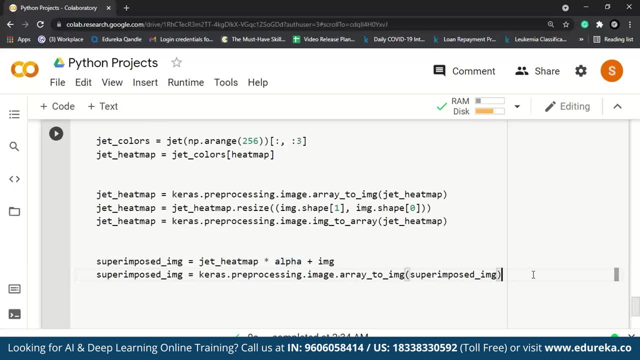 This is what happens over here. superimposed image, that is, heat map times. alpha plus image. This is why we are using the alpha value. So this is what is happening here and finally coming down to, you know, saving our model or saving a superimposed image. 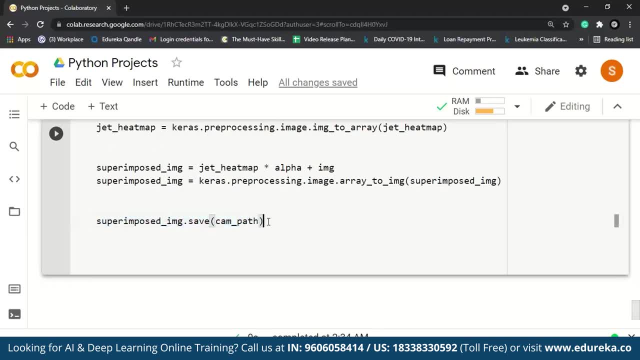 this function here: superimposed image, dot save and whatever the path you have given, that's a path where it's going to get saved and finally we are going to return the image right. So we're going to plot the cam image or whatever you call that up. 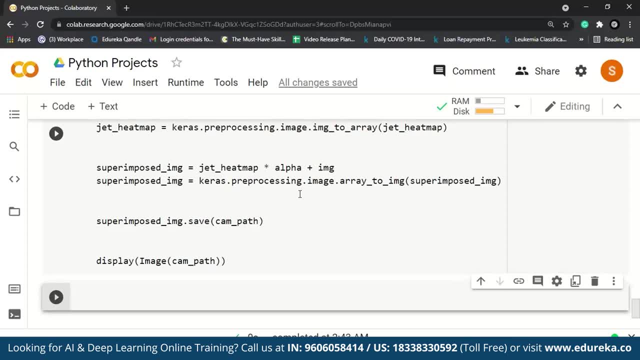 So this is all there is about building this function, And now, finally, what we're going to do is we are going to create a function which would make our life easier. So I've already written this function on top is kind of similar to what we have done earlier. 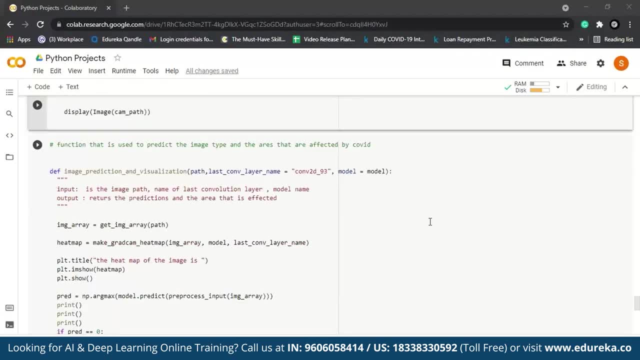 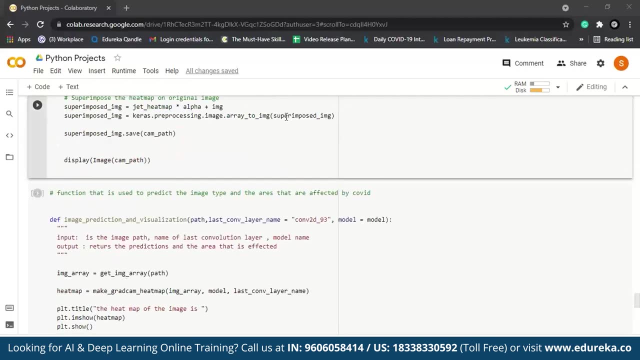 So let me quickly get that function up. So before that, let me zoom out for our simplicity sake. I have already returned the function here. So basically, what we're going to do here is provide the path We are going to give a function call. 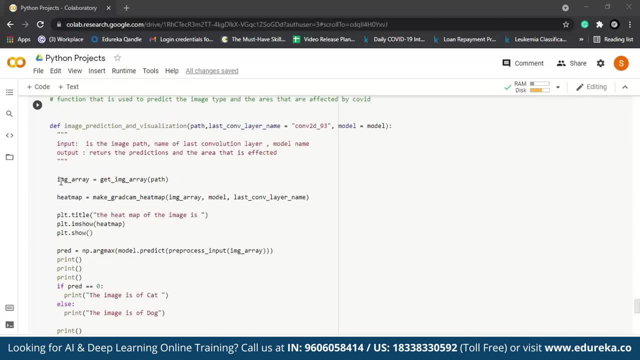 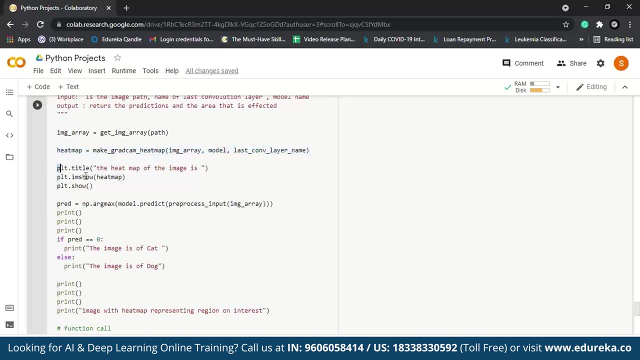 for a previous function that we had written, and what this function does is, first off, it converts the image, whatever we have, to an array, and within we call this function make grad cam heatmap. So this is done and finally, we are going to show the heatmap, what is generated, and then we are going to see: 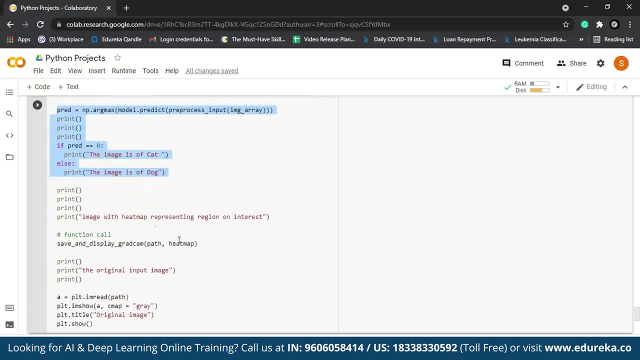 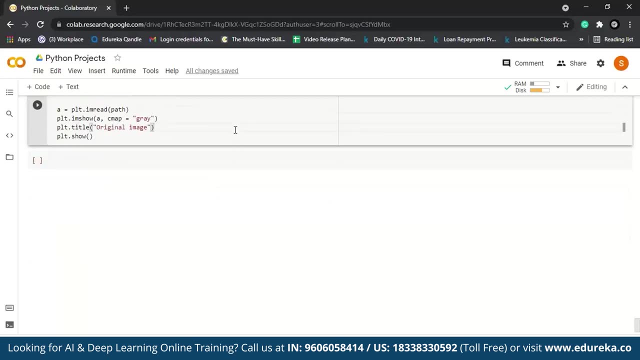 whatever the predictions have been done, And finally we are going to see whether it's of a cat or a dog, and finally, we are going to display our spot image on the heatmap and let's see how this would look like. So I have executed this, and now all we need to do 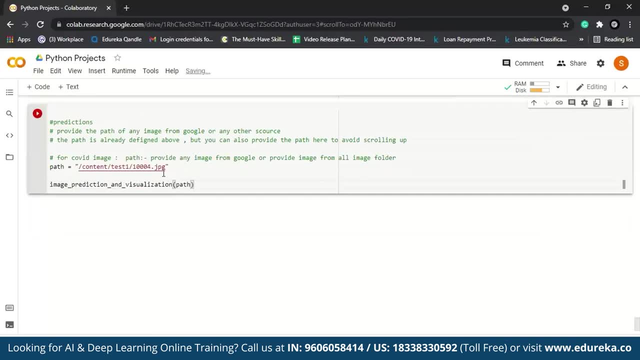 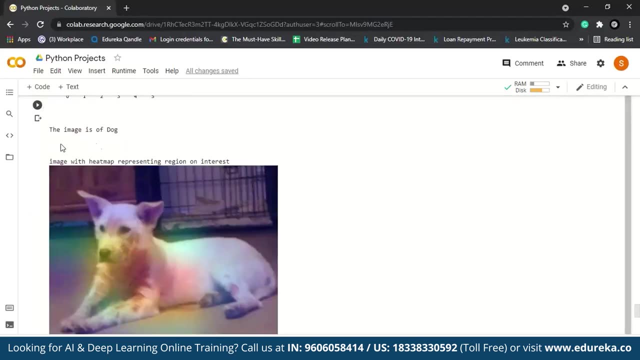 is: give a function call to this. So let's give a function call. This is a random image that I've chosen And let's add it over here. So, as you can see, this is the image of a dog, So a model has predicted the images of a dog. 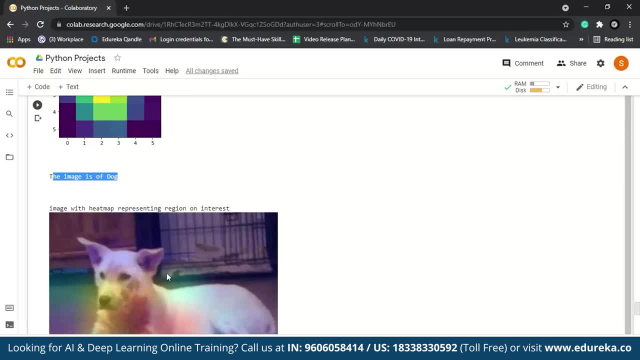 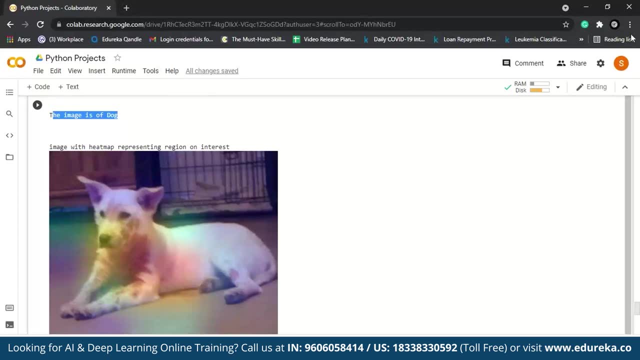 This is how a heatmap would look like, and when I try to map this heatmap to this image, you can see this particular model took this nose as an important function. So what we'll do is: let's go to Google now and let's take any random image. 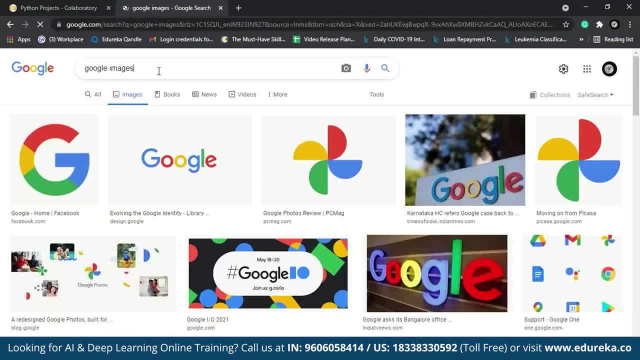 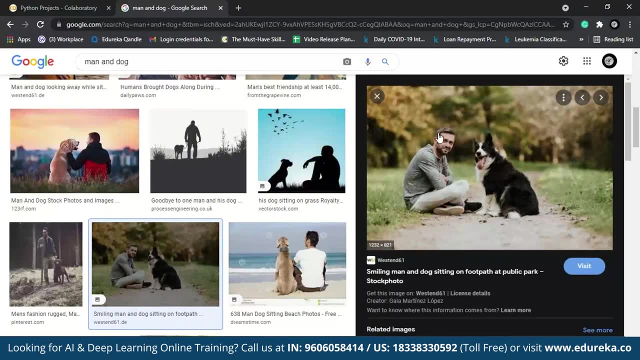 Let's say there is a dog and a human, so man and dog. So let's take any image. I think this is a good image over here. So what should happen now Is the heatmap should be formed on the dog. So let me save this image and upload it over here. 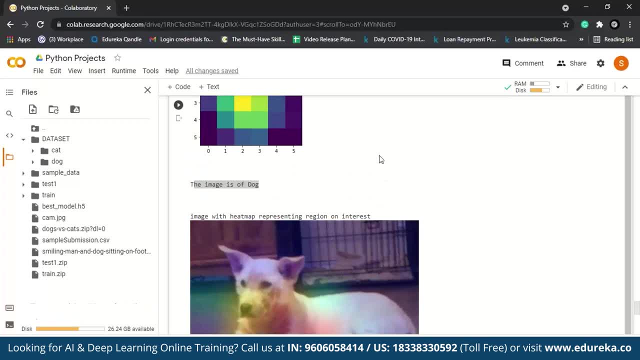 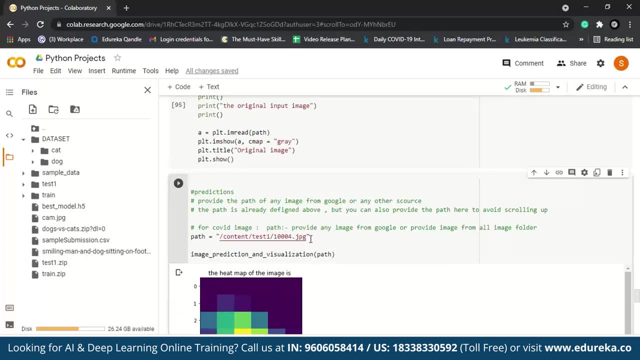 So let's try to upload this, and now all you're going to do is pause that image. So we have this one smiling man and her dog will copy the path and pass it over here And let's see how this would look like. Let me execute this. 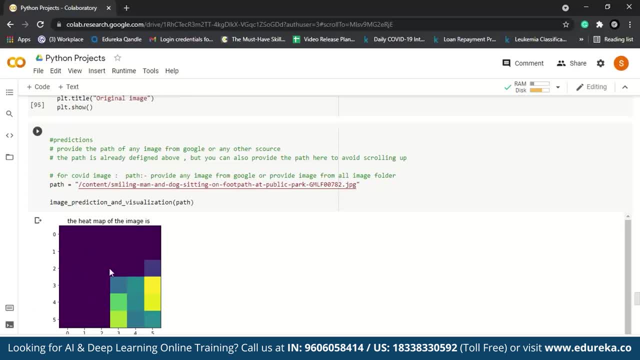 So, as you can see first off over here, according to the heatmap, this purple color over here represent that we don't have any feature, and this is where you know we have multiple features. anything closer to red, It means that that's the place that it's referring to. 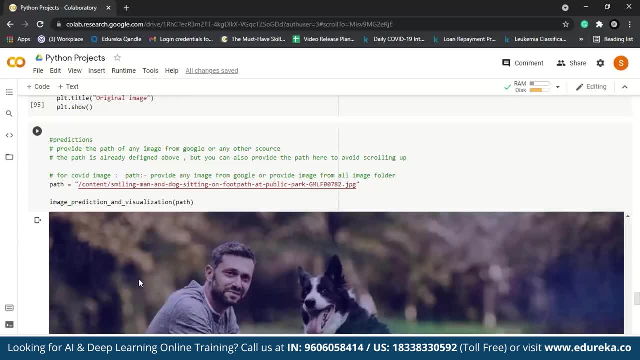 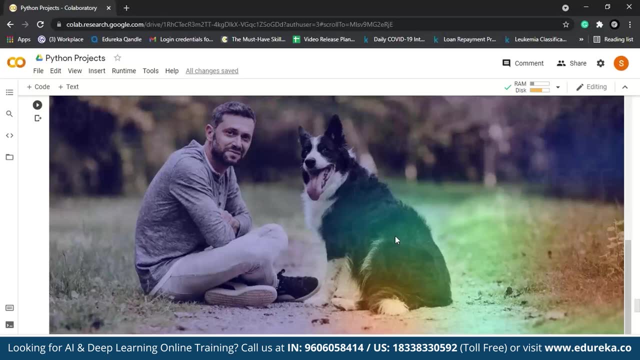 So here we know, we have a picture of a human being. So, if I scroll down now, as you can see, there is no heatmap which is generated over here, but the model has taken into consideration of, you know, the dog's tail and the fur and all of that. 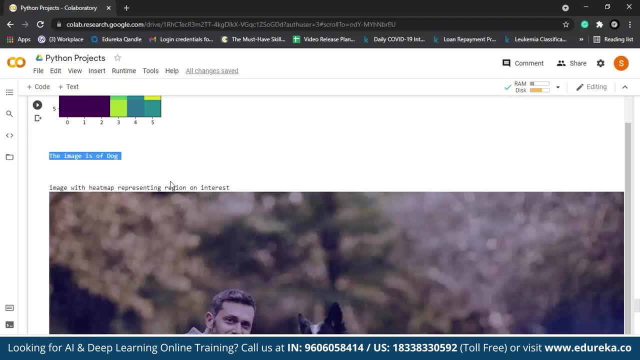 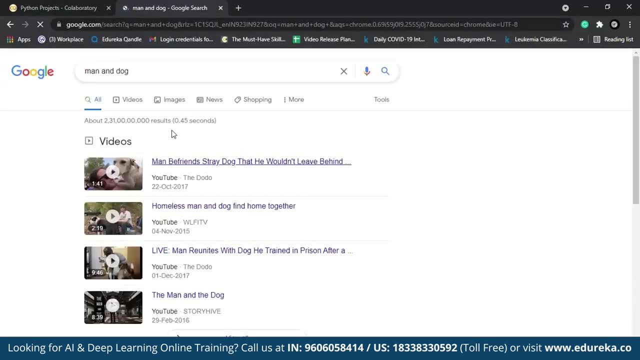 and let's see what it has predicted. It has predicted, right, the images of a dog, and if you want to see the original image, so this is the original image over here- Let's give it a try with other image here. Let's see how that would look like.